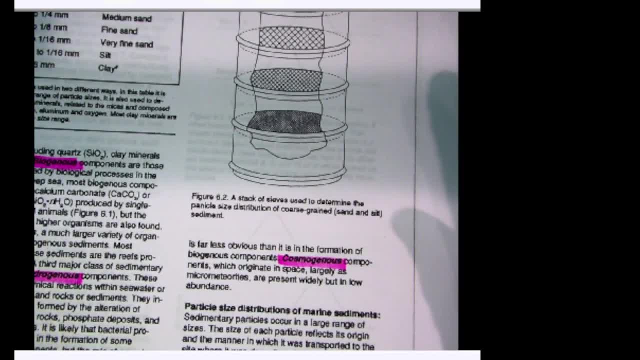 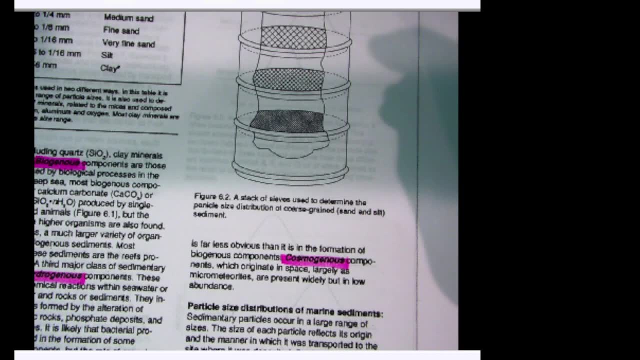 And then there are even cosmogenic sediments, right things like micromuniorites that fall into the ocean. So there's lots of different types of sediments based on where they come from, And then another way to describe sediments is to look at their particle sizes. 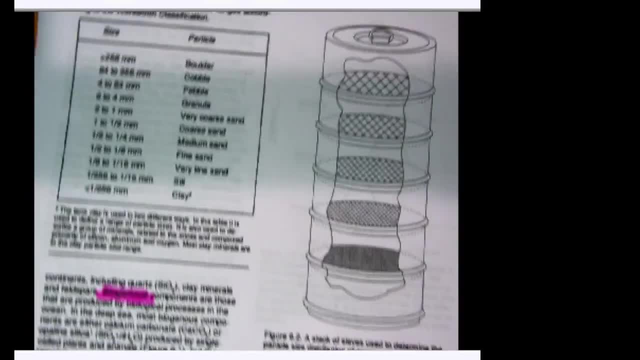 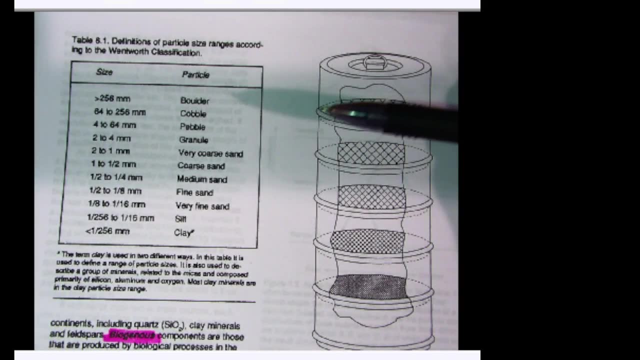 So this lab has a nice little figure here that shows the different particle size ranges. And so in geology we have these different terms for different sizes of grains. And so in geology we have different terms for different sizes of grains. So in geology a boulder is not just a large rock. 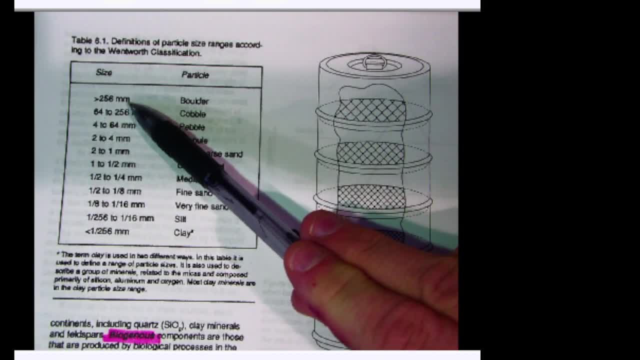 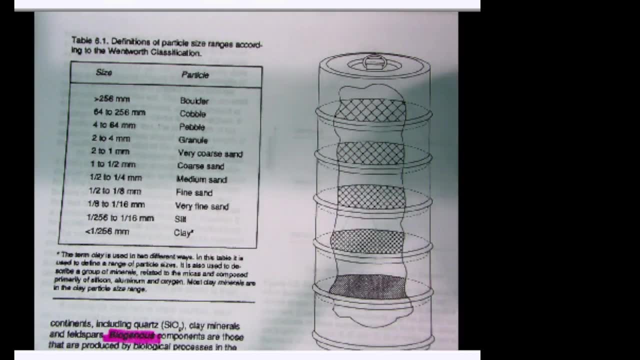 It's one that is more than 256 millimeters in its widest diameter, So some grains are perfectly spherical. Other ones are like oval shapes, so they have a longer and shorter axis, right, But that's this part of how we describe them. 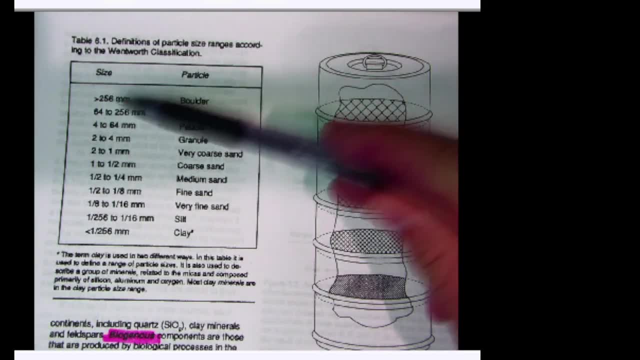 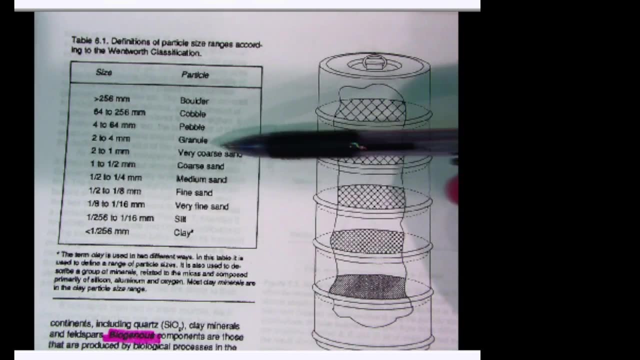 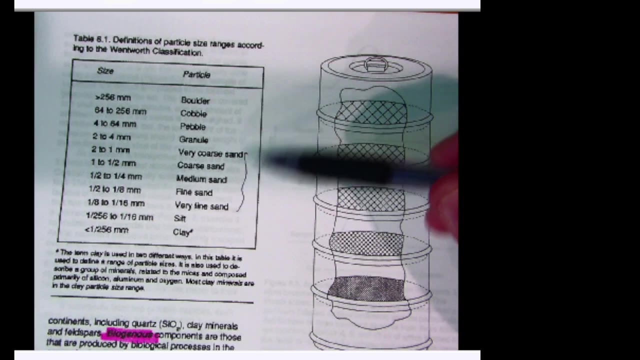 But if the longest axis is over 256 millimeters, it's a boulder. If it's between 64 and 256 millimeters, it's a cobble. And then we have pebbles, granules and all of these guys here. these are all different types of sand. so sand is a. 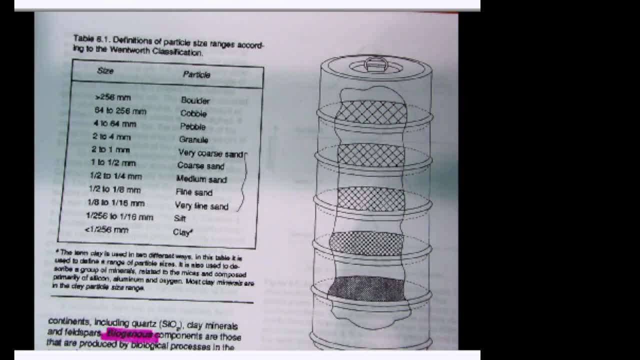 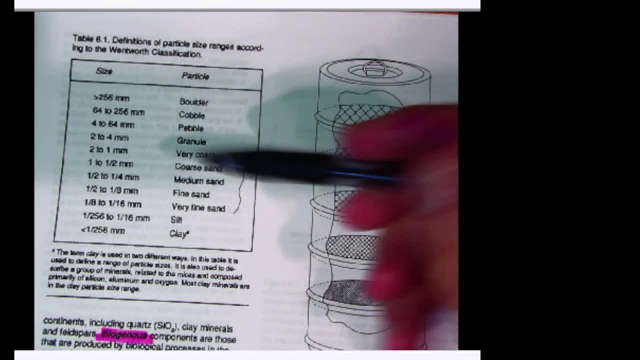 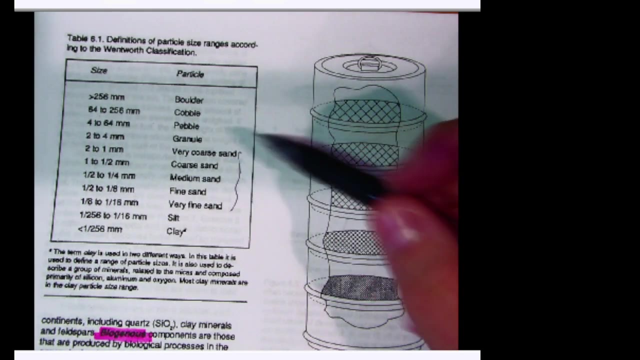 size class for geologists. not just, it's not a material, right like beach sand can be made up of a lot of different materials, but it's all sand because it has these size ranges. so sand is also. it's pretty important. it's well studied, so it's divided up into this very coarse, coarse, medium fine and very fine sand. 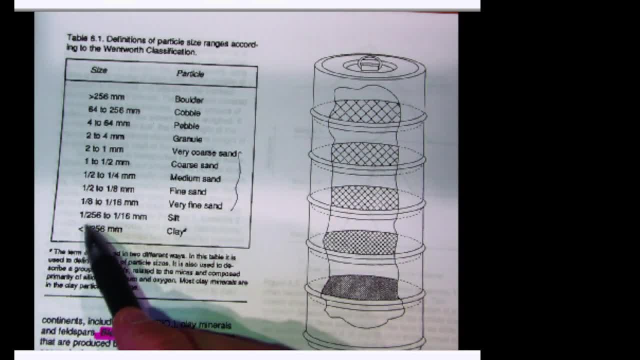 below sand sizes. so 1 256 to 1 16th of a millimeter. you have grains that are silt sized. so you take a millimeter, you break it up into 256 parts, right? one of those parts is the width of a grain of silt, and anything smaller than that is a. 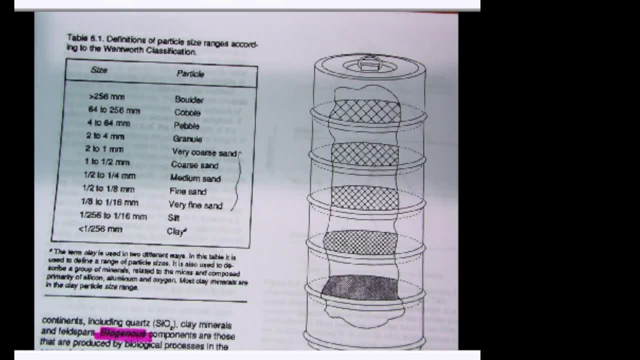 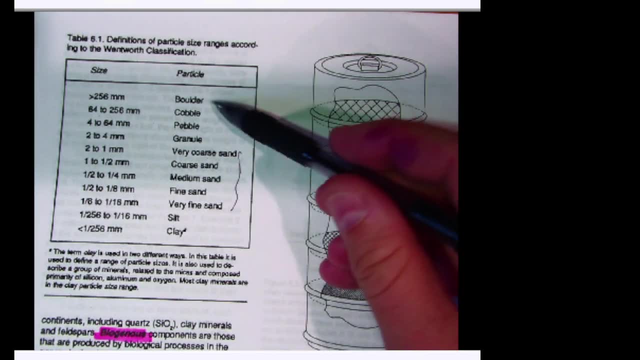 clay. right, the grains are clay, so clay can be a kind of mineral, but it's also a grain of clay. so clay can be a kind of mineral, but it's also a grain of, so a size of a grain. so you can have a boulder made out of quartz and it would. 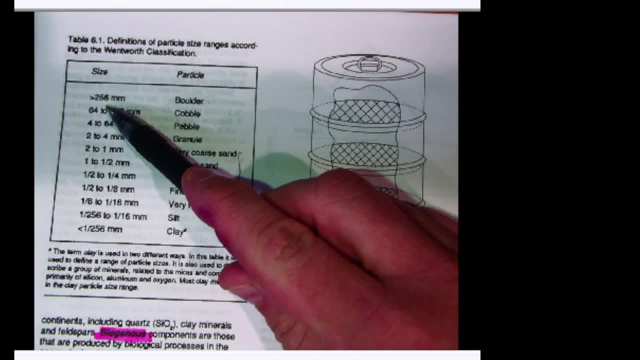 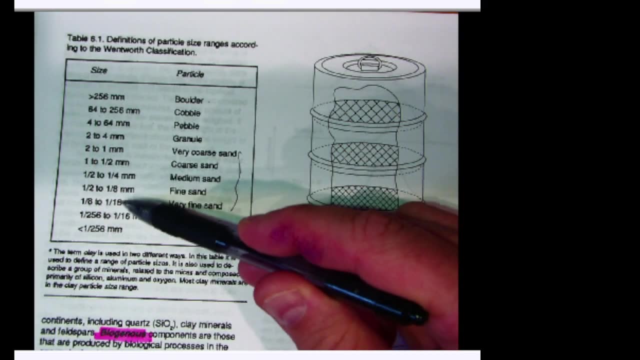 it would be a quartz boulder. if it's 256 millimeters in size, you can have grains of sand that are made up of quartz and they'll have those size ranges. you could even, in theory, have pieces of silt and clay that are also made out of quartz, or 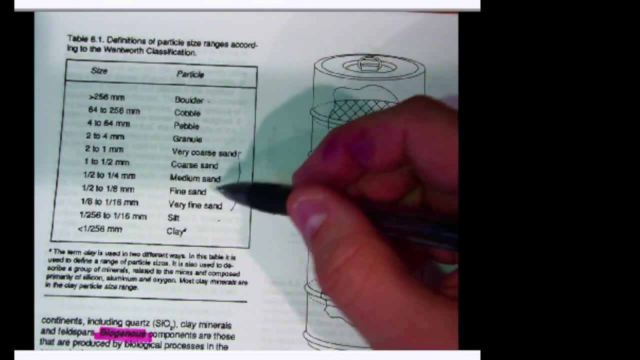 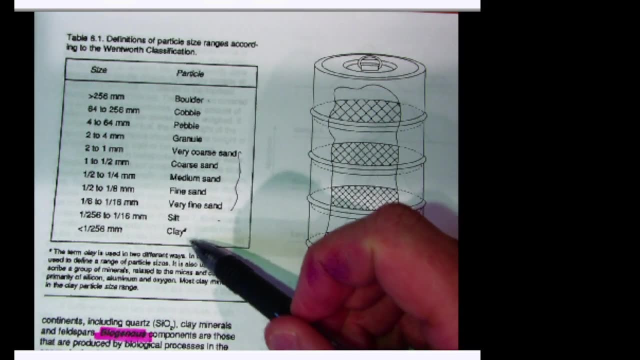 you can have it made out of feldspar boulder or feldspar sands or feldspar clays. you can also have the different clay minerals, which are a special group of minerals that are also clay and silt sized. so the sizes are really important for us, right, there's. 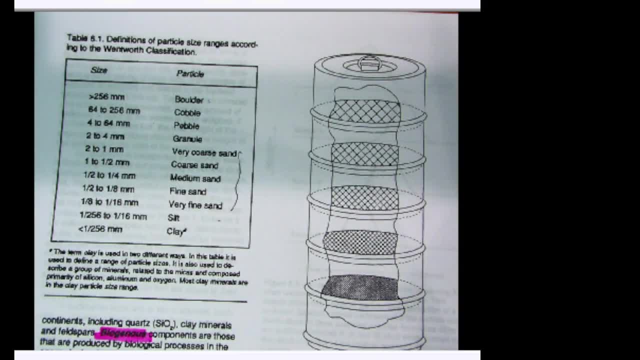 there's lots of ways to think about these sediments. it's, there's the minerals, the chemicals they're made up of. there's the way in which they were deposited or brought to a location right. was it from an organism? was it from land? was it from from a meteorite? 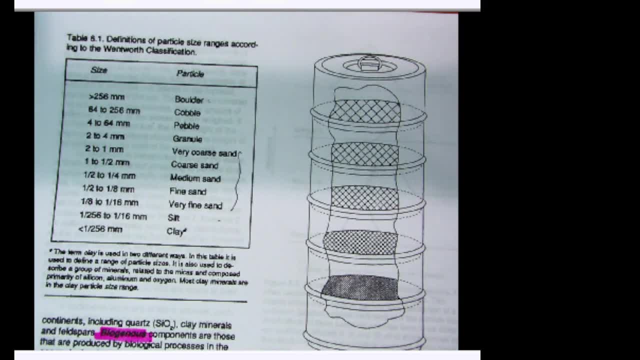 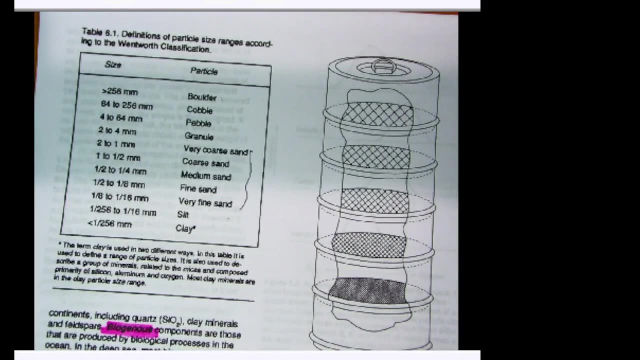 then there are the size ranges of the grains. so those are all important parts of understanding an ocean sediment. so you might go to the beach and dig up a pile of sediment or sand or you know, just sediments on the beach or in the water, and if you want to know about its size distribution, 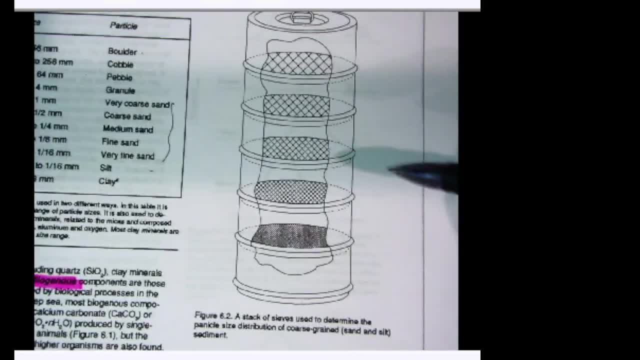 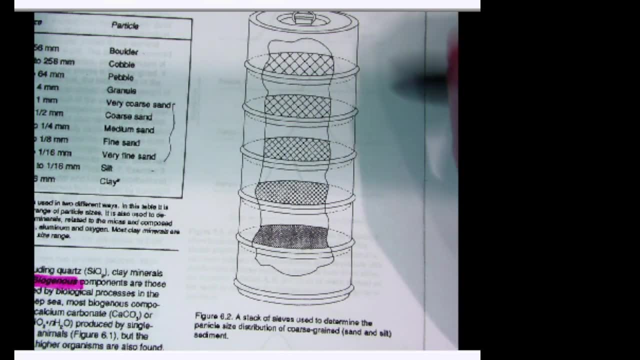 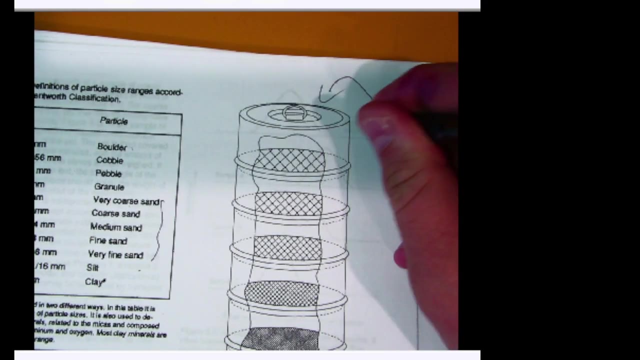 right, you can run it through some sieves. so this picture here shows a stack of sieves. they're basically little screens, and you would take your big mixed sample of sand right and you would pour it into the sieve, and so you'd have big grains and medium-sized grains and small grains. the big grains: 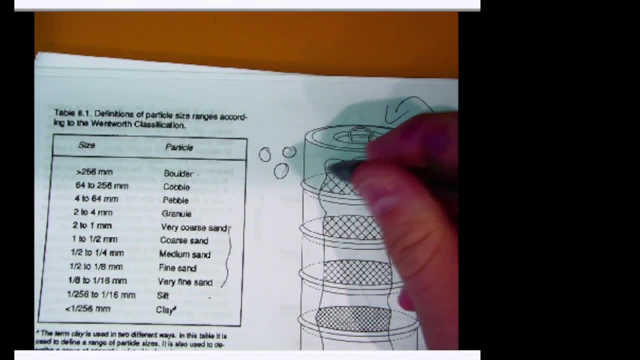 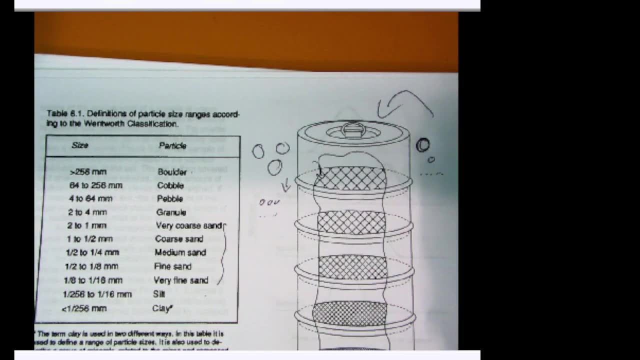 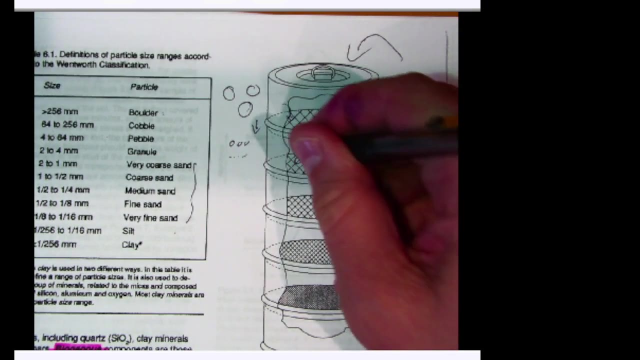 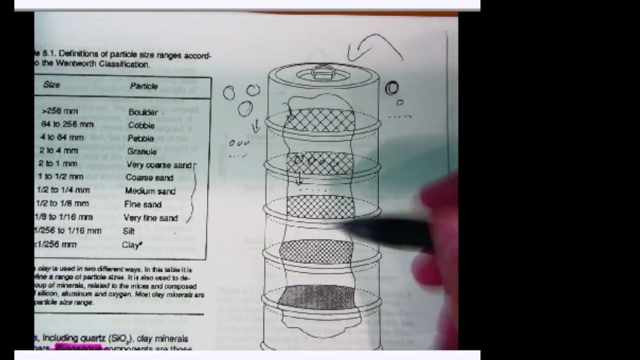 will get stuck on here and they can't pass through these little openings. but the smaller grains they can go through, so they'll fall onto this sieve. they'll get. some of them will get stuck here, right, okay. and then the really small ones will also pass through, and that goes on and on and on, with smaller and smaller. 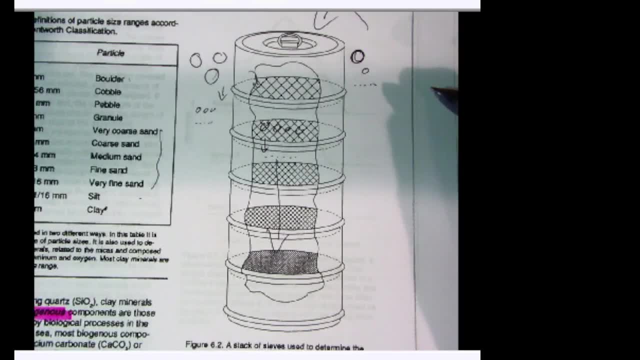 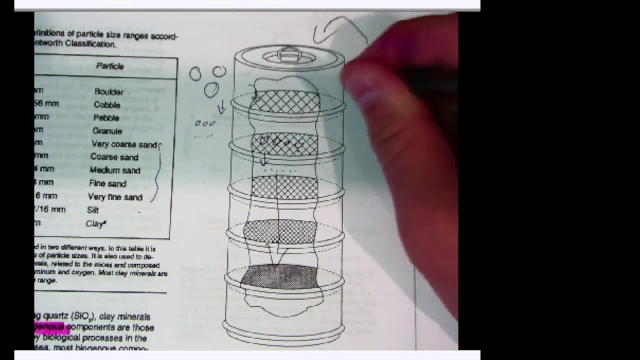 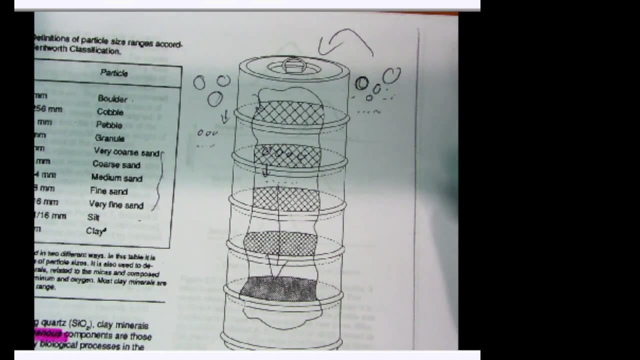 sieve sizes. um, and so you've. you've broken it up into all the different components of it, so you might again. you'll start off with a big random sample of sediments and we'd like to know what are the ranges of sizes here so we can run it through a sieve. 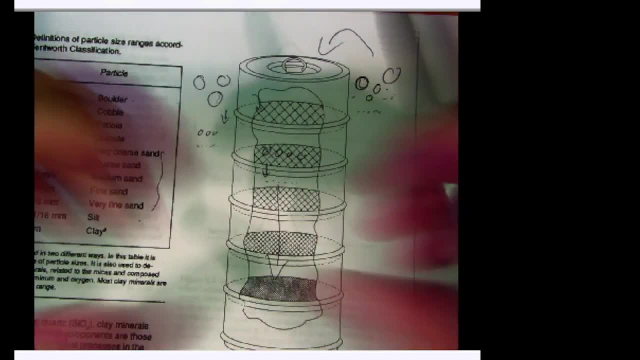 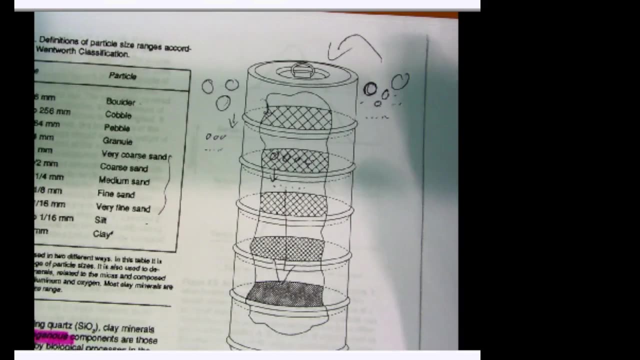 stack and these sins they can be. they can be small or they can be really big, like, like the size of a record. they can be eight inches across and we'd have stacks of sieves one on top of the other, so they're open at the bottom and at the top also. 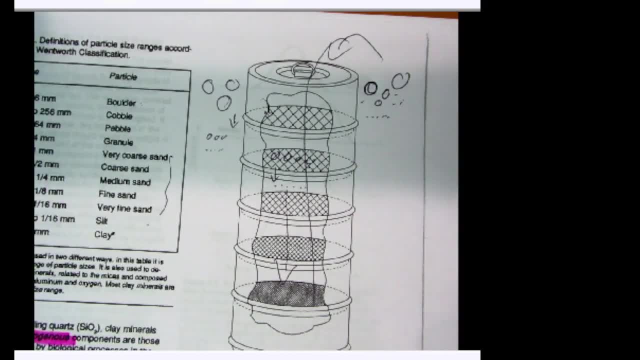 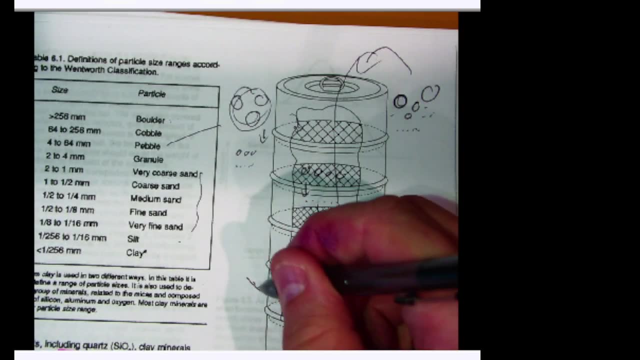 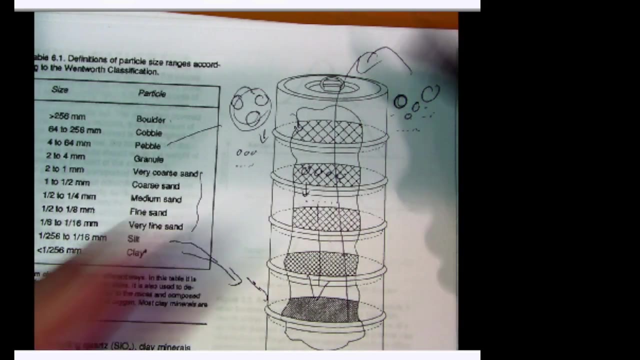 and the sediments go through here and they turn into these different size classes. so on this top piece you might have pebbles, and then, by the time you get down to here, you might have silts and clays. okay, so that's nice, you can break it up into the different. 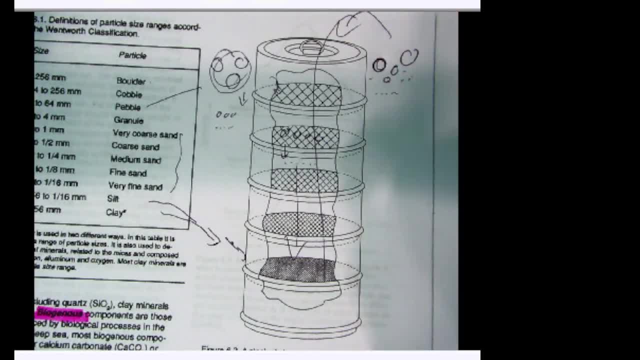 components we want, and then you could say, oh, there's very little cobbles, or it's mostly clay sized, or everything is sand sized here, or it's a mixture of sand and very little fine particles. right, but if you want to put numbers on that, then you can calculate the percentages. so you might start up with a. 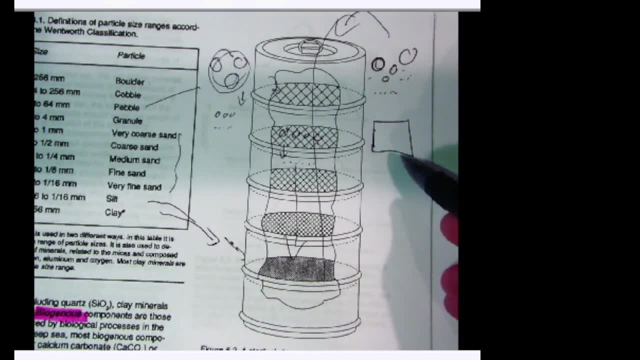 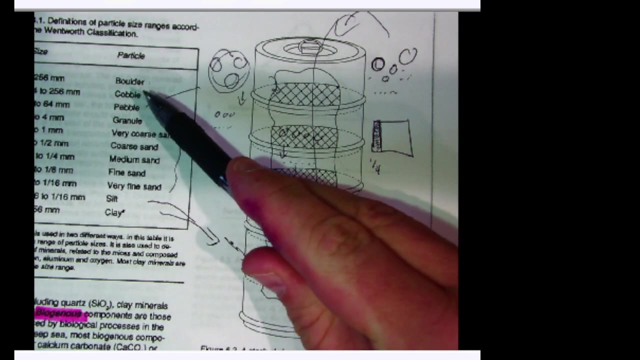 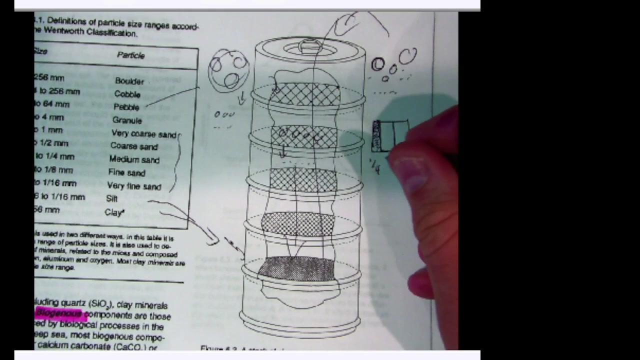 whole sample of sand of all different sizes and you might find out that a quarter of it, that's a metroid, but a quarter of it might be cobble sized, and then maybe- I don't know- maybe 30 percent is sand sized and and so on, and so you might have a very small percent, that is. 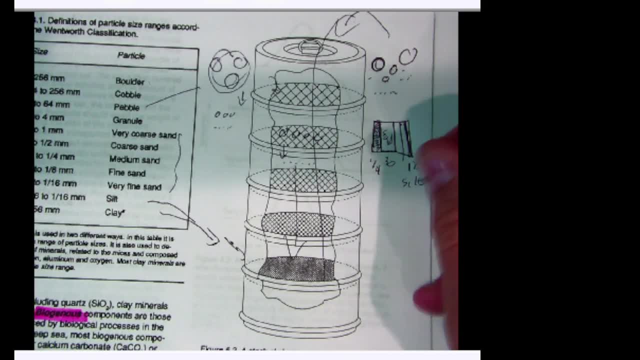 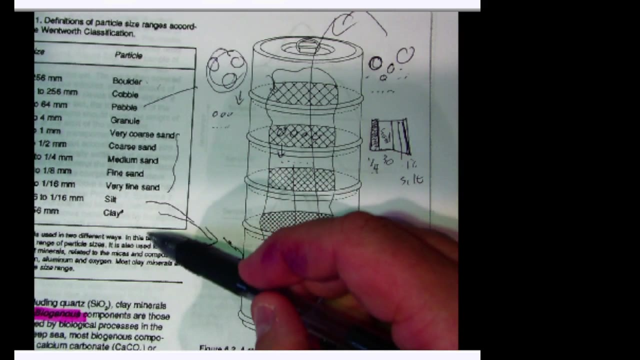 like one percent. maybe it is silt sized, okay, so just just conceptually, you can have this whole sample of sand, of sediments, and then you can start telling us what percentage of the whole each each sediment size is. so, conceptually, that's how you would do it. how would you do it in actuality, right? 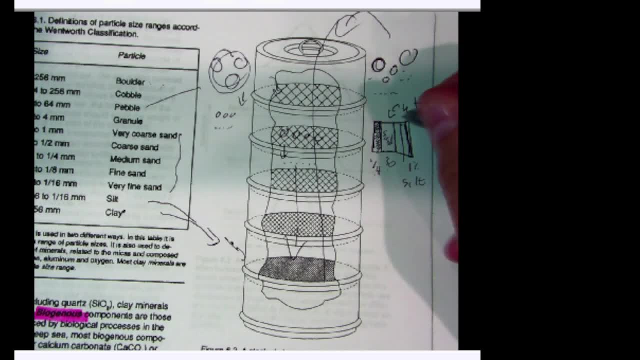 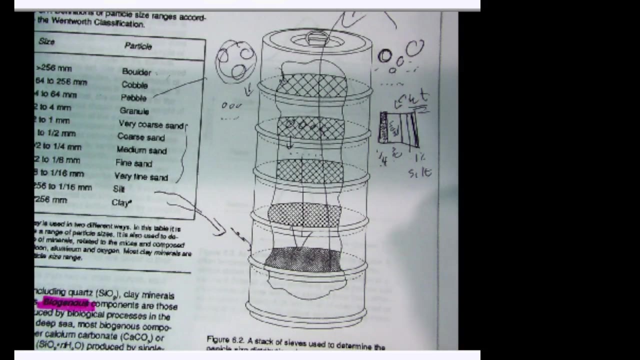 well, you would weigh this sample, you get its weight right, and if and if it weighed a hundred grams and then 50 grams was sand, that would mean that it's 50% sand, right? so just as an overview, that's how you do that kind of thing and that's. 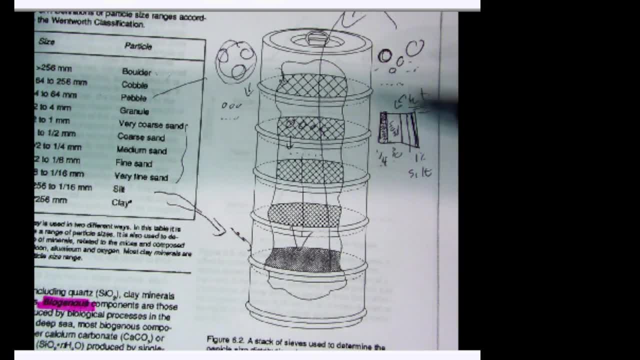 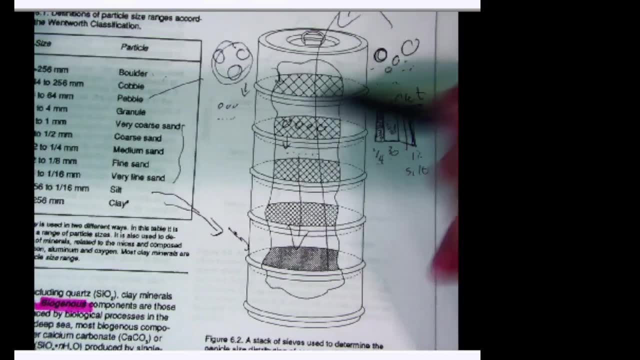 that's what we do it in this lab. so in an in-person lab we would actually have these stacks. we'd weigh the sand, we'd run it through this, we'd get each so in. then we'd get each component. we'd weigh how much was stuck on here. we'd weigh. 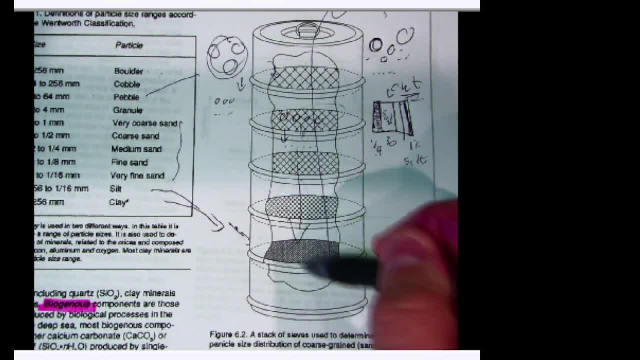 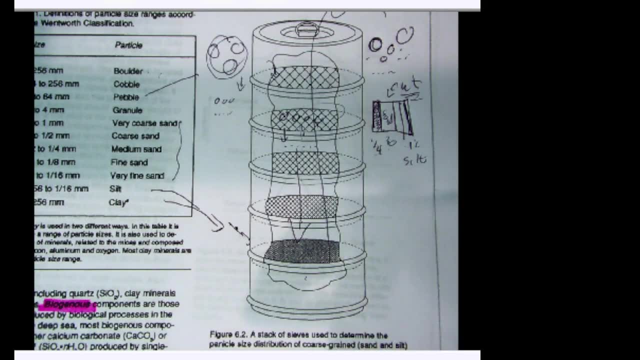 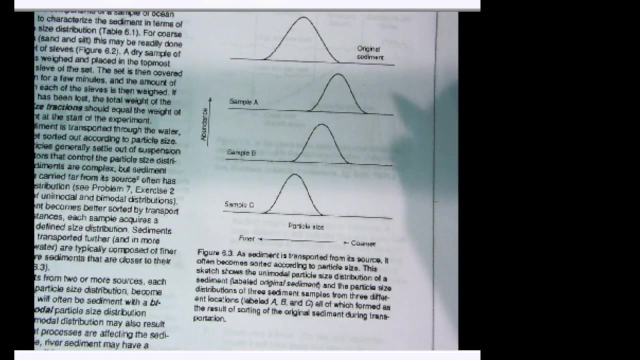 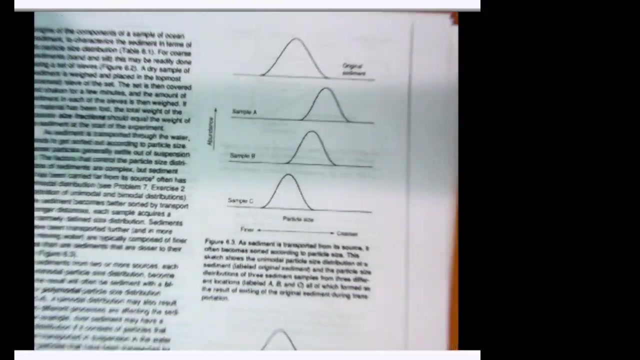 how much didn't fall through this screen. then we'd weigh each one of these and some would be zero, other ones would be a lot of weights, right, and that would allow us to calculate the percentage of each size class. now, once you know, this might be a little hard to read. once you know the size distribution, 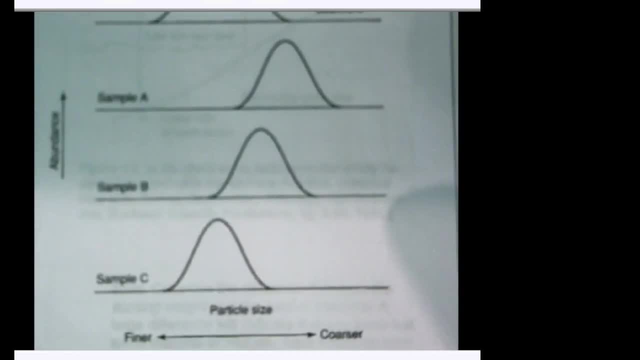 right, then you can do some more with it. so here's a just like a theoretical and conceptual chart. right, it has the size of particles along here. from very fine particles it's very coarse particles, so maybe boulders, gravel, sand and then silts and clays, and in this particular sample we might have found that there. 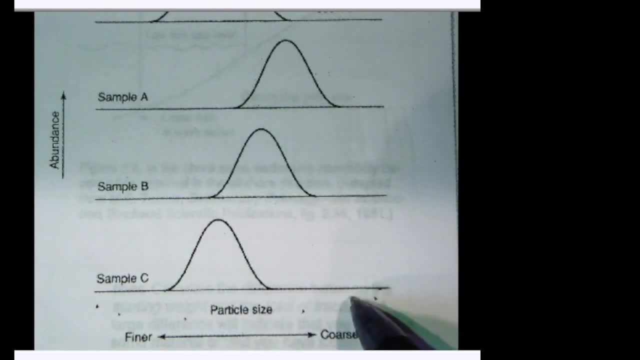 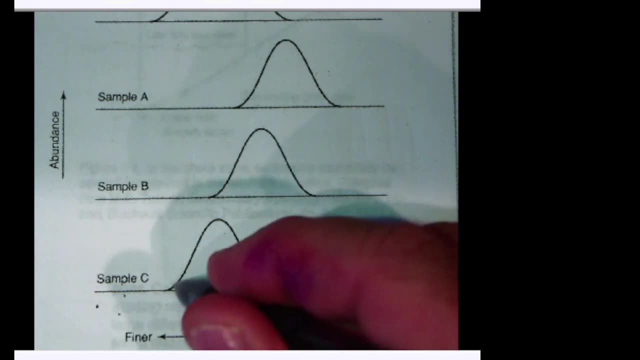 was a lot of sand size particles and very little boulders and very little clays. and so now what you can do is this chart shows us the abundance of those different sand sizes, of- sorry, of those different grain sizes. so the higher the peak, the more of that particular size. 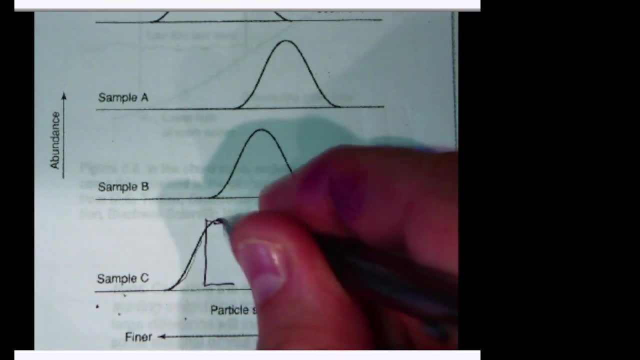 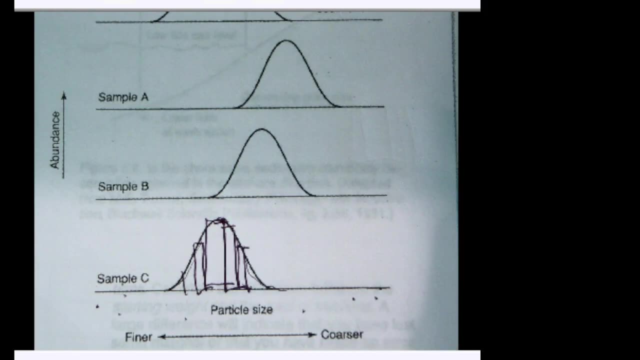 there was, so you can kind of think of it as a stack of these rectangles right instead of a nice curve right, and so this might be 50%, and this might be 40%, and that could be another 10%, right? so each one of these? 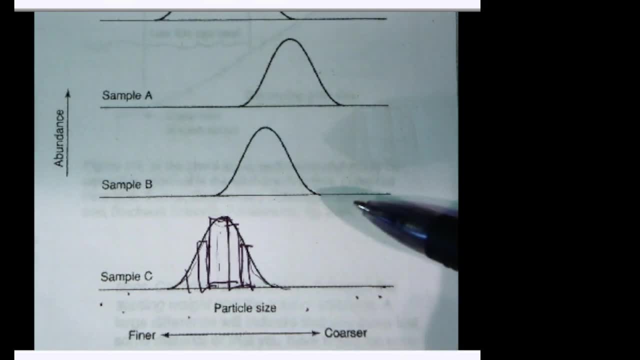 could be that, so you can take that information you got before, where you weighed them and found out their percentages, and then you can just make a little, a little bar graph right showing how much of each, what percentage, each size class was, and it would eventually look like this curve. so 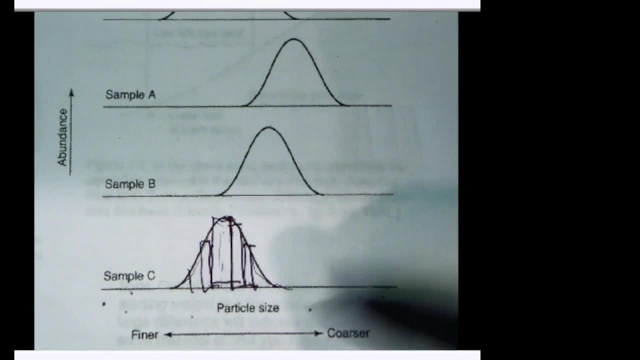 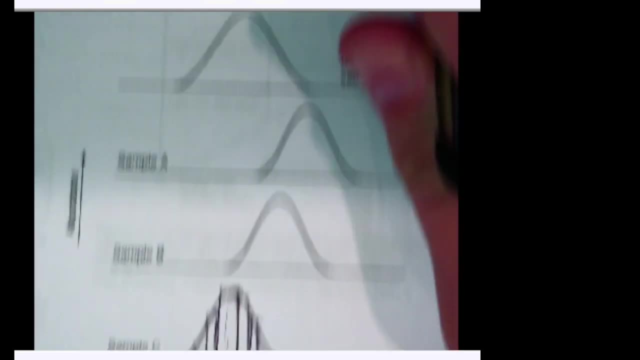 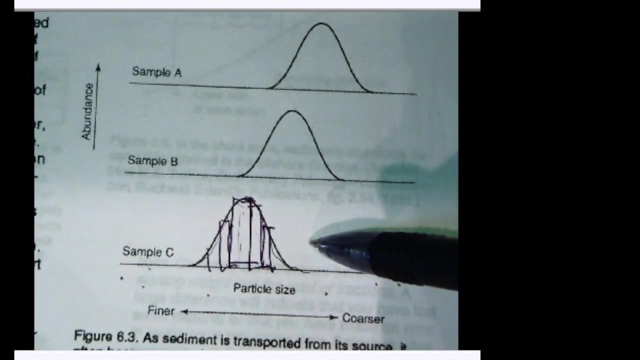 the curve is really smooth, smoothed out version of that. so one sample of sand might look like this, one sample of sediment might look like this, another sample might look like that right, and another one might look like like this. so this could be a beach in, you know, Brooklyn. this could be a beach out on. 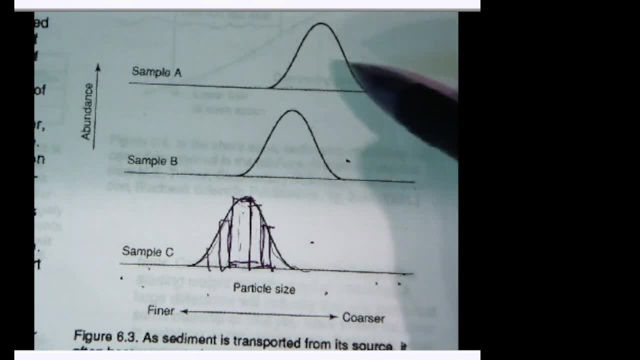 Long Island. this could be a beach from New Jersey, right. they might all have different distributions of their grains. this could also be so. this lab talks about it. this could also be different zones along the beach. this could be the dry part of the beach, right. this could be the part that is in the area that is. 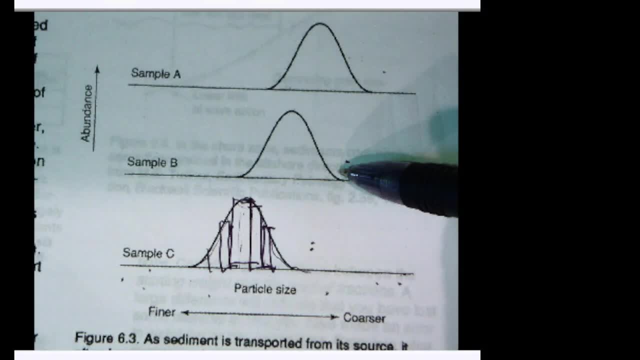 hit by waves. the weather waves go back and forth and this could be a sample taken from a part of the beach that is always underwater, right, so you can go in increasingly offshore, right, so you might see different patterns based on where you are along the beach. and I'll just move down to this one. I just described a really simple situation. whoiamou have one peak. most of the grains are centered around that one peak. 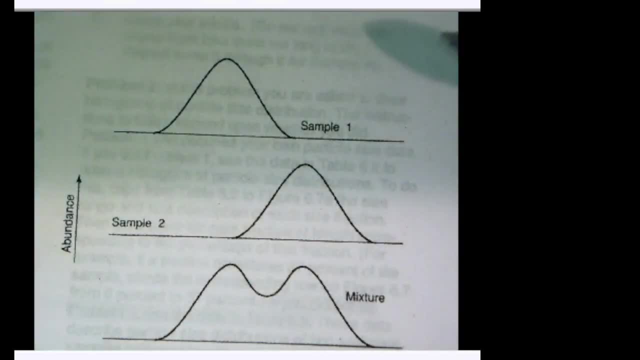 so we had- I just described- a really simple situation where you have like one peak. most of the grains are centered around that one peak here and I'm gonna just this size range. here's another sample where they're also have they have one peak. they're mostly centered around one size range, even though it's a different. 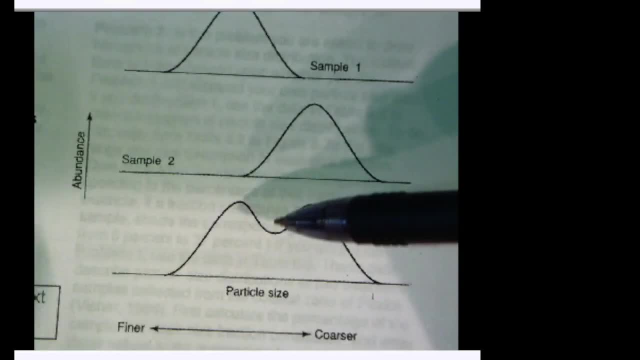 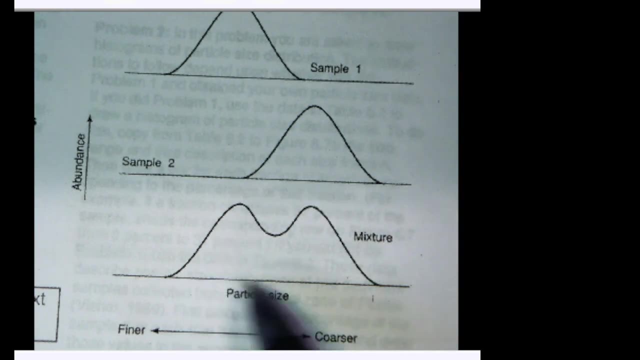 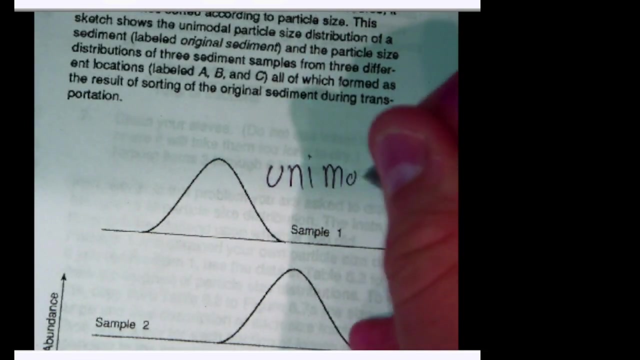 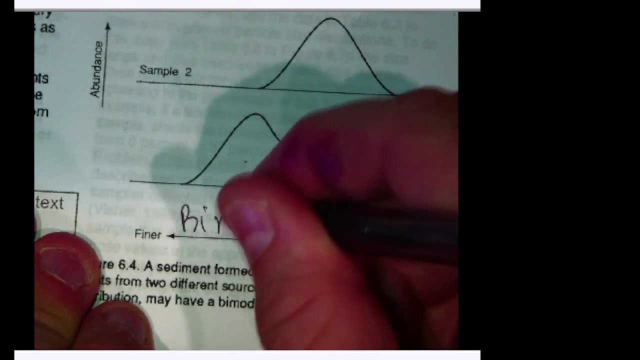 size, but here's a sample. so another beach right or another location along the beach where the particle sizes have two peaks right, and so we call this a bimodal distribution. there's two modes, modes like kind of an average, right, so this is unimodal. okay, one mode and this is bimodal. two modes, right, and you can. 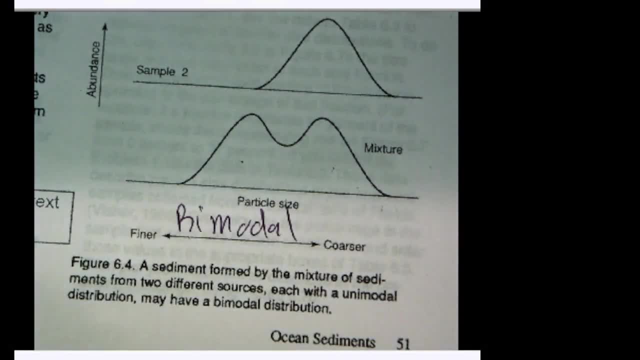 even in theory, have trimodal and all kinds of other ways to describe that distribution. so we might, when we're doing scientific work, you might have a bimodal distribution and you might have a bimodal distribution. or when we're studying this stuff, we might say, oh, here's the full, here's a. 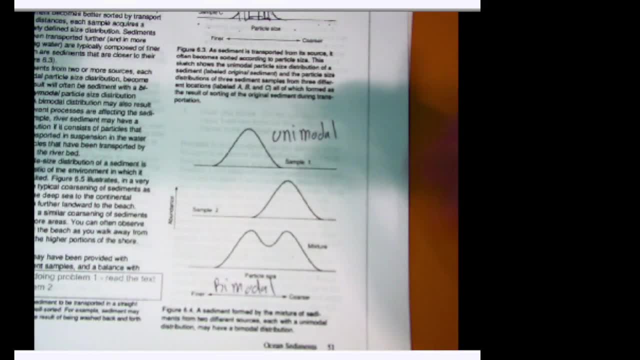 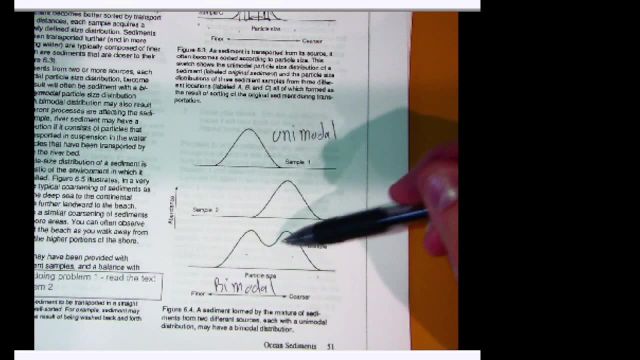 chart of every grain size that was found in that sample, and there's a whole bunch of numbers to look at. we might say, instead of providing a table of values, you might just draw the histogram right. or we might even just say that this sand had a unimodal distribution. this other sand had a bimodal distribution, centered. 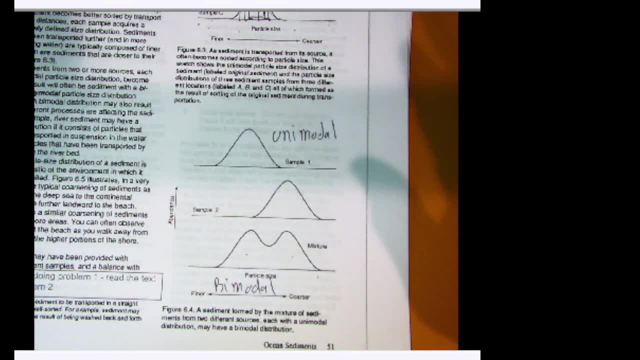 around the, you know, the coarse sands, or centered around the lines and and the cobbles, or something like that. so we can describe it in a lot of different ways, some with more and more finer details. right, so just being able to describe it in words ends up being useful. so in this lab, since it's 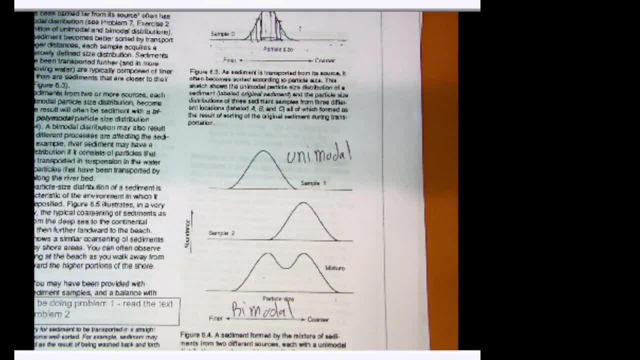 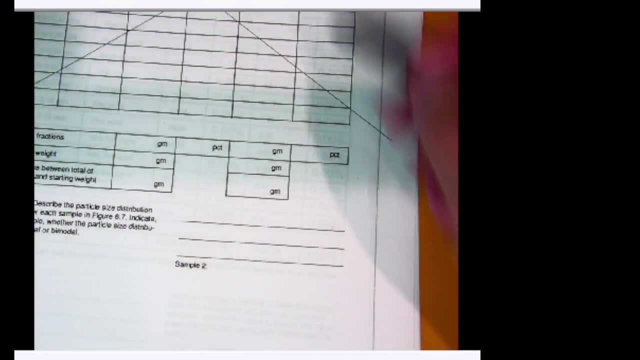 online. you obviously aren't collecting sand and running them through sieves and all that stuff, right, um? so we'll skip past this for you. so there's this, this chart. that's x'd out. you don't need to use this, because this is for when you have the. 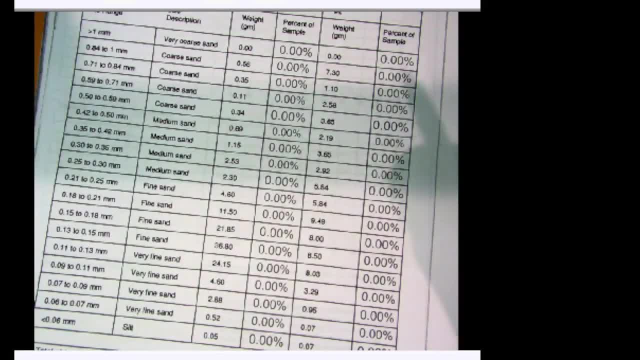 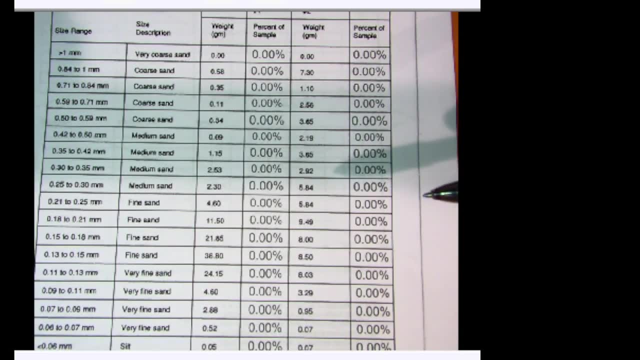 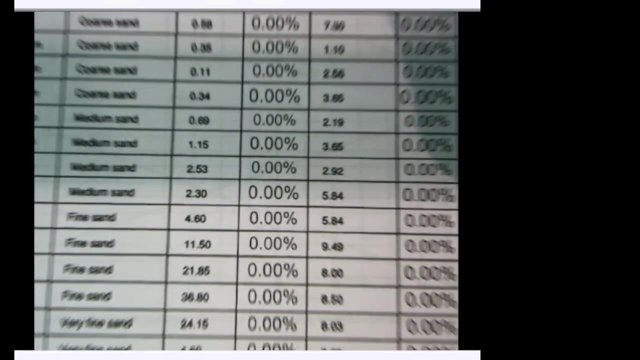 samples and you're running through them. you instead have this chart: okay, and so on the PDF. this chart is filled, these zeros are empty and you have to put down the value, so you have to calculate what they, what these values are. so let's just look at this. I'm going to zoom in a little bit, so what you have here is: 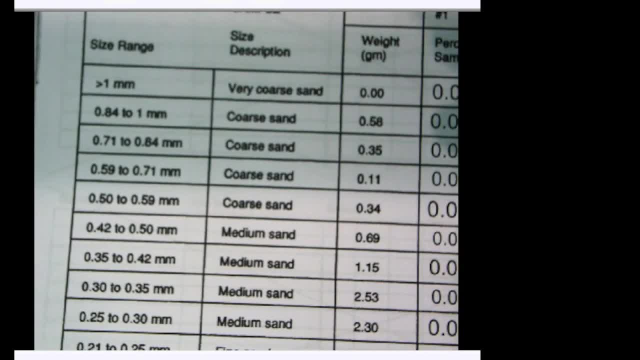 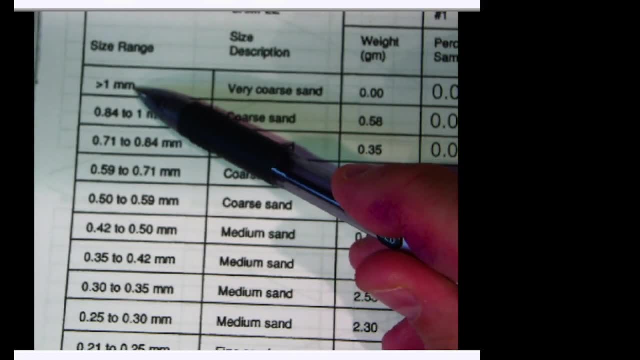 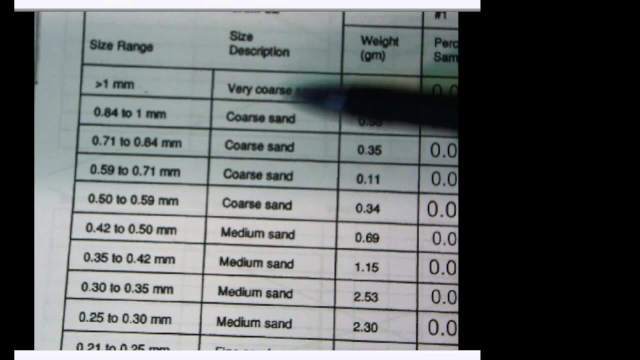 a chart showing this is kind of typical of what we would work with. it tells you this: the actual, like linear size right, the, the millimeter or meter or you know, micron measurements that you're using the size terms that those correspond to. so coarse sand isn't just any kind of, you know larger grains, it's these. 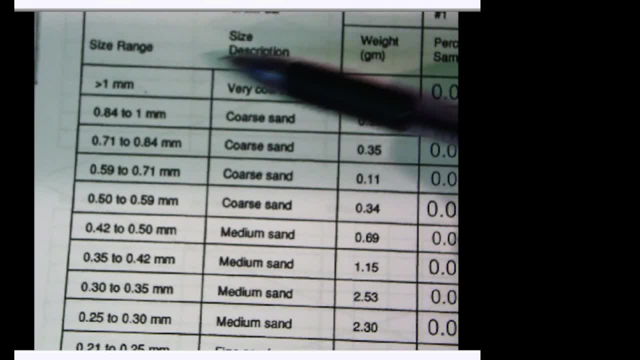 particular ranges of sizes, and so this is all descriptive. and then here we have the weights that was measured in this experiment, right? so it's as if someone else did this experiment and weighed out the sands and separated them and everything, so you have none of this sample is very coarse. 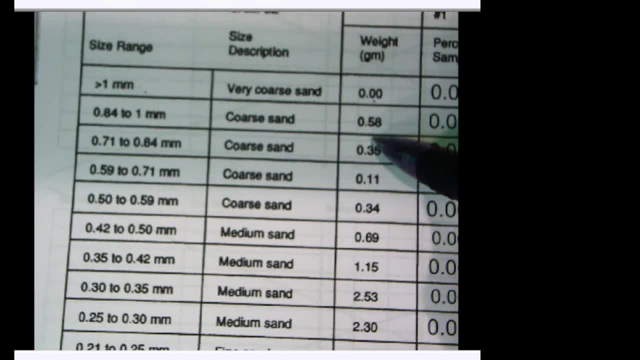 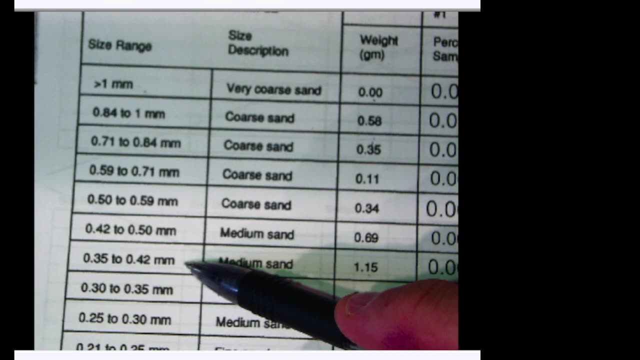 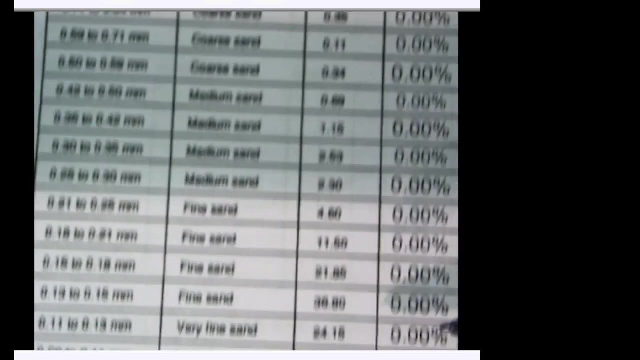 sand. only half of a gram is this range of coarse sands. here you have just a little bit more than one gram. that is medium sand in the 0.35 to 0.42 range. okay, you can so. so you have all these measurements here, and then, if you look at the bottom, there's all these weights. they are then. 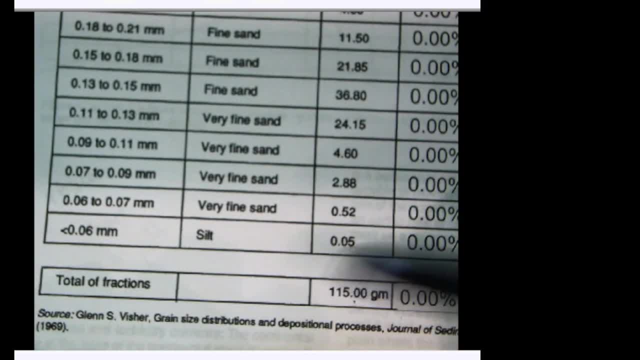 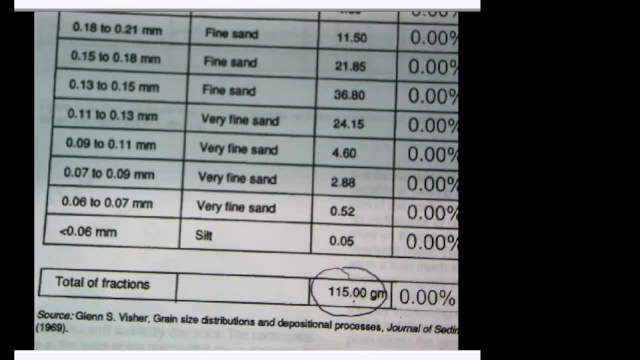 added up right, and so actually, really, what you would normally do is you'd weigh the sample before you even started separating it, and so this is the total weight of the sand sample, the original weight, and so each one of these other measurements you can do is you have to divide them by the total weight of the 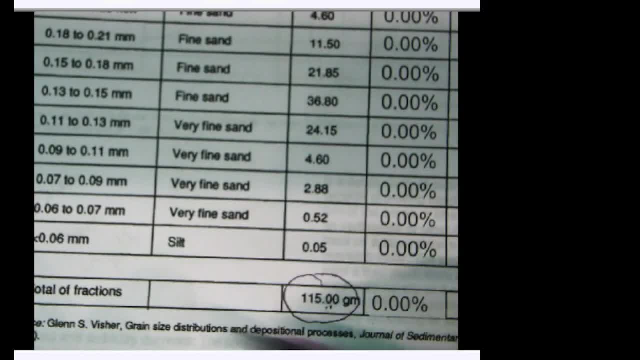 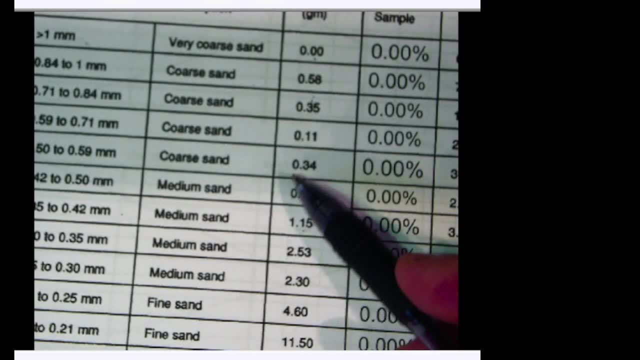 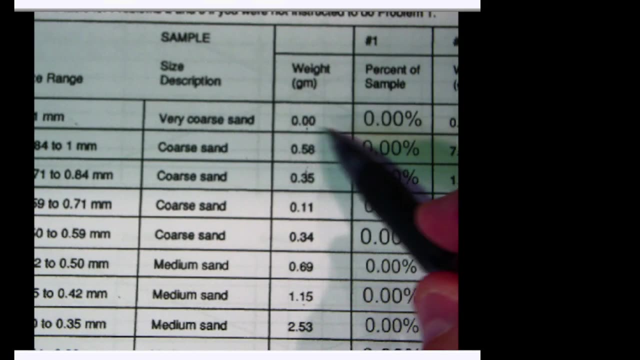 sample, and so what you want to do is you want to calculate what percentage of this whole sample is silt, what percentage of this whole sample is coarse sand in that range, right, so like quickly, what sample percentage of the sample is very coarse? and well, zero percent, so you can leave that there. so 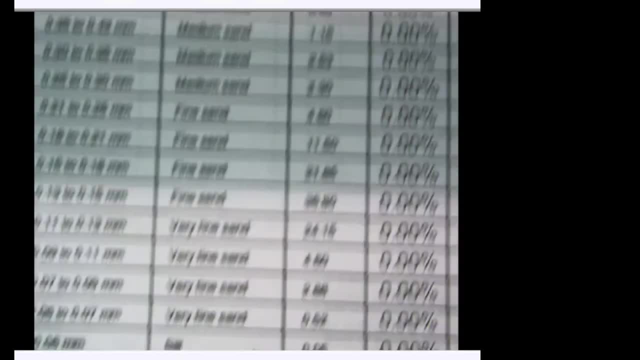 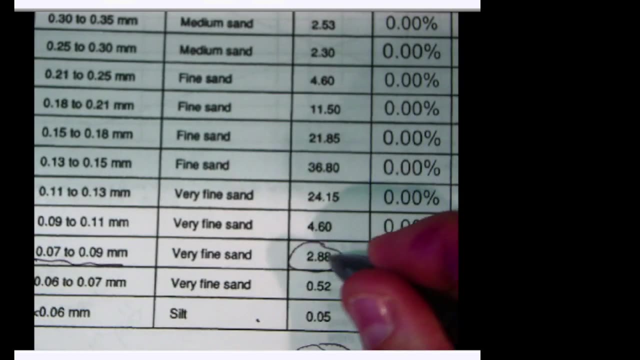 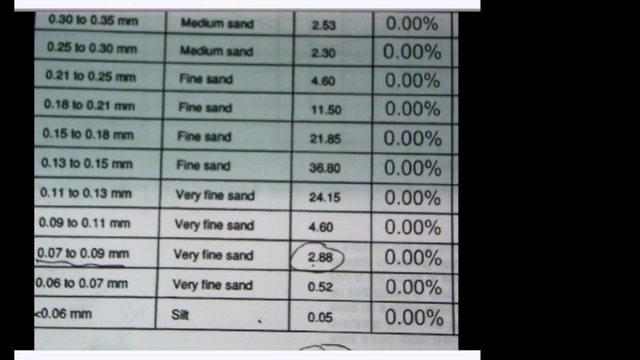 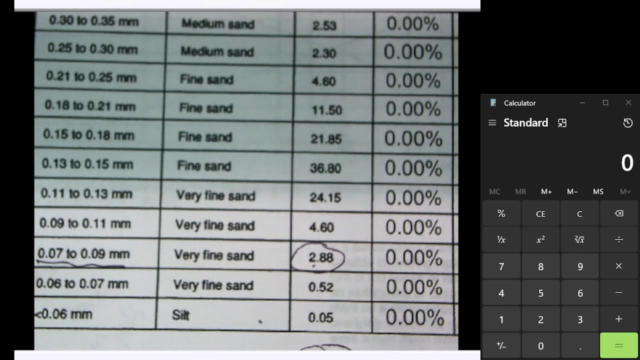 right. so let's take a look at that calculation. so here you have very fine sands in this size range: 2.88 grams of the total sample. are this? what percentage is that? so you can take your calculator: you have 2.88. okay, you have. 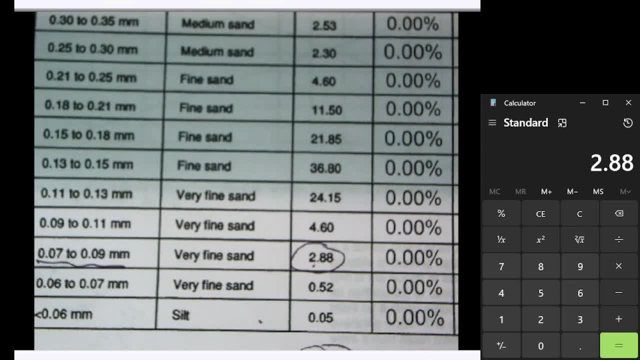 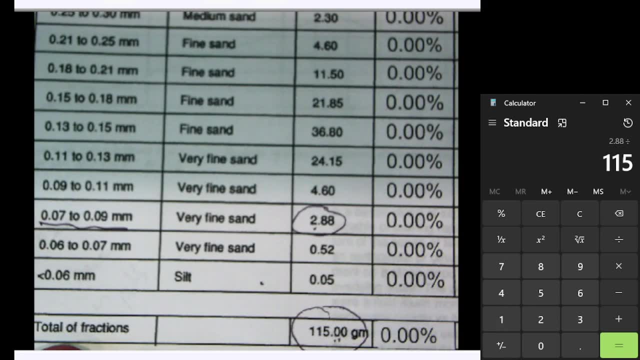 2.88 grams of sand in that size range. divided by the total right, which is 115 down from the bottom, that equals this number. multiply that number by 100 and you get 2.5. so in that case we have 2.4. we're gonna write this. we have two. 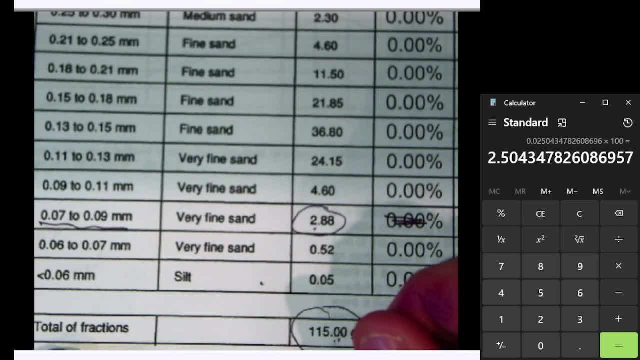 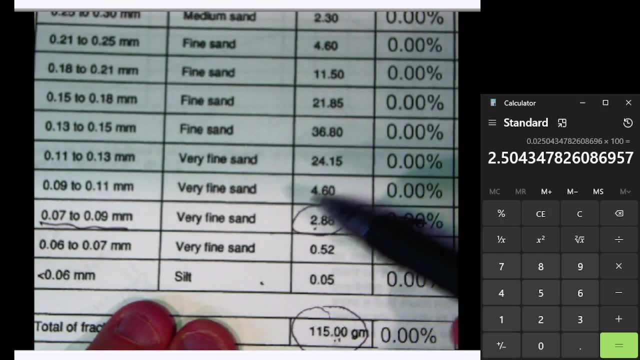 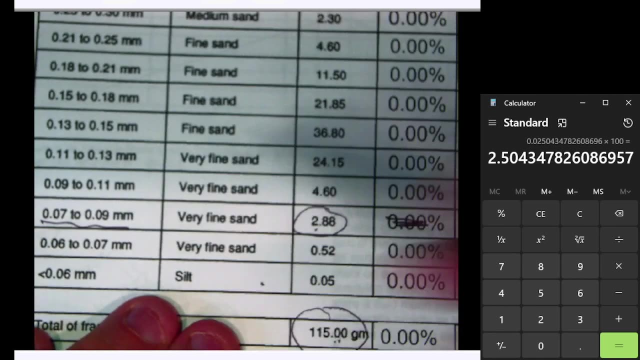 others right here just 2.50%. so 2.50% of this entire sand sample is very fine sand between 0.07 millimeters and 0.09 millimeters. so you're gonna do that. that count. so you took the, you took the sand. 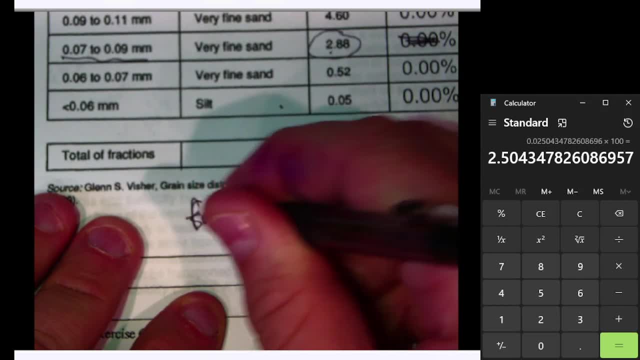 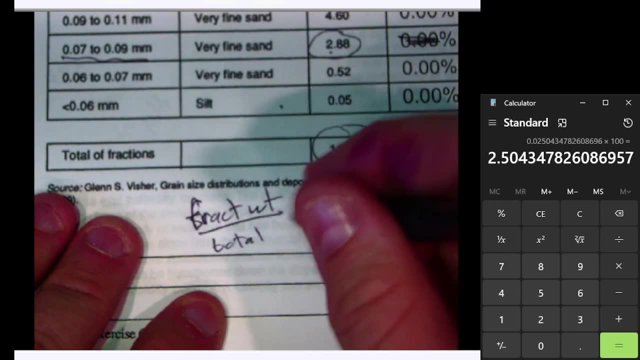 weight, or the. what I should really say is the fraction weight. you divided it by the total weight, the whole sample, and then you multiplied it by a hundred. because you get a small number, you have to multiply it by 100 to get percentages right. that's gonna equal a percentage, so you're gonna repeat that. 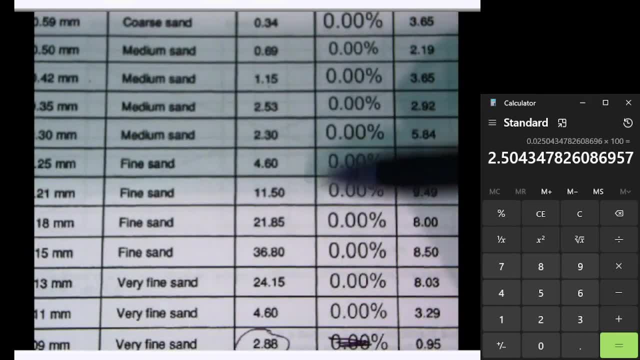 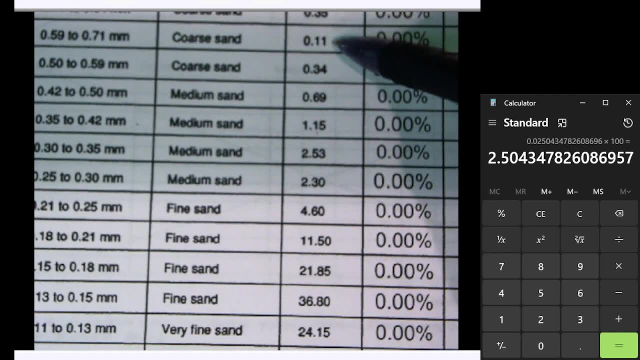 for every one of these. okay, and you're gonna fill it out on the PDF and just looking at it, point point: one: grams out of about over a hundred. point six: nine grams out of over a hundred. these are gonna be very small percentages: 21 out of the hundred and fifteen grams. 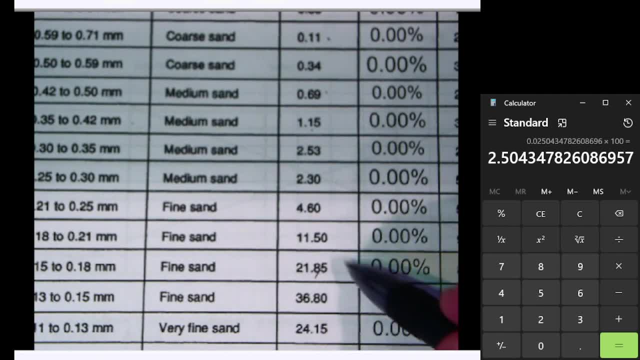 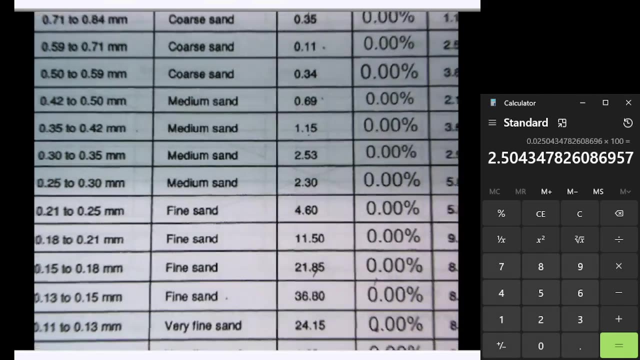 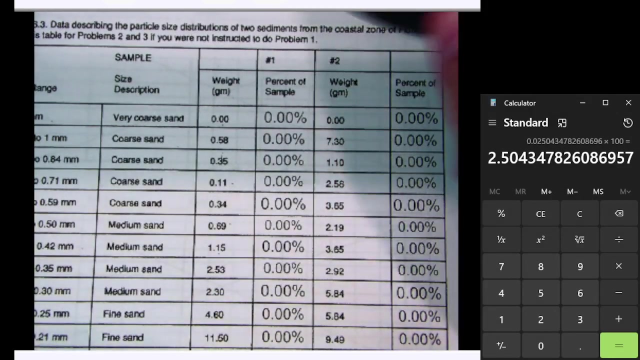 are. are this kind of sand? that's gonna be a large percentage, right? 36 percent, sorry, 36 grams. are this kind of fine sand? well, that's gonna be a large percentage for that one. now, looking at the chart again, you'll notice that it's it's got two parts. so over here there is. it's maybe not obvious to everyone. 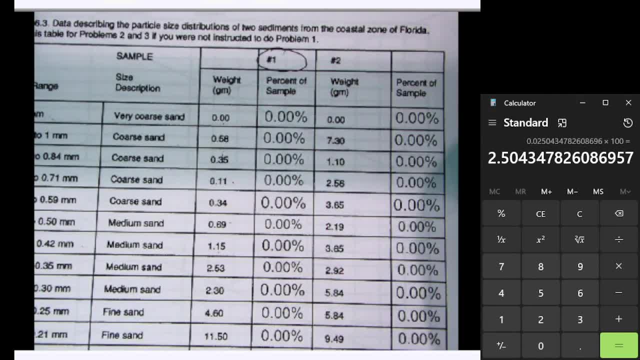 there's sample one and then we do all this stuff for sample one. so someone went out to a place, they dug up the sand, they ran it through the sieves and these are the weights they got. then maybe someone else at the same place, or the same person at a different place, took another sample. 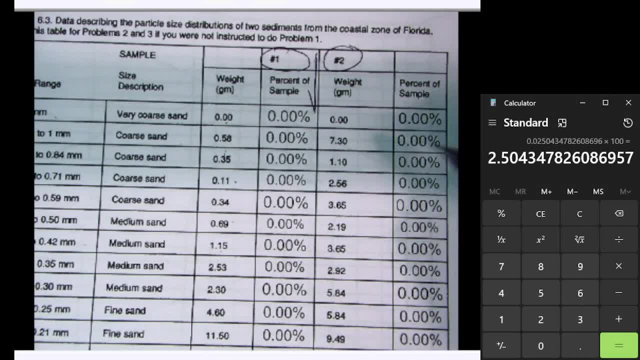 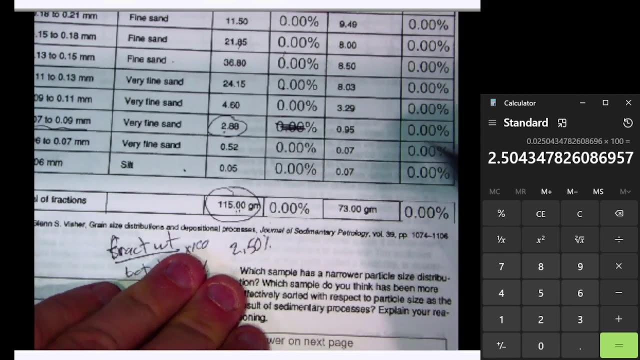 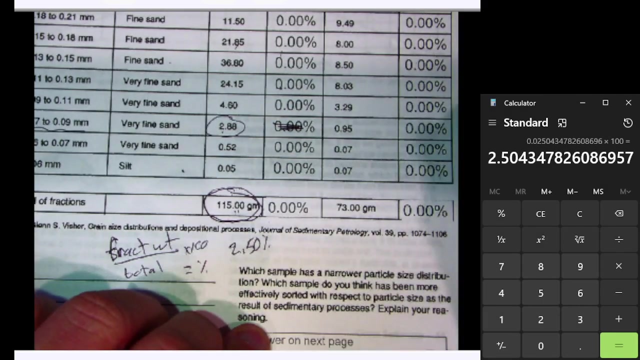 another shovel of that sand and they ran it through the sieves, sent the same sieve stacks and they got these weights. you're gonna calculate the percentages here also. and so now notice: for sample one, the total weight was 115, that's how much they shoveled into the sieves. and for sample two, they don't have the same. 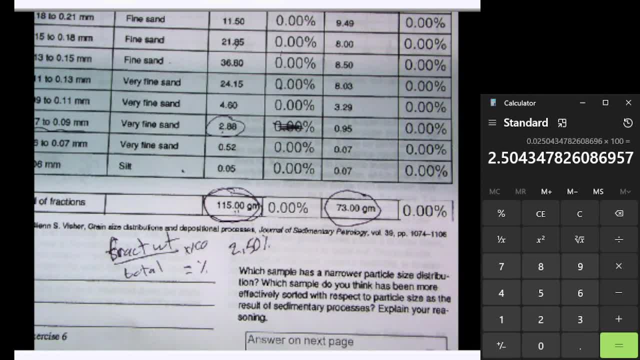 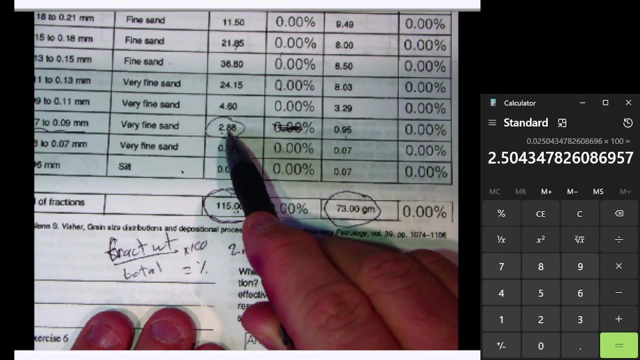 weight, it's a different amount that was put into it. so this is actually kind of a nice example, because how can I compare the sands from these two places? right, I can't just look at the weights of any particular size fraction right now, if I, Because maybe at this location maybe I collect like a thousand grams of sand. 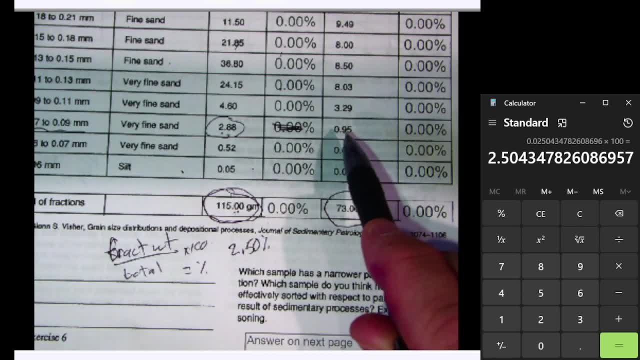 And then at this location maybe I only collected a couple of grams, So the absolute weights aren't really useful. I need to have it turned into these percentages And then if this sand has a different percentages of these sizes than that one, that might be useful. 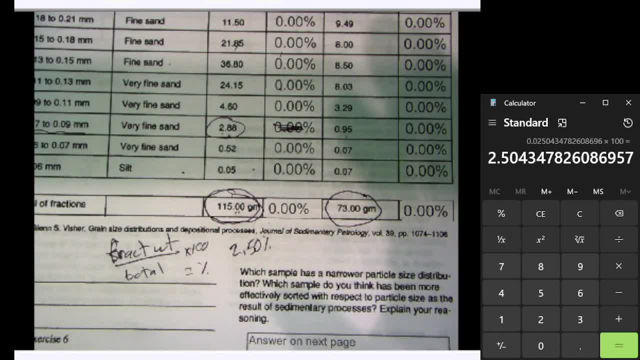 If I was told that I had a whole bunch of sand samples and two of them were from the same exact location, I would expect them to have the exact same spread of percentages, right? And other places might have a different spread of those percentages, right? 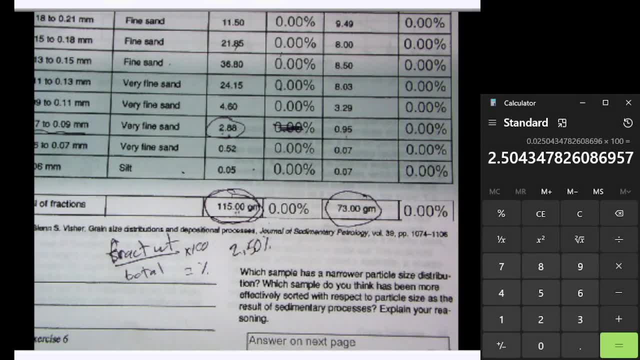 A different profile. So this can- you know very vaguely- be used in like forensics to tell us if a sample corresponds to one location or another, or something like that. So it's useful. It's useful in a lot of different ways. 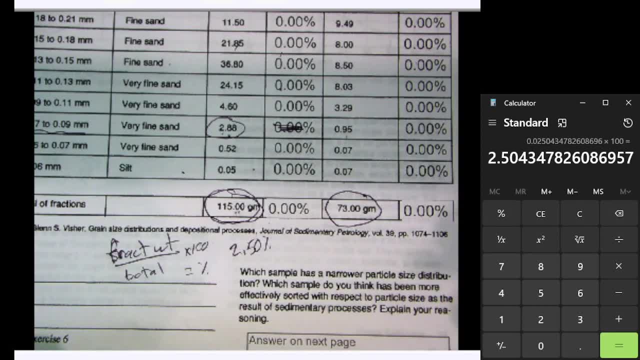 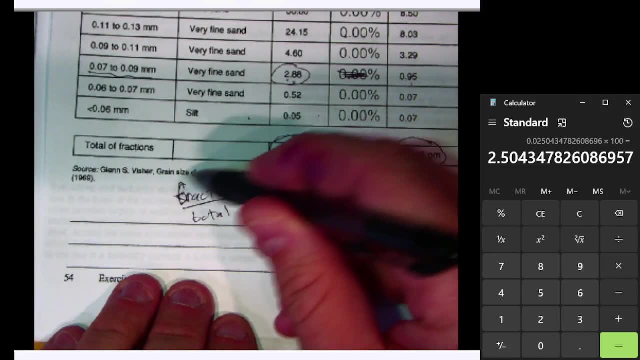 It's useful for classifying and describing these sands to geologists, And it's useful for you know other kinds of work. Okay, So again it's a lot, but you're just taking the weight of that fraction and you're dividing it by the total weight of the whole sample. 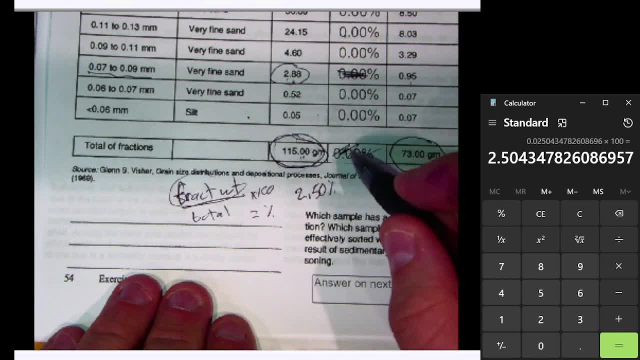 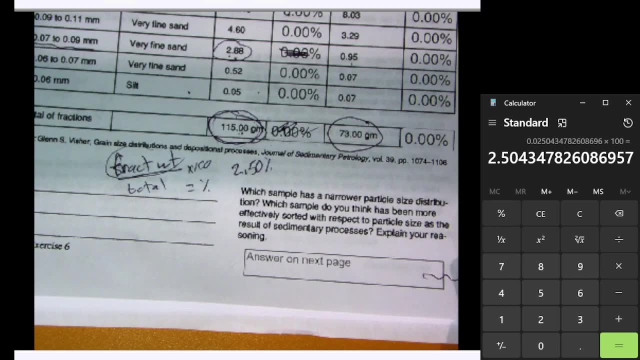 And so this doesn't, this is 100%, So it doesn't matter because it's everything, right, Okay? Then it asks you some questions like: oh yeah, Okay. So once you've got them, you then And go to the next part. 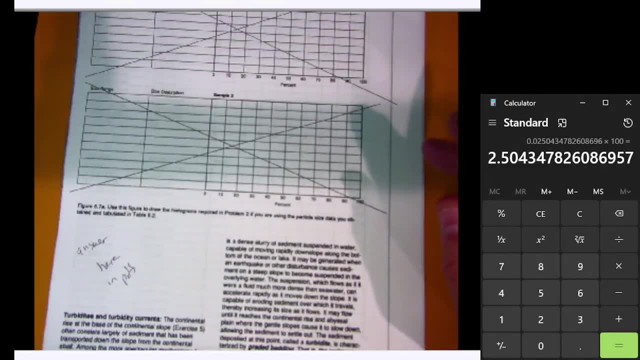 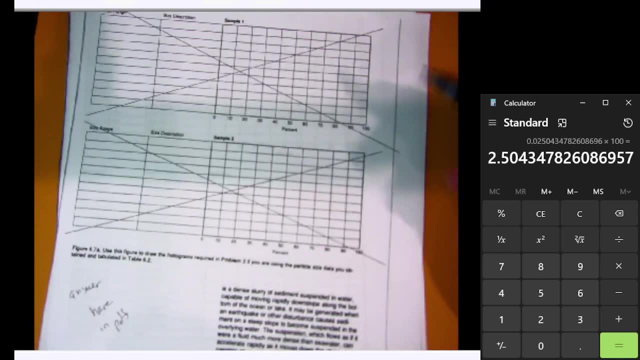 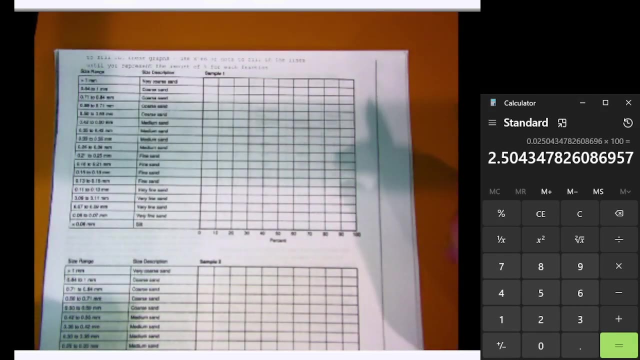 So on the next page, let's zoom in a little more. You don't need to use this. This is X'd out because it's it corresponds to when you do the experiment in person, And then over here we have the chart for you to use for the online version, right? 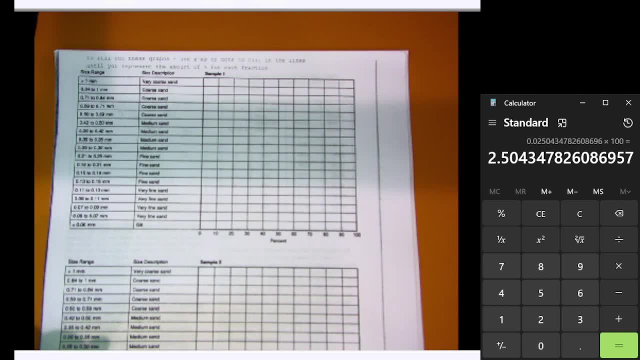 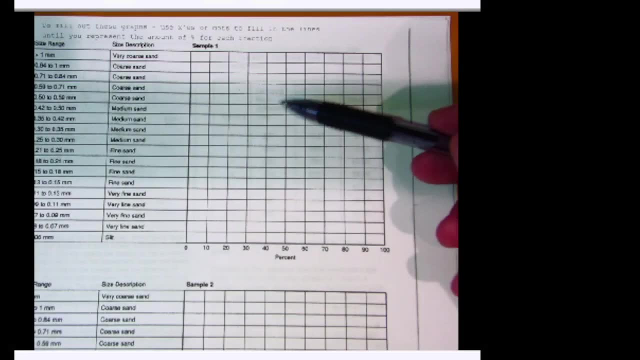 Where the data was given to you. So in this one I'll zoom in again. You have two. Well, first off I'll go back. You have two different tables. Table one is for the first sample and table two is for the second sample. 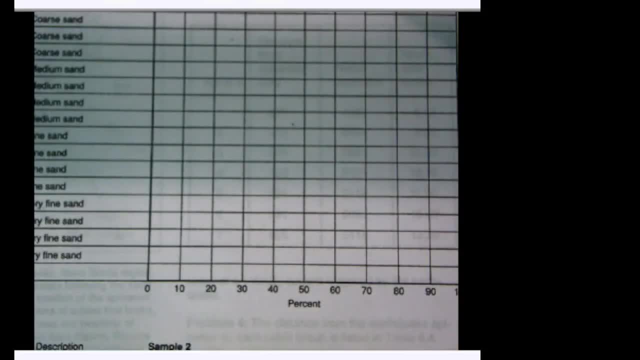 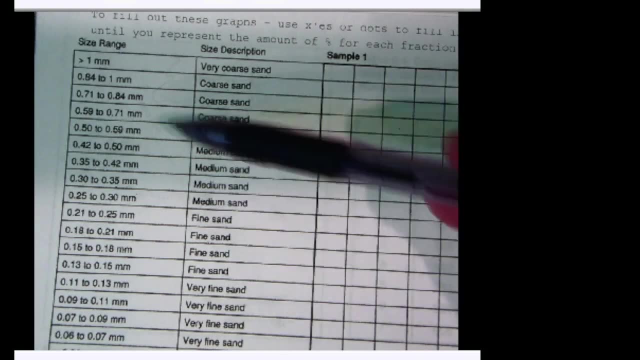 Okay, And if we can move in a little, If you look at them, they look very familiar at this point. You have the range of sizes, Okay, The terms and the ranges. these correspond to the same thing on the other table. 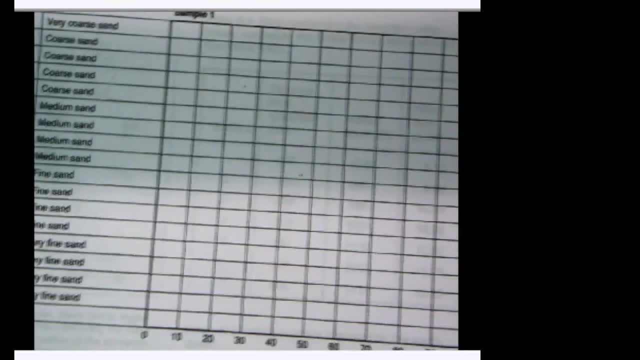 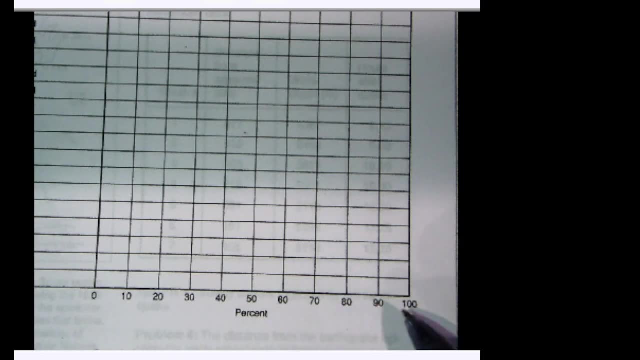 And then you have this. you know this table to fill out. How do you fill it out? Well, if you look at the bottom over here, it has an X-axis in percentage and it's very blocky. It goes from zero to 10,, 10 to 20.. 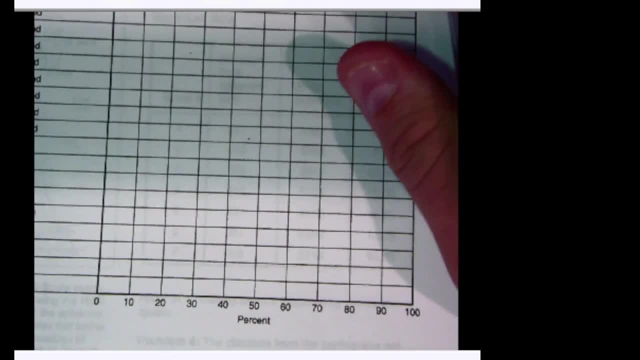 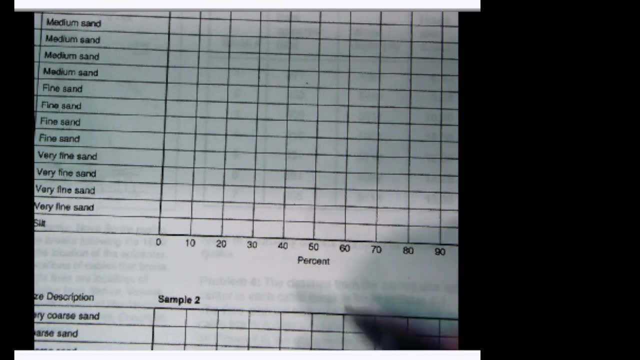 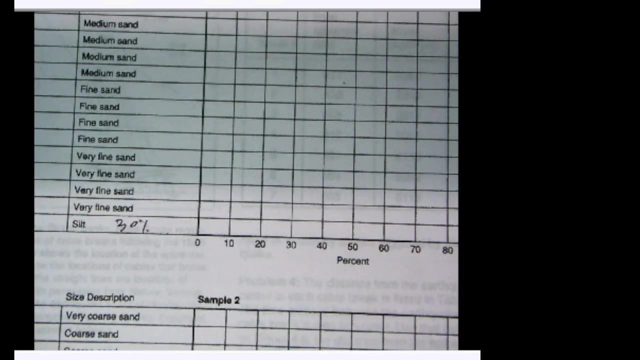 So each square is 10%. Okay, So let's say this is wrong. but let's just pretend that in sample one the silt right. Let's pretend the silt was 30% of the sample right From that other page. 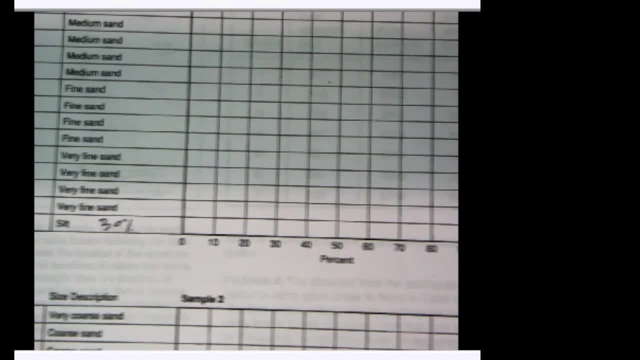 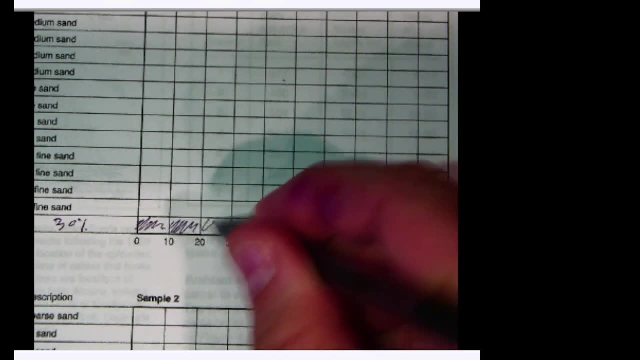 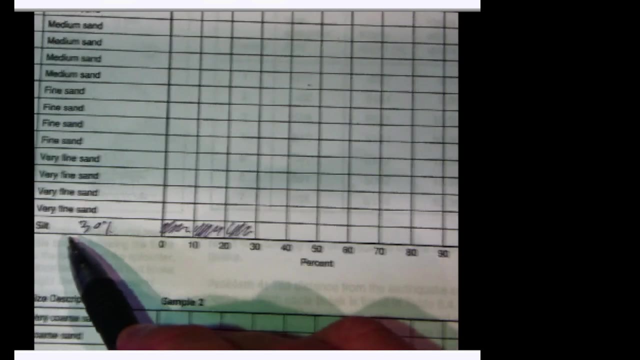 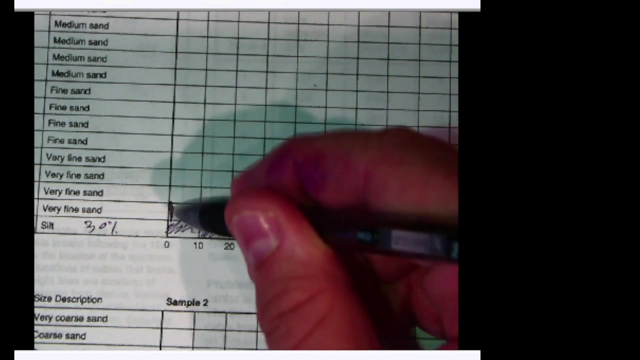 You can then show that here by filling in this block and that block and then that block, And so anyone looking at this will say, oh, this sample right was 30% silt, And then it might only be you know 1% of this other guy. 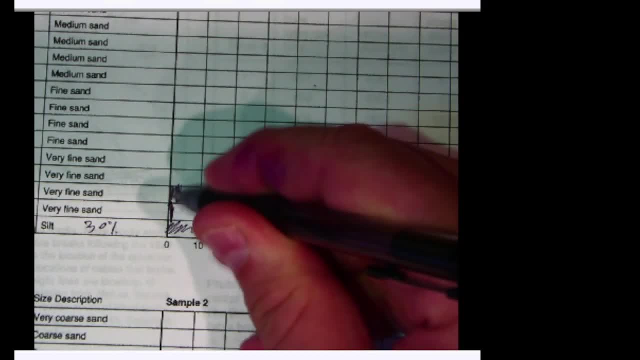 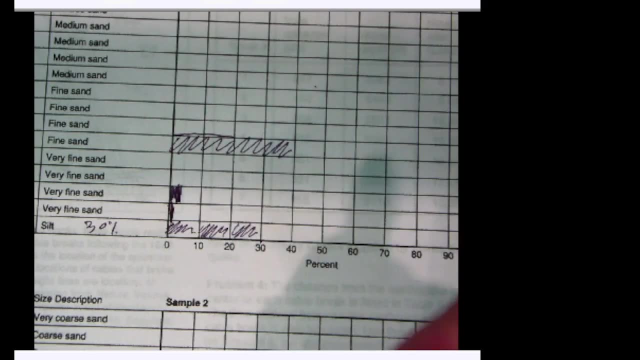 And maybe there was, you know, 5% of this guy And then maybe there was, you know, a large percentage of this piece and another large percent of in this size class. You can estimate. you know, between here and here is 45.. 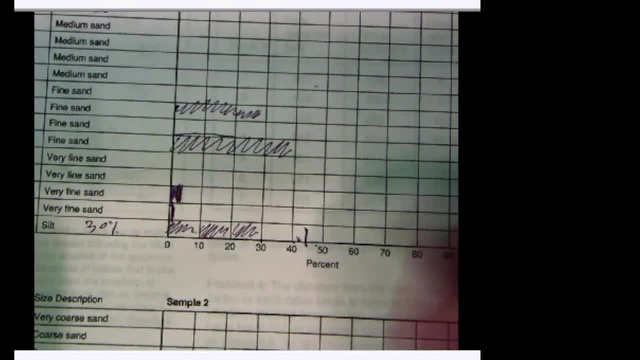 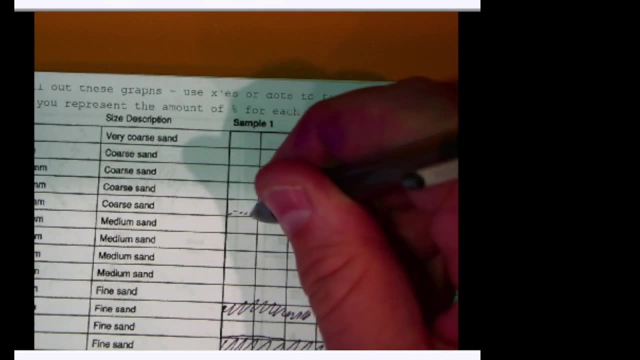 There's also five little marks there. You can get it pretty close in the PDF. What you can do is you can just type little dots or Xs, right, or anything you have to do in order to just fill it out, And this can be pretty approximate. 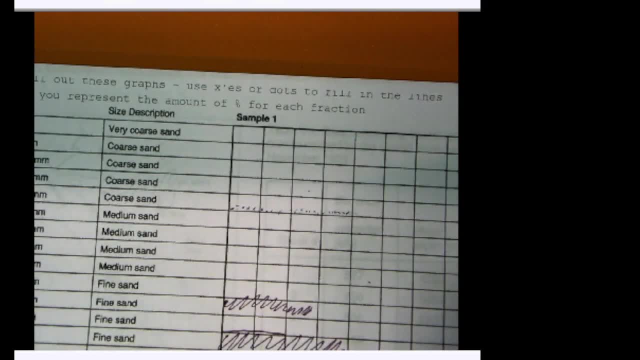 Okay, I just want to see people have put something in. you know, if you have 45% instead of 50, that's not wrong. If you have 30 instead of 50, that's obviously pretty wrong. right? So you would fill this out. 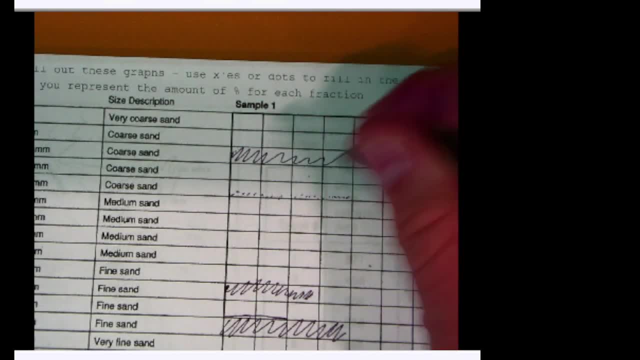 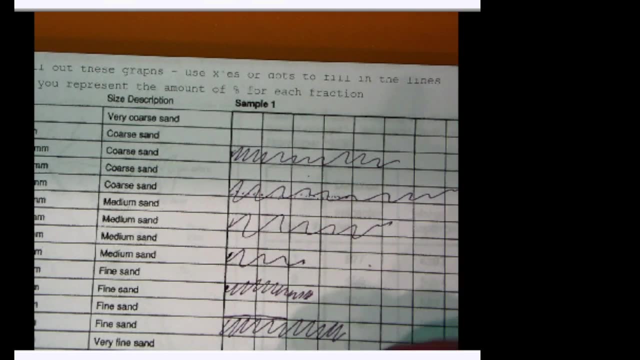 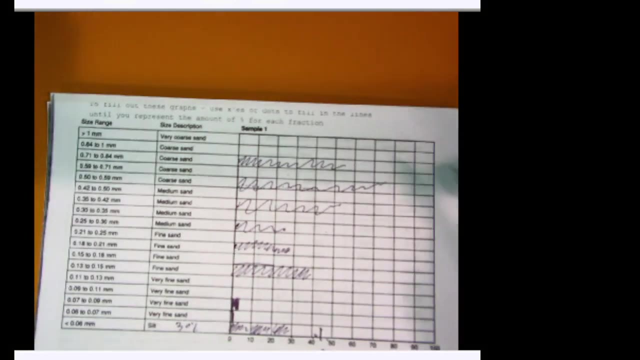 And what you're going to end up with is a bunch of this doesn't work because it all adds up to way over 100%, But you might get something like this kind of distribution And that distribution. What you've been doing is you're actually making a histogram. 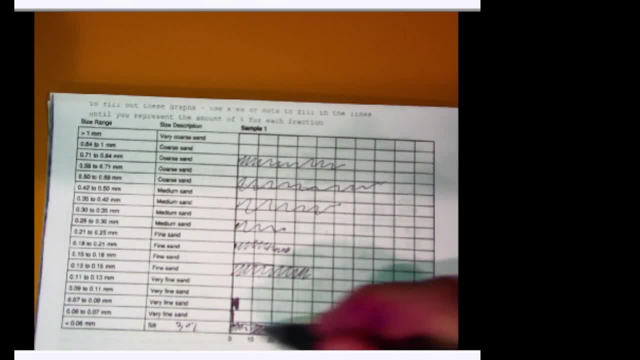 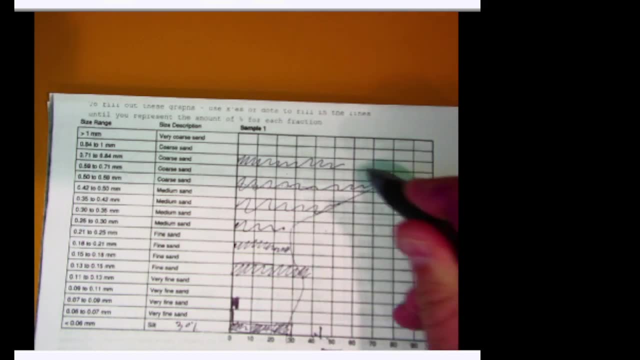 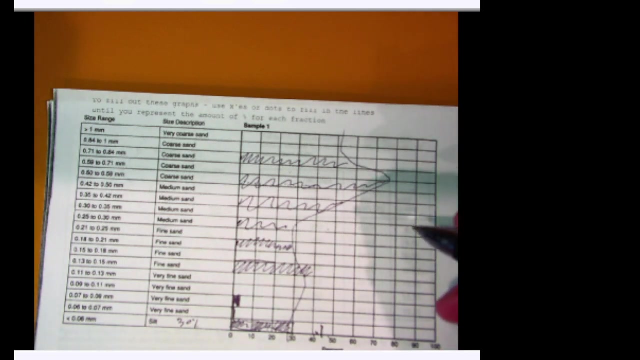 So once you filled all of them in, so a histogram is like a bar chart and then the bars go out to the percentages of each thing And you could even start connecting the tops of the bars And that should look like, or could look like, the previous pictures that we saw right. 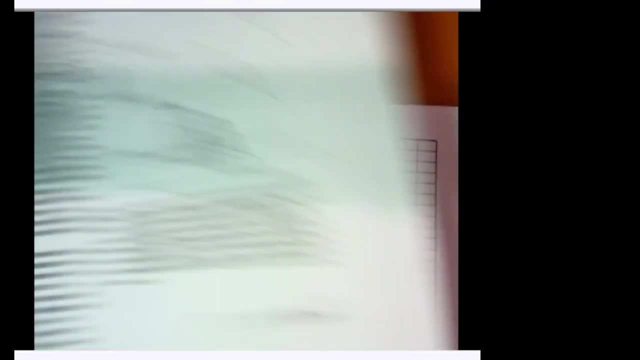 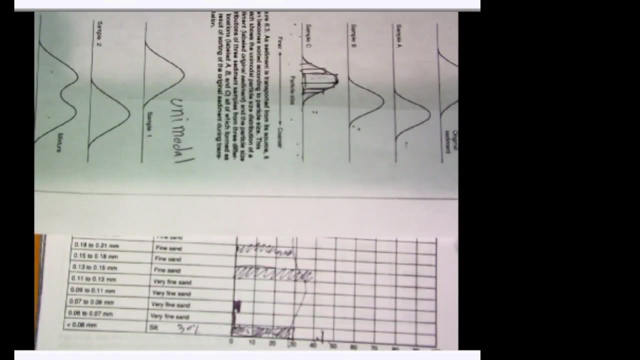 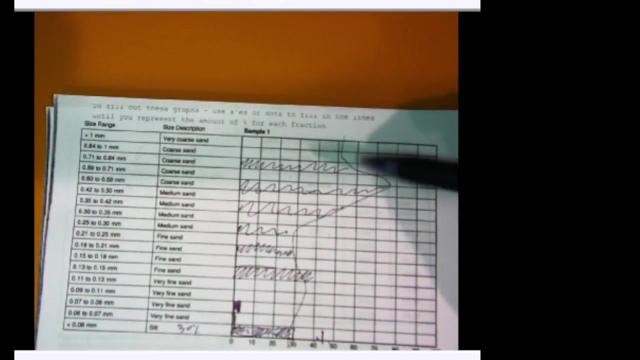 It could look like those other distributions that we saw, So they could look something like this. So if we took this on its side, it would- it might- resemble this chart pretty well. Okay, And then what you want to do is, at some point it asks you to describe these. 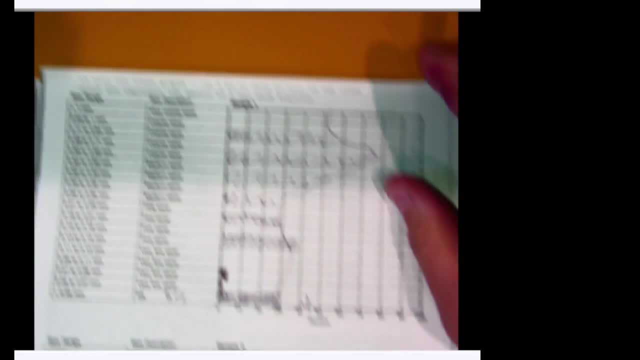 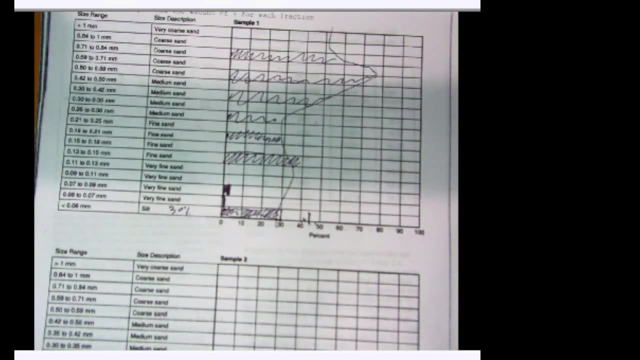 So you've described- you've already described them right. You made that table that has the numbers, So anyone- that anyone that wanted to read your report- could look at those numbers and know exactly what they were. Someone could also quickly glance at this histogram that you've created. 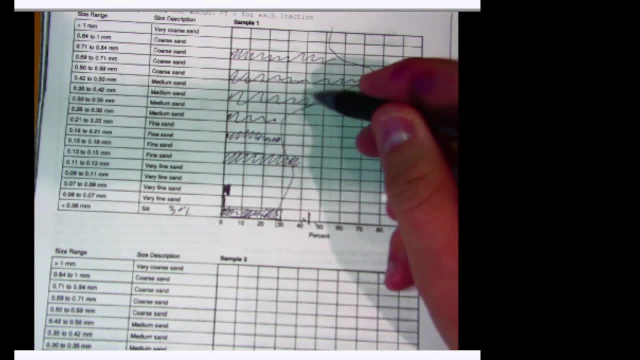 You don't need to trace the shape right, You just fill out for each and every one how how much they are, Or you could just describe it So here this might be described as a unimodal distribution centered around the coarse sands. 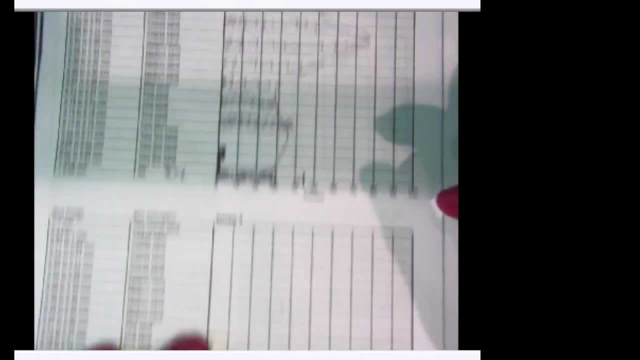 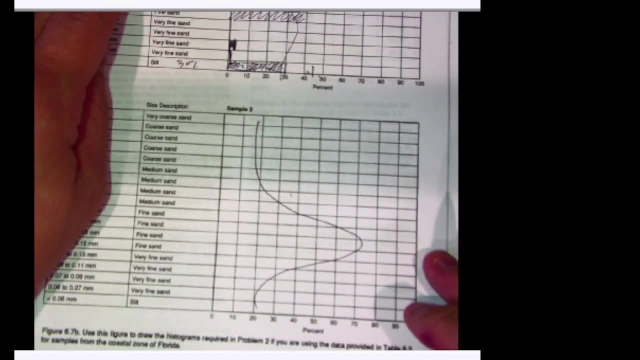 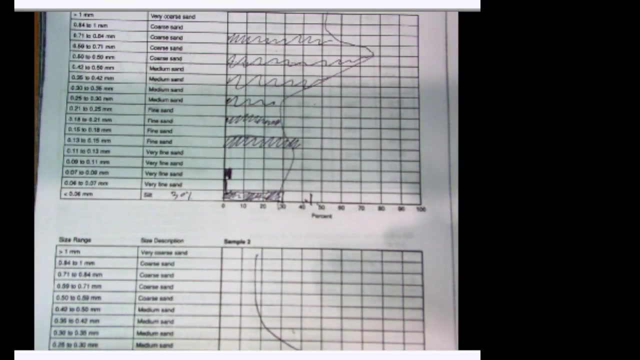 I just made this up, though, And so then you can compare these two samples very rapidly, right, Looking at the picture, they might have very different charts to them, right, So you can describe these samples and differentiate them or make Other statements about them, using this basic information. 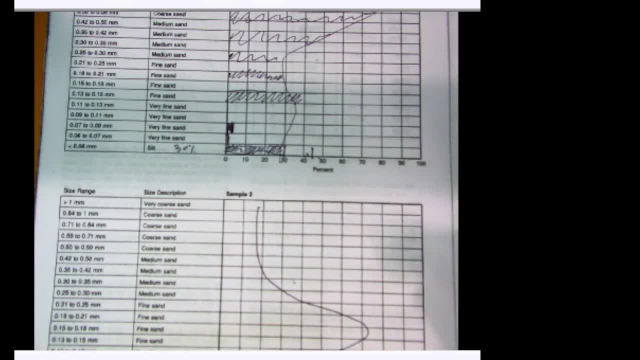 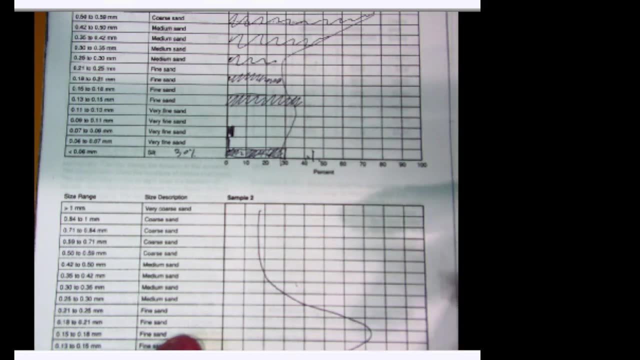 So that's why we have you do it. So this is something that people that work with sediments do all the time. It's like a first description of the sediment samples that we might be getting Now. we might be really interested in the fossils that are present in there, or the chemicals that are present, or it might be sand. 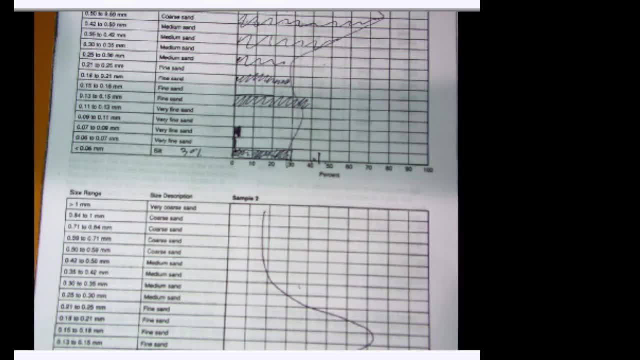 That's not just taken from a beach. It might be sand that's taken from the deep ocean and it's from you know, a million years ago. So there's other things we might want to get, but this is the first thing we do. 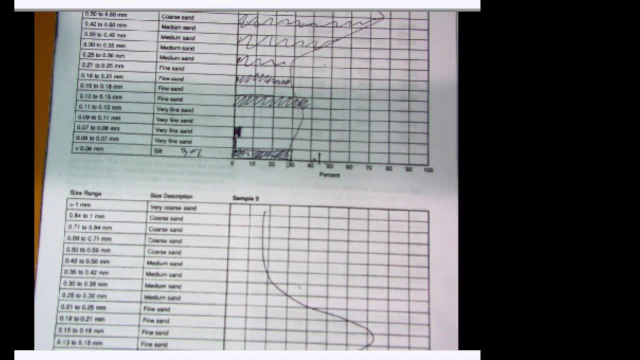 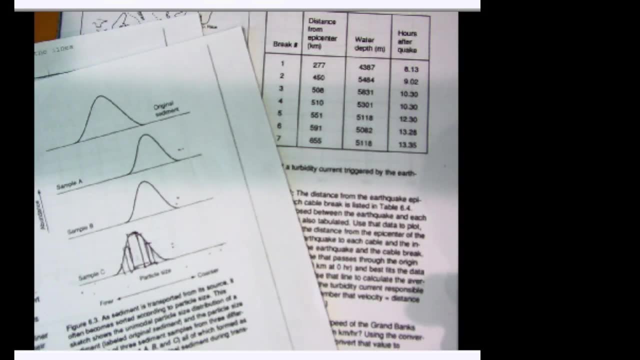 Right, What does we kind of call this? the lithology or sedimentology of the samples? Yeah, So it asks you a few questions to fill out, like: describe the, Fill out these charts and describe the distributions and all that kind of stuff. 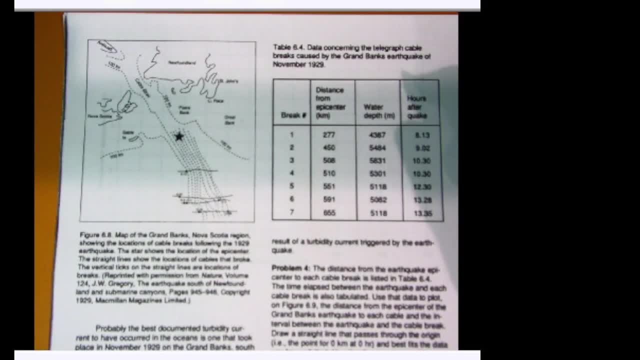 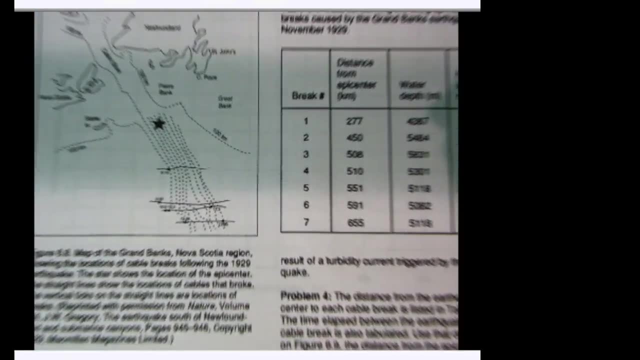 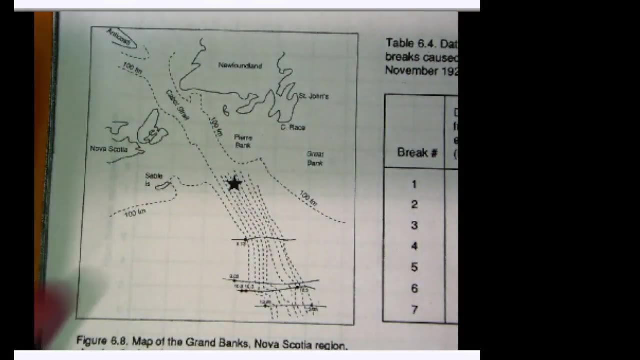 Then it kind of switches modes into this part of the question, part of the lab. So here this is kind of a famous example in oceanography and marine oceanography, marine science. So this little map that's shown here, this is a map of Nova, of Newfoundland and Nova Scotia. it's part of Canada. 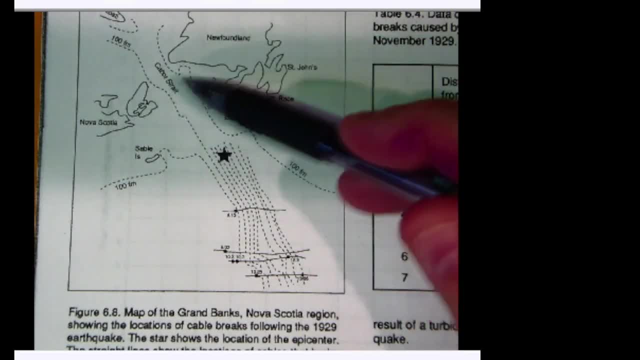 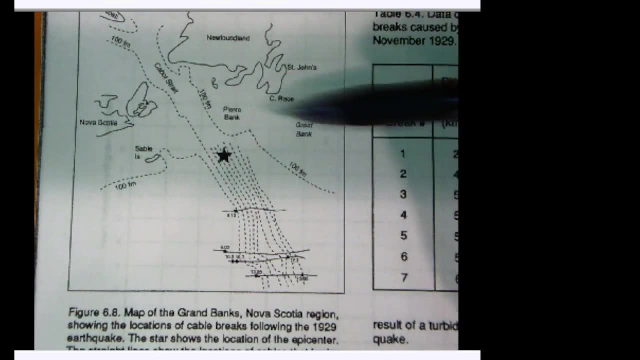 So we have this land here. this is like Northern Canada and Eastern Canada, right? So the US and where we are is way, way down here, and this is the northern part of the Atlantic Ocean And it's maybe hard to see here, but it's showing some topography here. 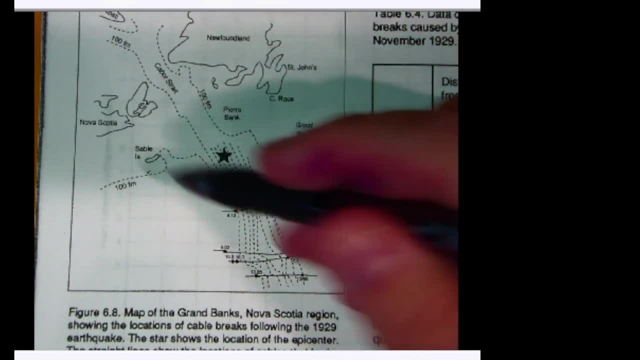 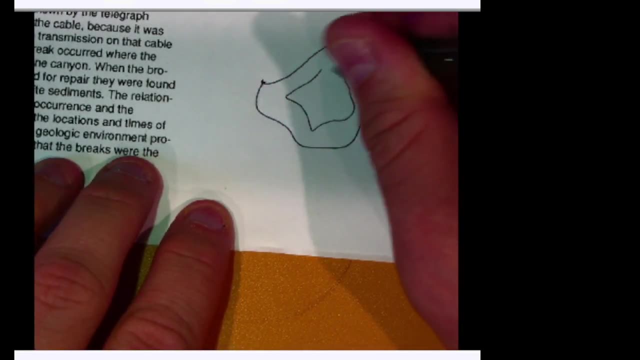 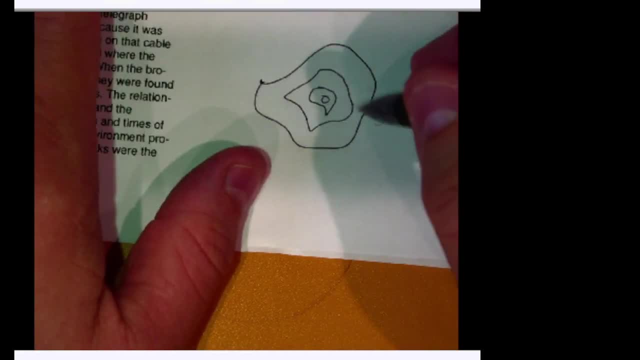 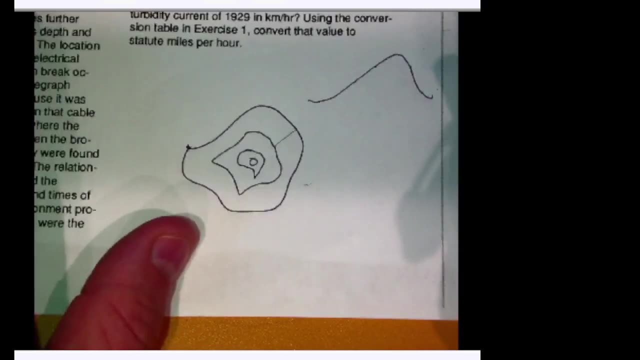 If I'm looking down at a map, right like bird's eye view looking down at the land, this might be what a hill looks like, And so the hill would, in profile, maybe look like that. then we would show it in this way, just like super brief. you know how those kinds of maps work. 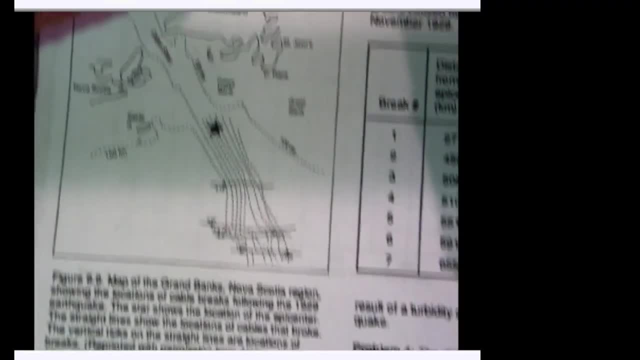 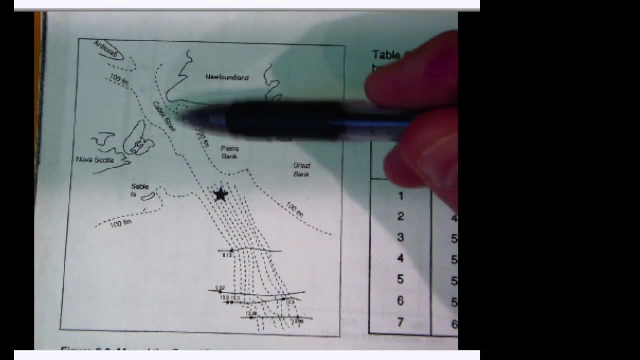 So that works on dry land. it also works in the ocean, And so I'll just. what you're seeing here is a channel. This is a deep, a steep, deep valley or channel in the ocean, right in the ocean floor. 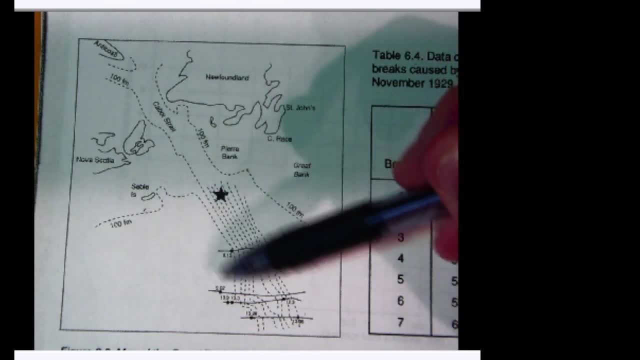 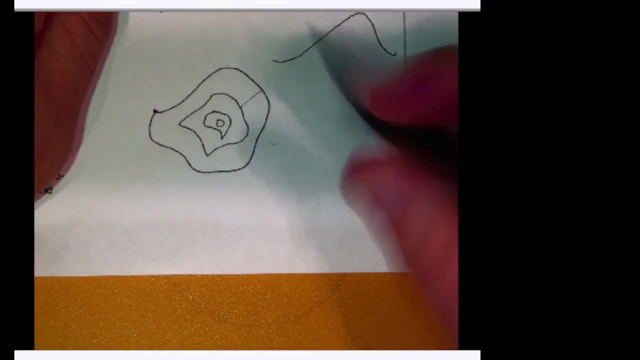 So you have some flat land up here and then you drop down into this channel. So it's kind of the opposite of what we had here, right? So what you're looking at in that picture is you have the flat land and then you go into a deep channel. 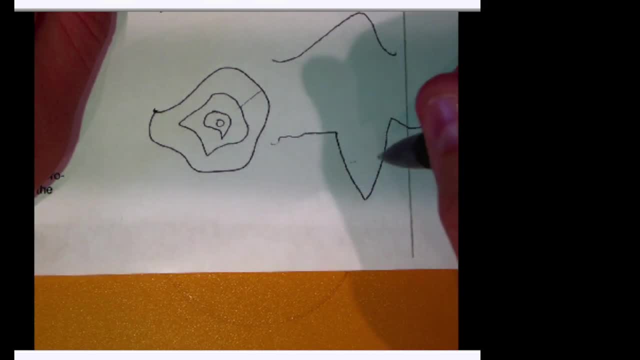 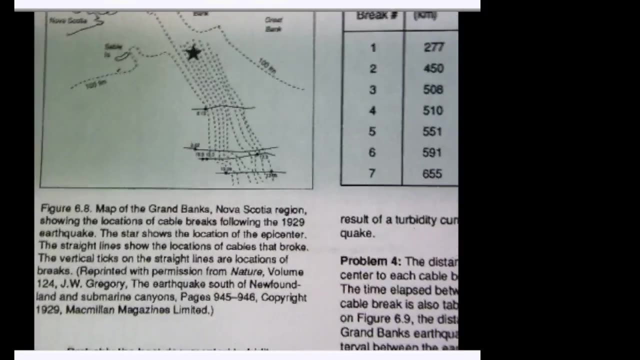 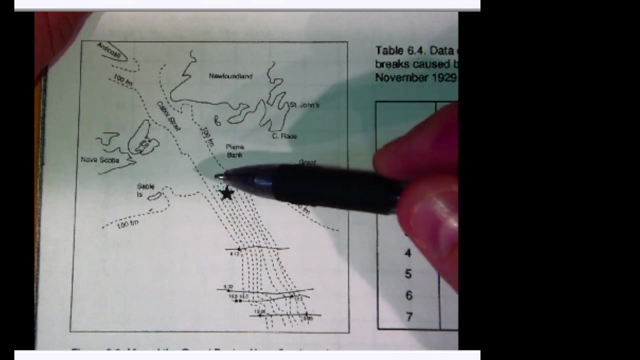 Okay, This is the bottom of the ocean, This is a profile right, and all this is under the ocean, And so that's what the land looks like, And so into these deep channels you sometimes have, well, on dry land would be an avalanche or a mud landslide. 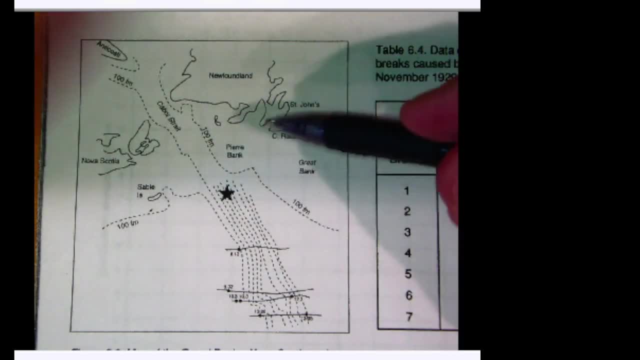 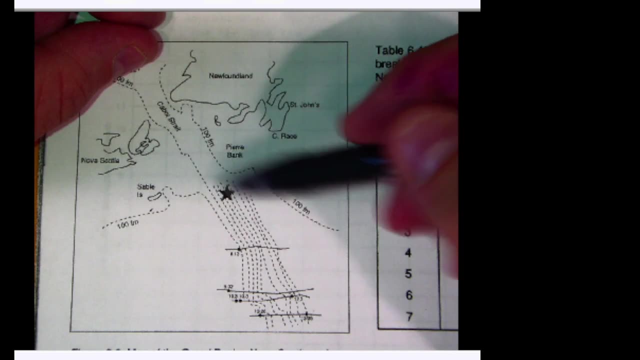 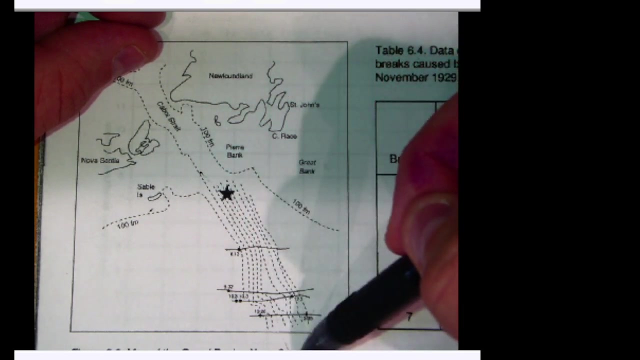 In the ocean we call it a turbidite flow because it's a little bit different, it has a special name, But it's basically a kind of avalanche under the water along those steep cliffs. And so what happens is that in these channels you have these turbidite flows, these collapses that run through the whole channel. 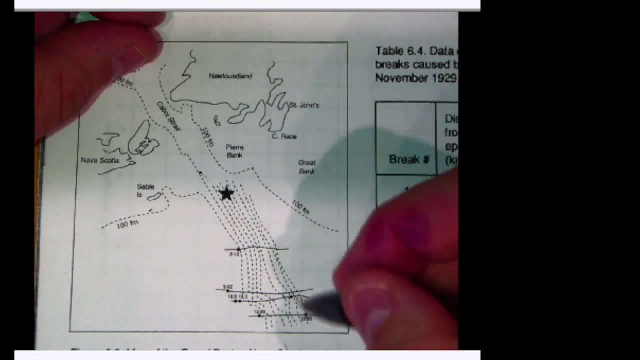 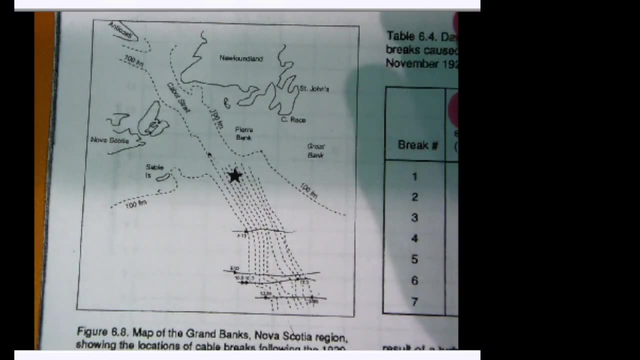 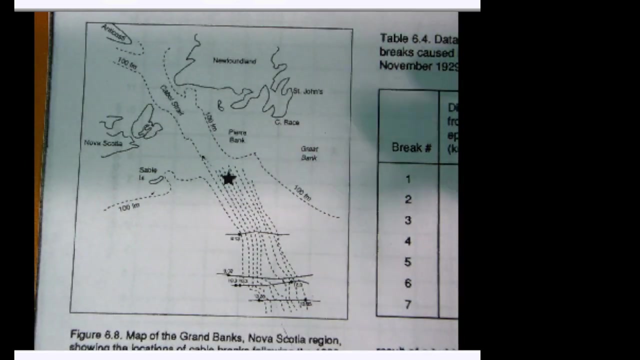 And they kind of clear it out right and scour it out, And then you get a deposit of sediment somewhere at the bottom. Now that happens normally in nature and we weren't really aware of it or we didn't know a lot about these kind of turbidite flows in these submarine avalanches until this event happens. 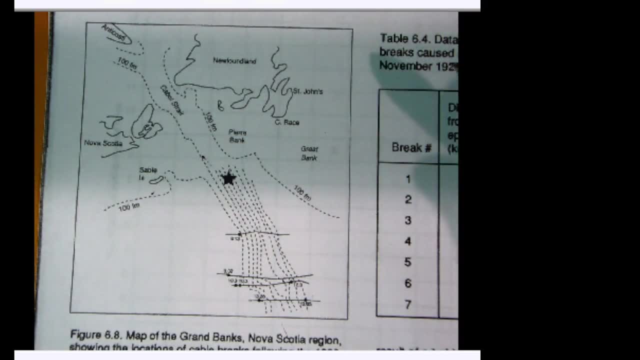 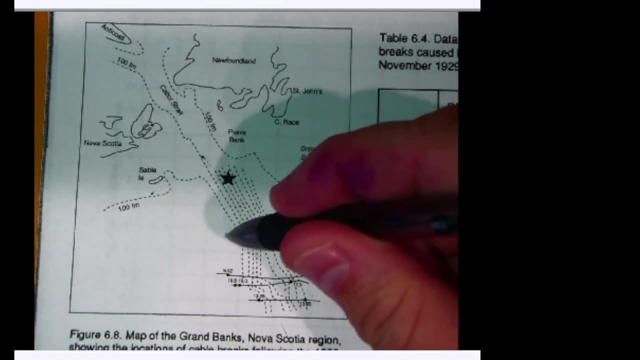 So this is in, I think, the middle, So this is in the middle, So this is in the middle. Okay, Okay, Okay, Okay, yeah. 1930s, 1929, and so the technology then was different from today and they had these telegraph. 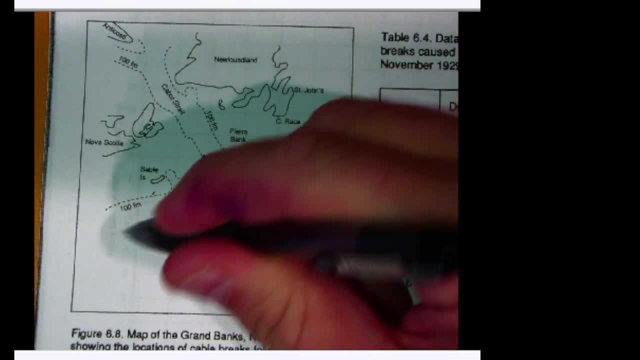 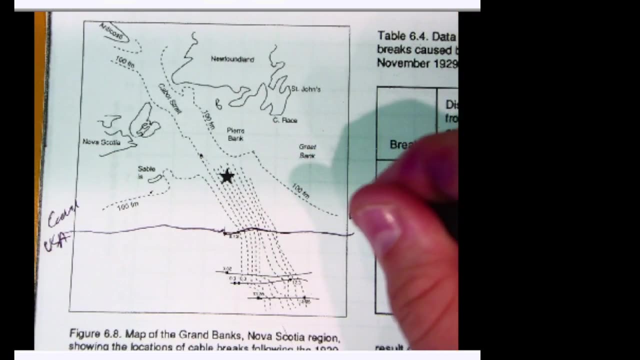 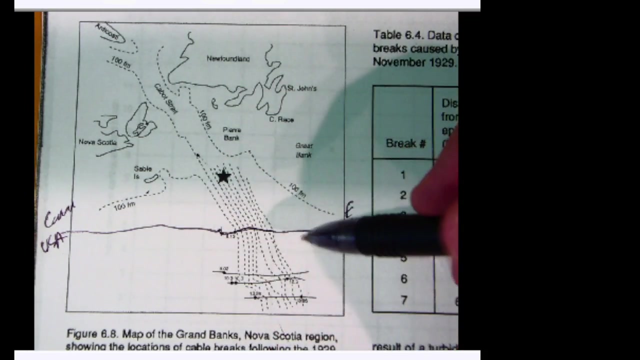 lines and so they're only showing part of it. but these telegraph lines would go from, you know, Canada and the US to like Europe, and this would allow communications between Europe and the US and North America right using telegraphs, right like those like 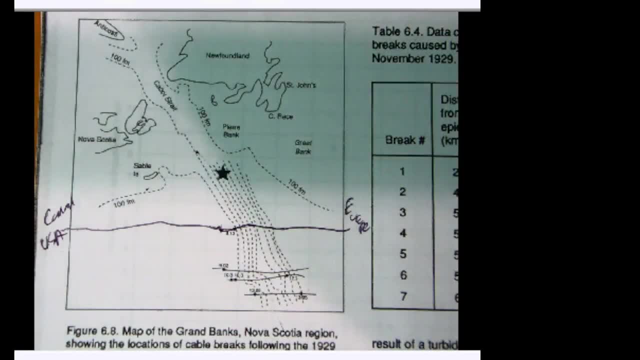 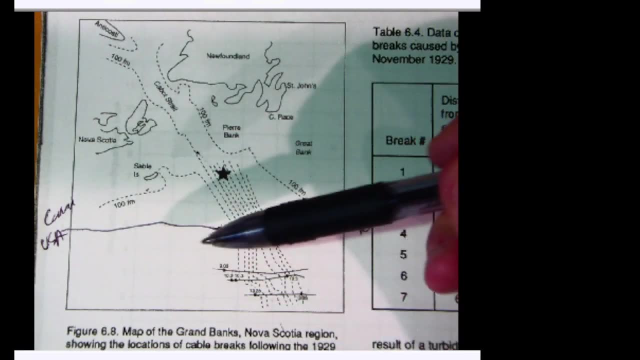 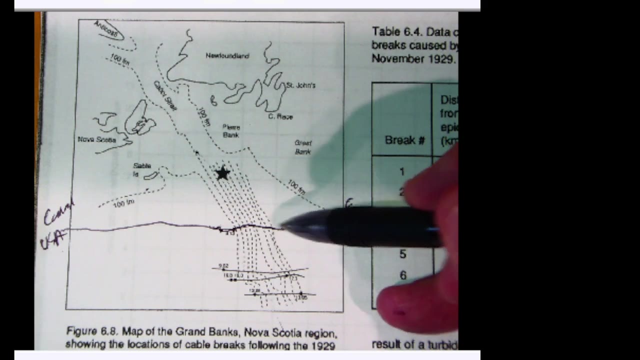 morse code: dot, dot, dot, dash, dash, dash kind of kind of thing. right, and so these were all. these were lines that were laid down by ships on the seafloor, and so here you have this canyon, and the lines are going across the canyon and they're dipping into it in some places, and 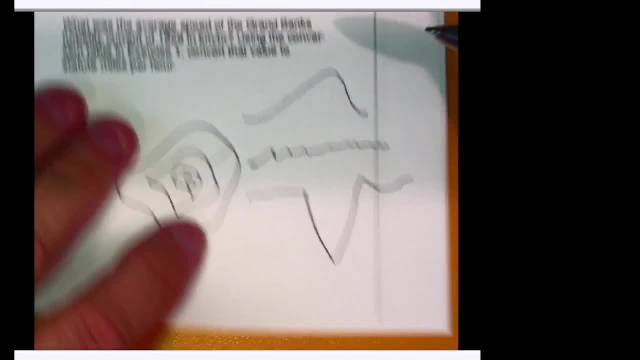 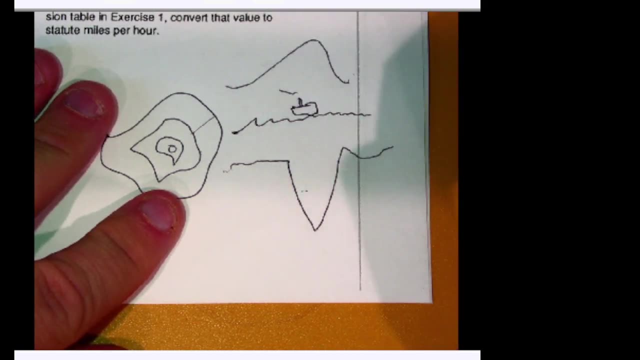 everything else right. so let's just go back to that profile pic. here's the canyon, there's a. here's a little cartoon boat. here's a little cartoon boat. okay, very bad drawing and and they were laying down these, these lines, these telegraph lines, and so you get them like this, and maybe sometimes they droop into the canyon or whatever. 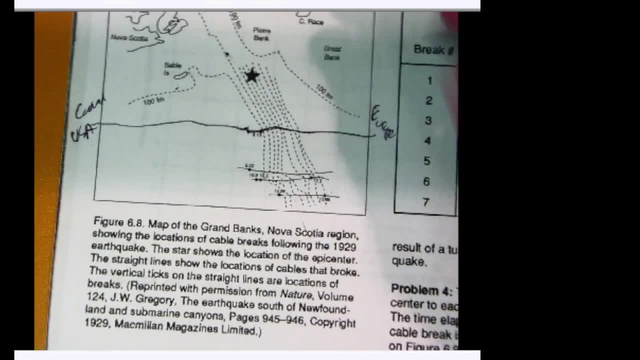 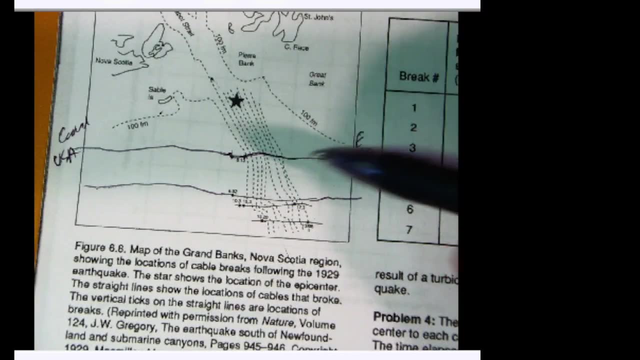 okay, so this was, this was the setup. you had all these lines and cables going across we. so I'm saying this is telegraph lines. we have these today. right, we still have them today for internet communication and other kinds of telecommunication lines. they're actually still out there that we've laid many new ones since then, but so these were really. 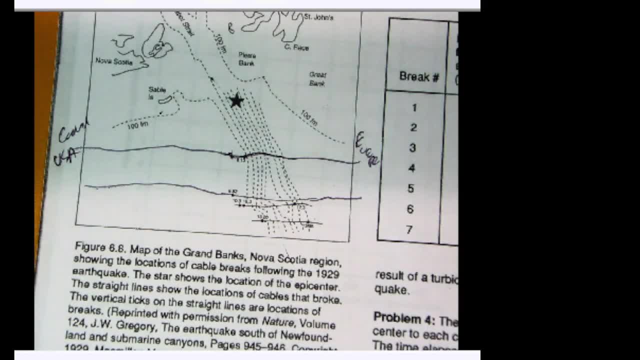 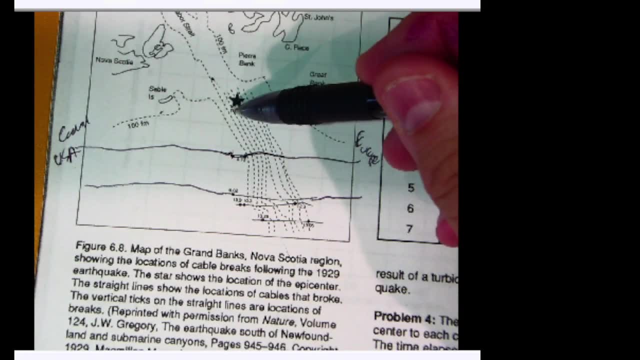 important. this is how people in the US and Europe and other parts of the world, how we could have like global communications back in 1929. so in 1929 there was an earthquake. the earthquake was centered here. that shaking caused a collapse of the marine sediments and it caused this. 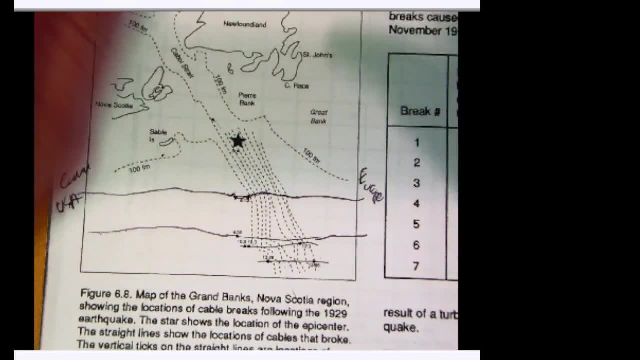 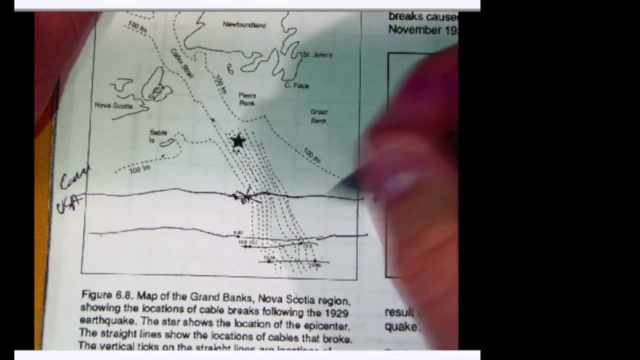 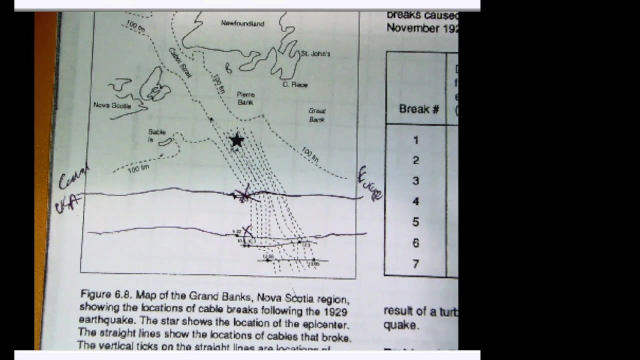 turbidite flow or avalanche, and the avalanche ran down the canyon and it started snapping these lines. it started, it started breaking them apart, as that you know flow of mud and sediments and boulders or whatever was in there, crashed into them. it ripped them apart and so the 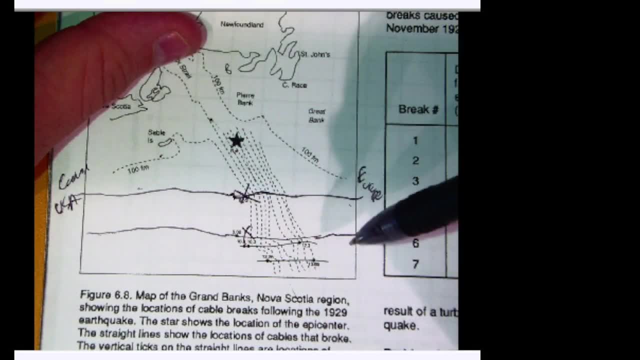 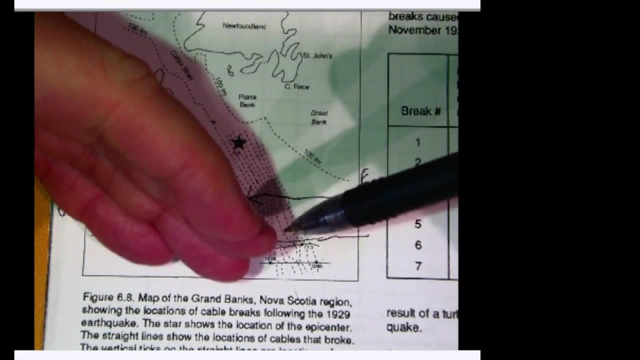 communications that were going on between these across the ocean. they got shut down and we knew. so that was bad and people realized: oh, there's all this stuff going on down here, right, there's, there's all this movement of material, these submarine avalanches that are happening. 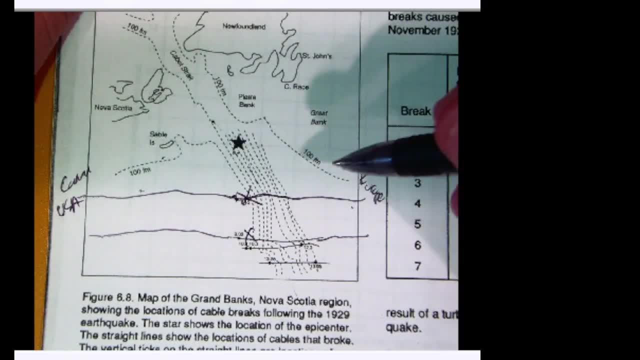 we know about it because they interrupted our communication. and we know about it because they interrupted our communications. we had to go out and relay these lines, and it took time to even figure out what actually happened. right so they were able to detect the earthquake, and then they. 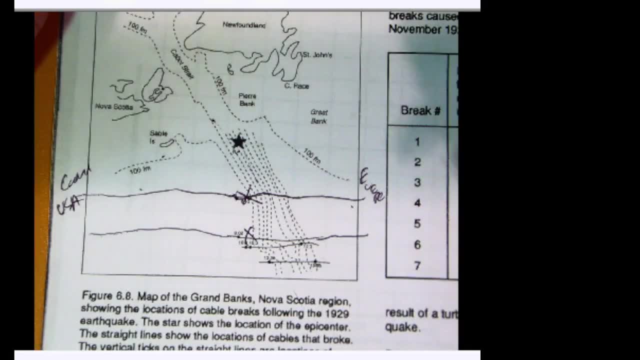 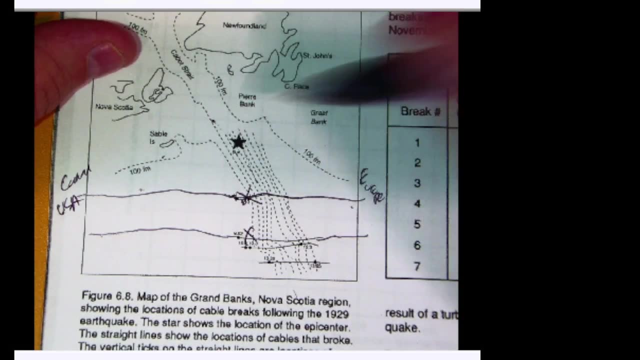 were able to realize that. you know, their communications got cut off. it took time to figure out what the connection there was, what actually happened? right, because there's lots of things going on in the world at any moment. so this and now as these, so when the the real story. 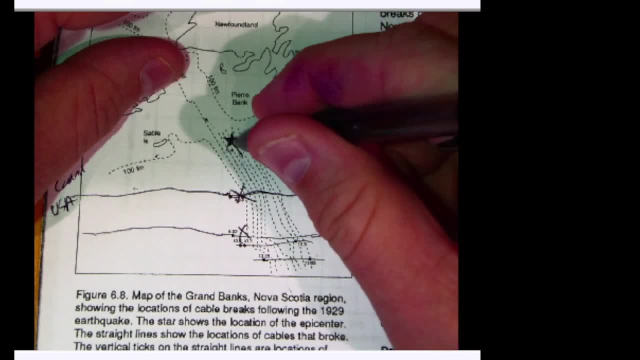 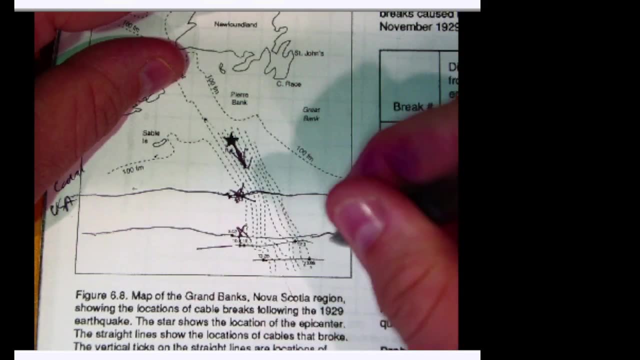 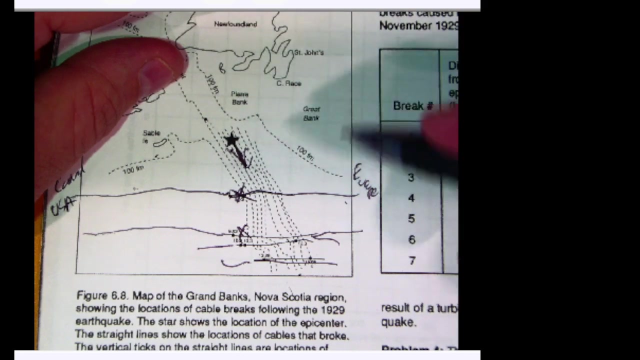 is that, as these um as after the earthquake happened, the turbidite flow, the avalanche, flowed down the canyon and so it hits this cable first right, and then this one second, and then this one third and fourth and everything right. so it hits them in sequence. we know exactly when they were hit, because we know the time that we lose communication. 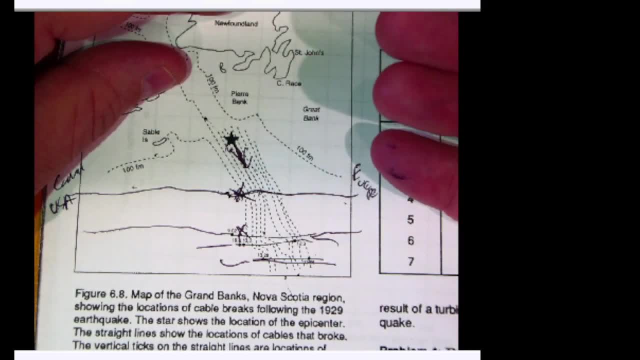 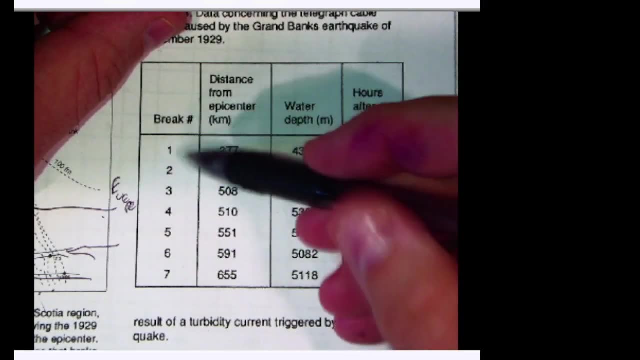 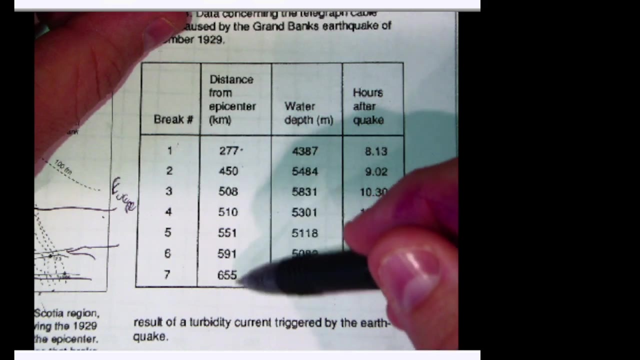 and we know where these cables are because we laid them down. so we know exactly how far apart the cables are. so if you look here, this is just showing you the cables that were broken, how far each cable was from the source of the earthquake, from its epicenter, how deep in the ocean it was. this is, these are deep. 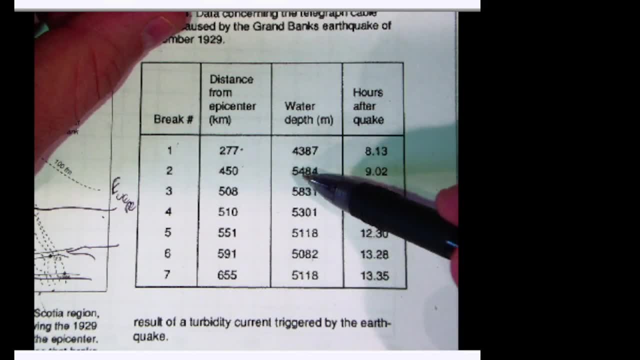 water. that's five kilometers, 5.4 kilometers right, 4 000 meters deep in the ocean, and how long after the earthquake started that the cables were snapped. so we have seismogram stations that tell us when the earthquake started. that's like time zero, eight hours after the earthquake starts. 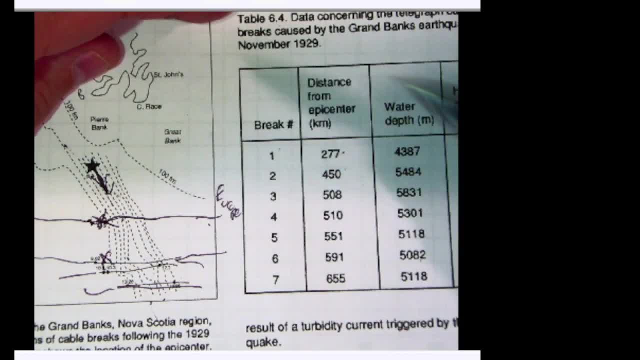 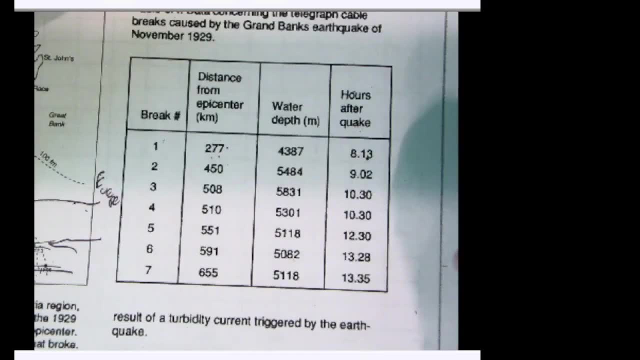 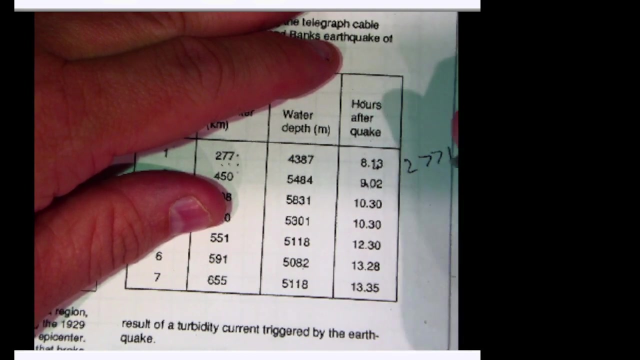 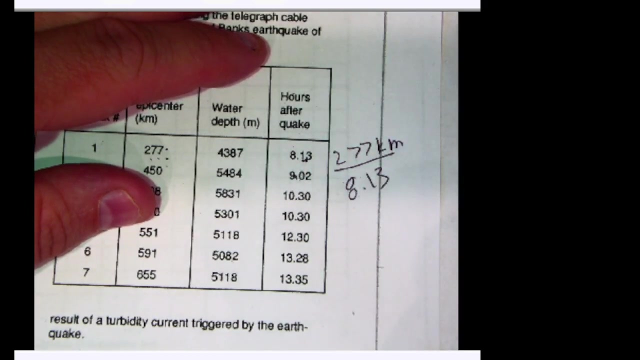 this first cable gets snapped. it's 277 meters from the site of the earthquake. so it this flow was able to travel 277 meters in eight hours. uh sorry, um kilometers in eight hours, so 270. so we can tell, we can get a speed from that kilometers and hours. right, there's a distance from the site of the earthquake to the. 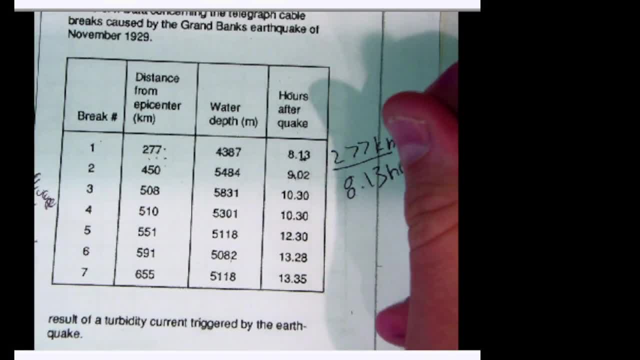 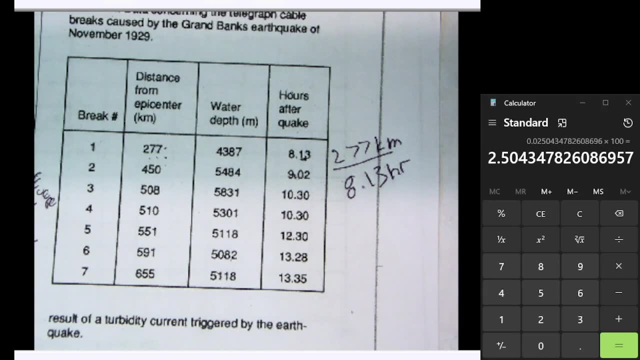 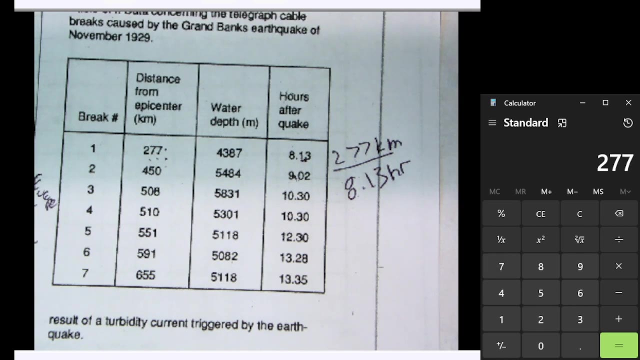 source and distance and and the time. if we have distance in time, we know how fast someone was going. so i'll just quickly put this back up. all right, and so if you had, if you were going, 277 meters kilometers in 8.13 hours, that means you were traveling 34 um kilometers an hour. 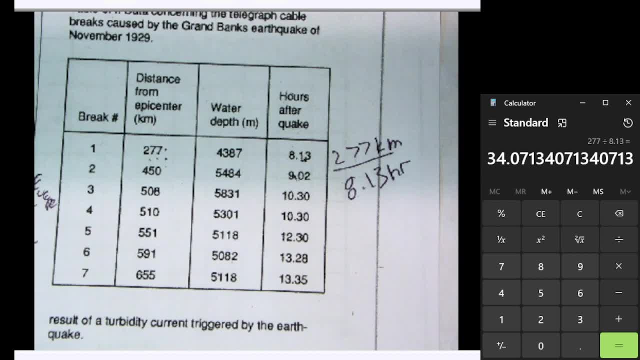 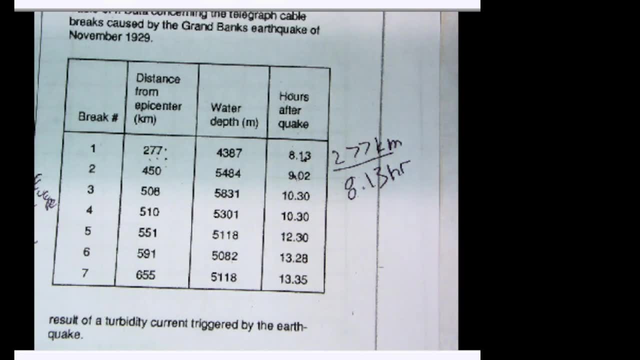 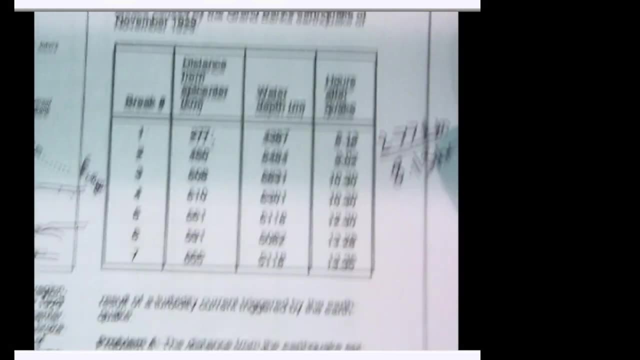 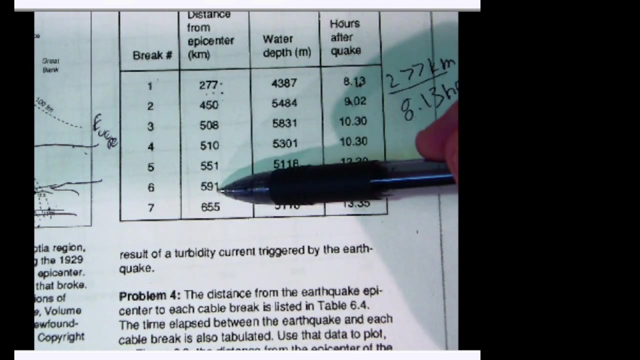 and so we can look at this. this flow crossed the canyon, and so you're asked to find the average speed at which it it flowed down the canyon, and so the way to get the average, the best way to get the average, is to take the total distance and divide it by the. 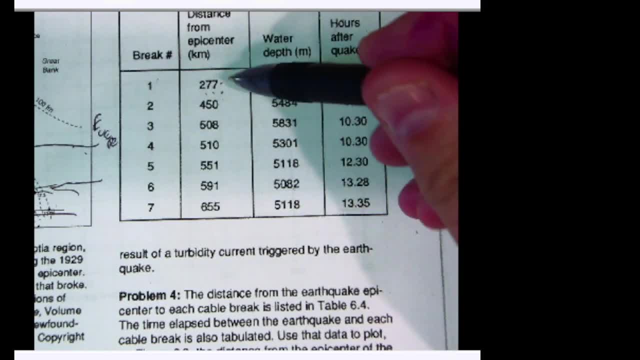 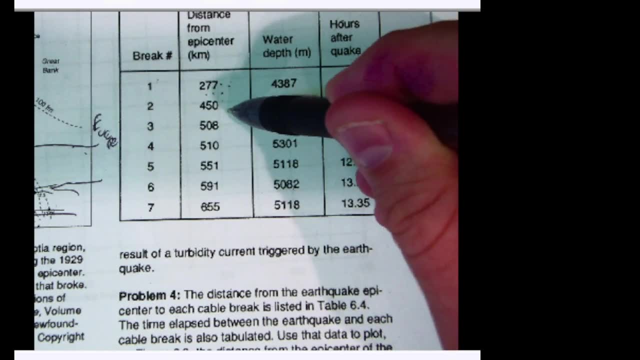 total amount of time. so this is kind of like if you're in a car and you go from your house to location one and and then you go to another place and you're going to a whole bunch of different places. when you're driving between place, you 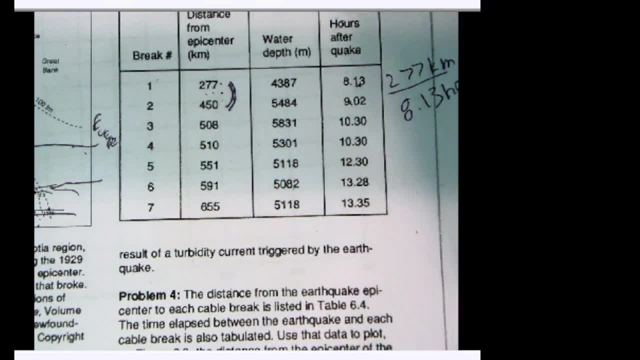 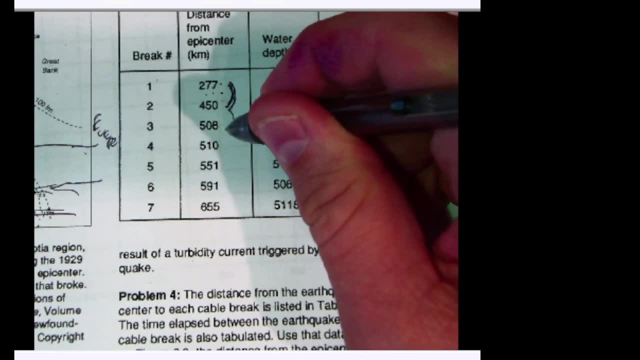 know location, the grocery store and the. you know CVS. right, you might be going one speed and then if you go to your friend's house, maybe you can get on the highway, so you go a different speed, so you would have different speeds during all of this, right, but if we wanted to know your average. 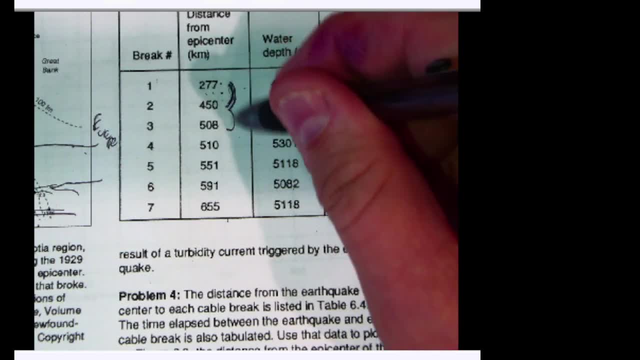 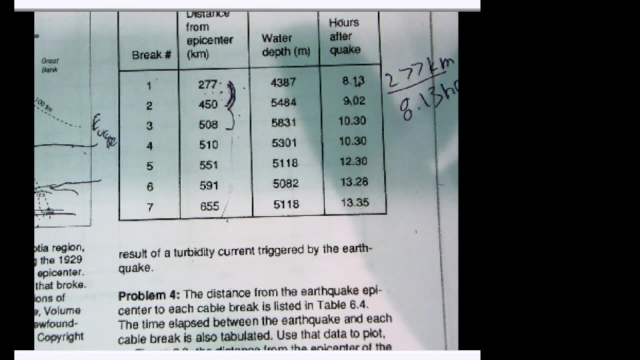 speed during this time. we would find the total time, total distance and divide it by the total time. so maybe you drove with many stops, a hundred miles, and you did the whole thing in one hour. your average speed was a hundred miles an hour. right, maybe one part was faster, other parts were slower, right, so you can. 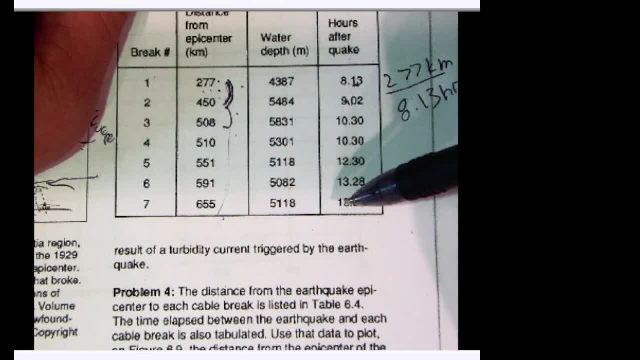 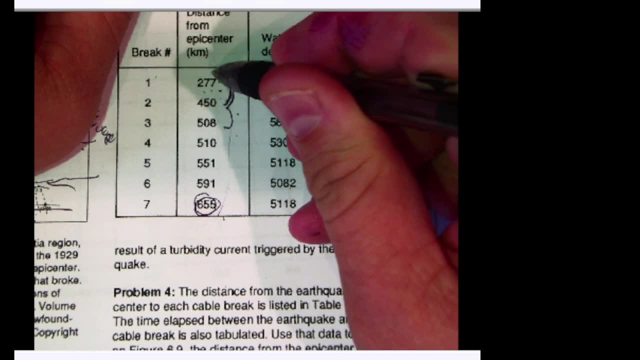 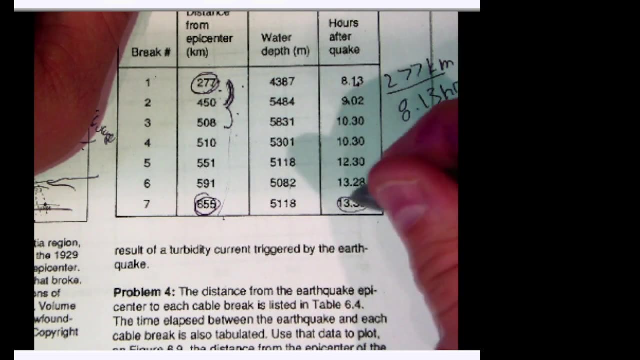 calculate the total distance and the total time and you can get the average speed. so you would take this distance, subtract this distance from it. now I'll give you a change in distance and then you would take this time and subtract that time from it. that would give you the change in time. so you know, you don't, you don't. 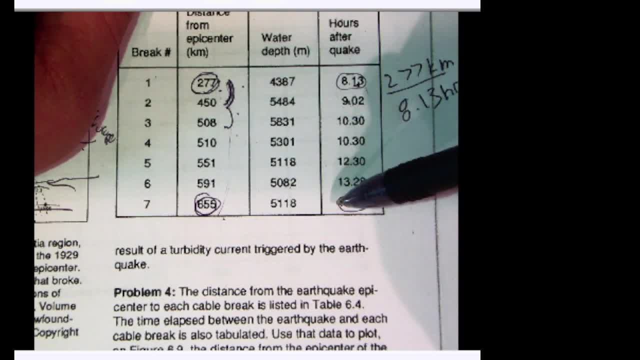 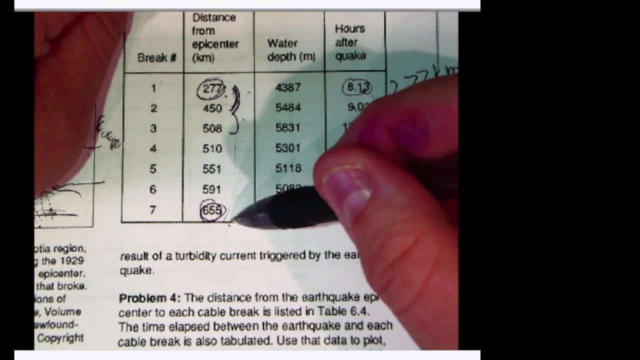 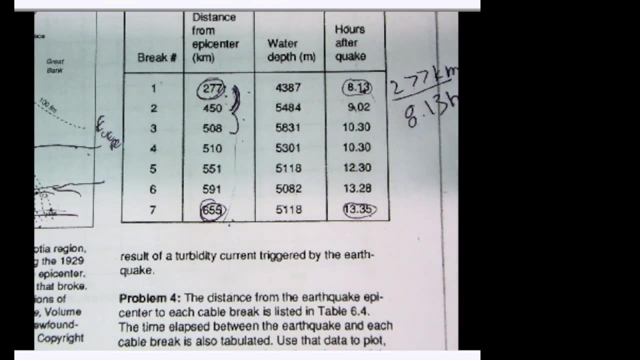 necessarily add up all of these times, or something like that. if that, if that's not clear, you want to find the change from point one to point seven and the change in time between point one and point seven, and so once you've done that, then you've calculated the, the average speed of it. okay, so that's, that's what. 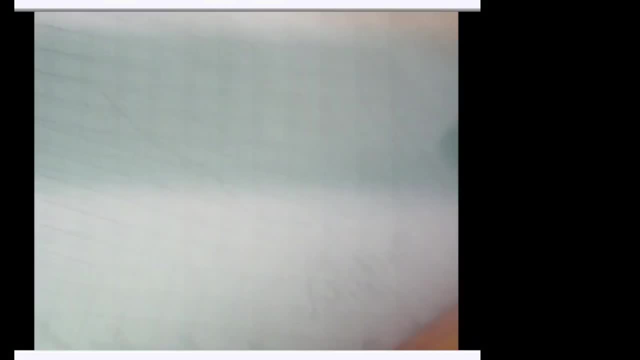 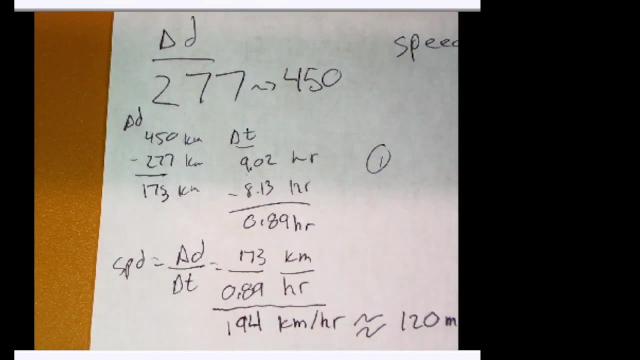 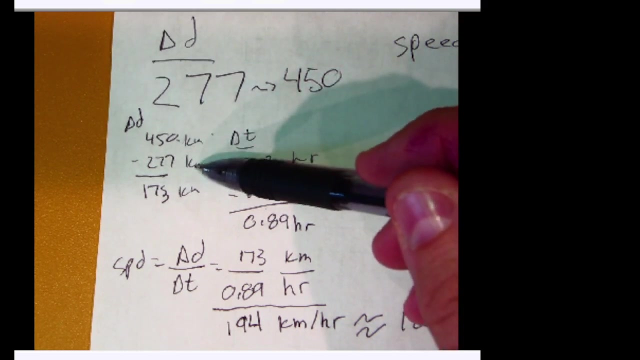 we're looking for in that one also. oh, I kind of worked through something, right, so so, for example, these are the kinds of answers you're you're kind of looking for, right. so here we go, from 450, the, the cable break. at 450 kilometers, the cable. 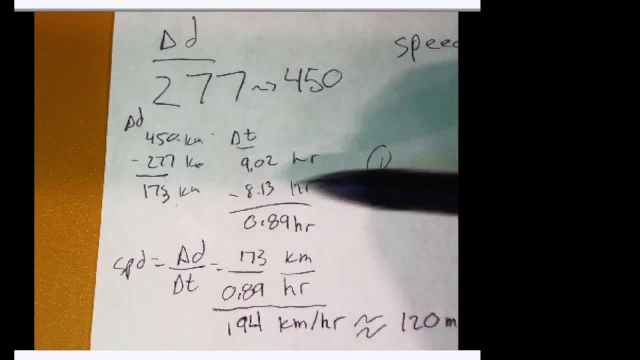 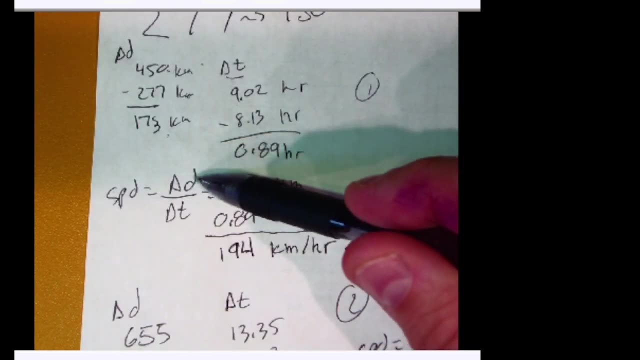 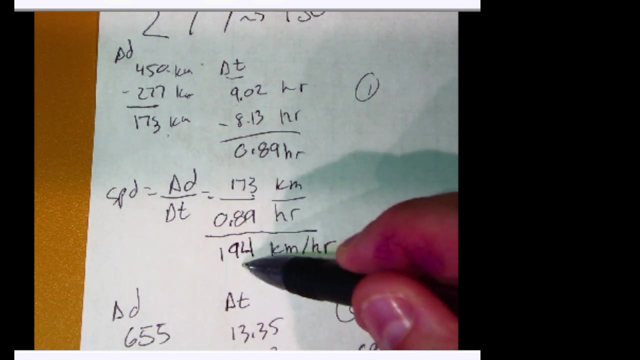 break at 277.. the difference is 173. the difference in time between those two things was 0.89. the speed is change in distance divided by change in time. so this was the change in distance, this was the change in time. you get a speed of 194 kilometers an hour. so this one was very, very. 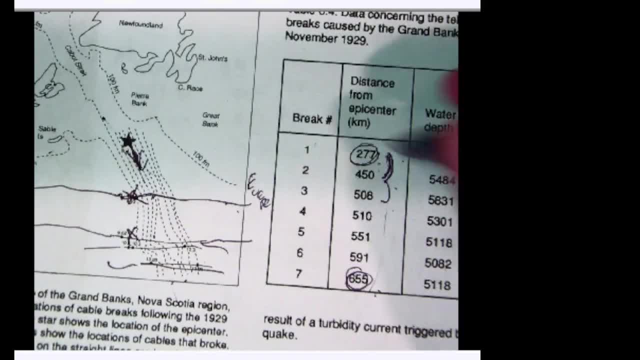 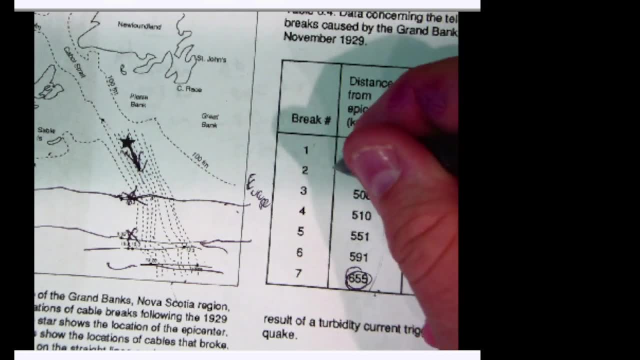 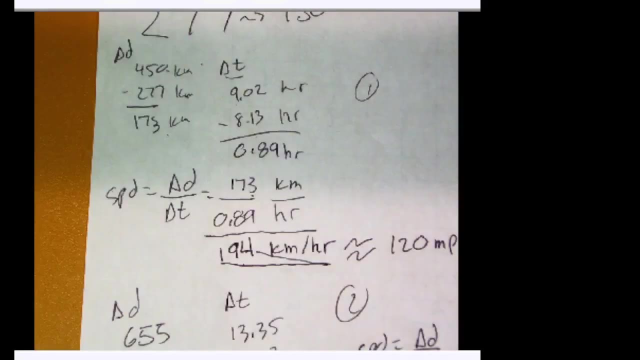 fast, right, and so that was going from the 277 to the 450.. okay, so it's going almost 200 kilometers an hour when it, when it travels from from this line to that line, it's going very fast. and so this is. you can use this for calculating the the. 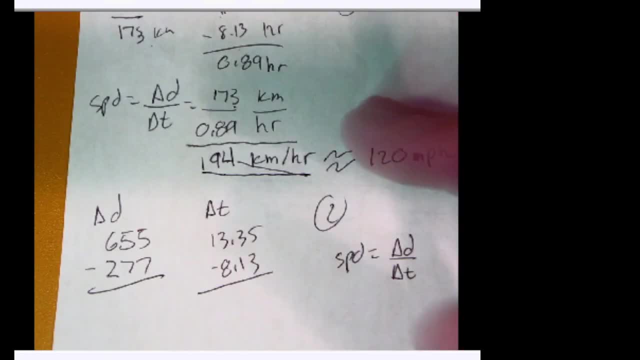 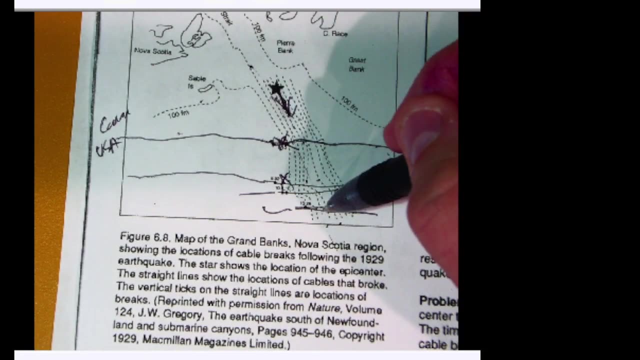 total average. okay, you're gonna see that it's slower overall. the first part is much faster. the later stages kind of make sense. right, you're running downhill, you're running down a canyon, you lose speed over time, and so we're trying to calculate the average speed of the whole collapse. 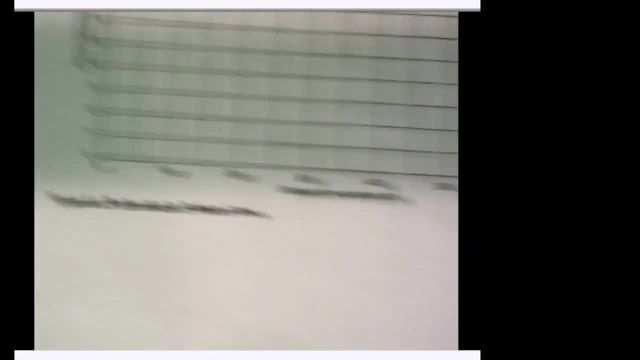 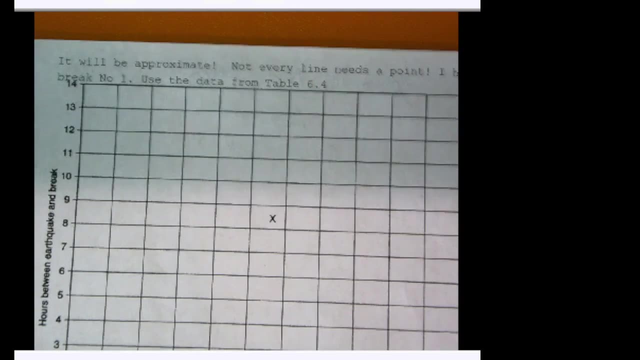 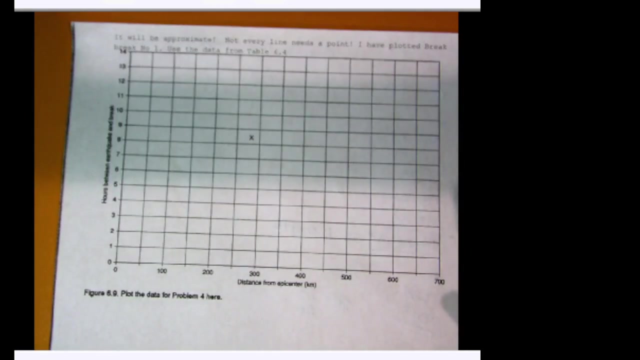 yeah, so you can do that. oh, and then there's this other part right now. this part shows you how to is asking you to make a graph. so look at the. let's look at the whole thing first. so it's really just a piece of graph paper and on the, 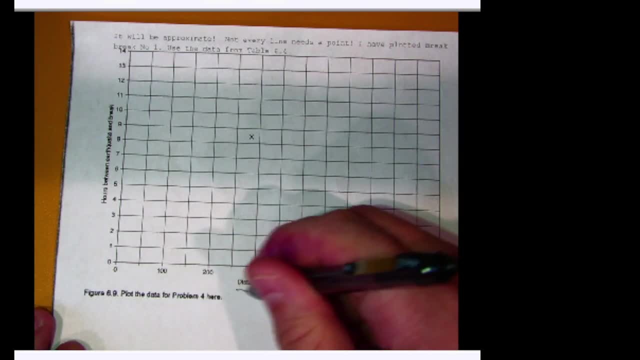 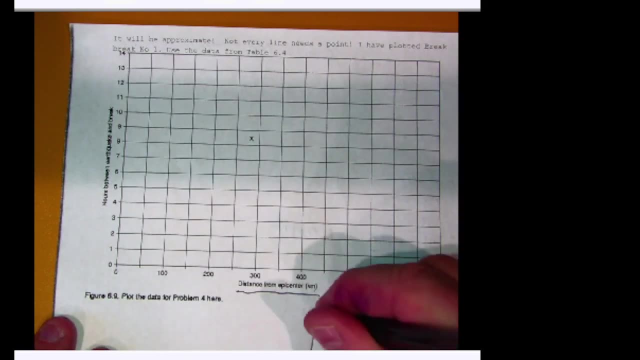 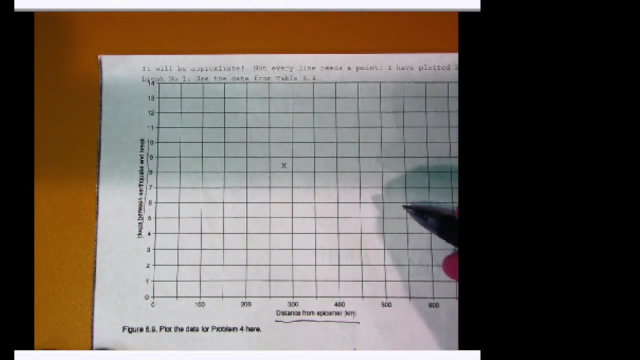 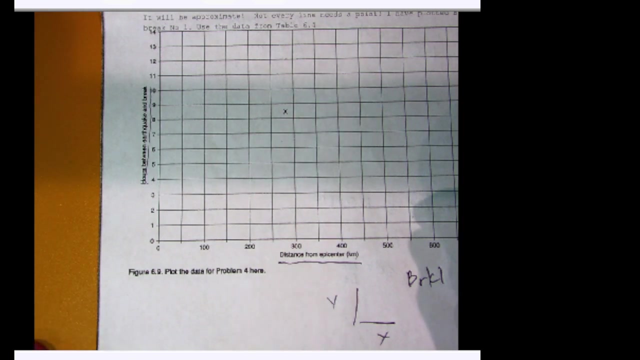 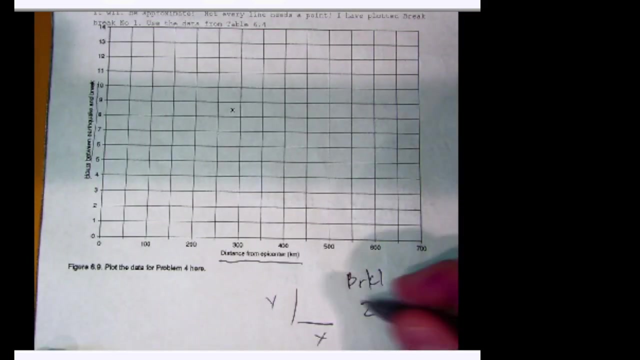 bottom. it has distance from the epicenter in kilometers. right, that's what the KN is, and then that's the x-axis, and then the y-axis is a between earthquake and breaks. so break one. what was its data? it happens at 277 kilometers distance. okay, that's its X value and its Y value was eight point. 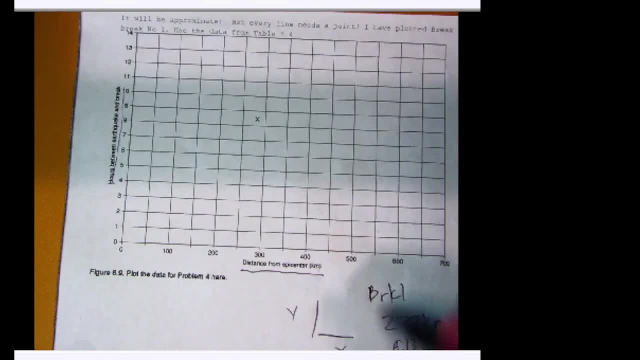 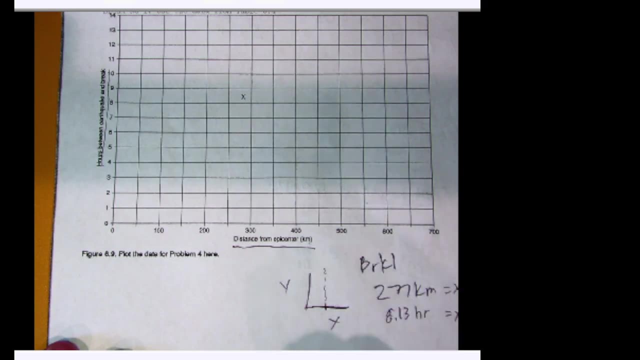 one, three hours. so when you make it a graph, you take the X value, find out where it is. you kind of draw a line all the way up, and then you look for the walk corresponding Y value, find out where it is. you got it. you can draw this. 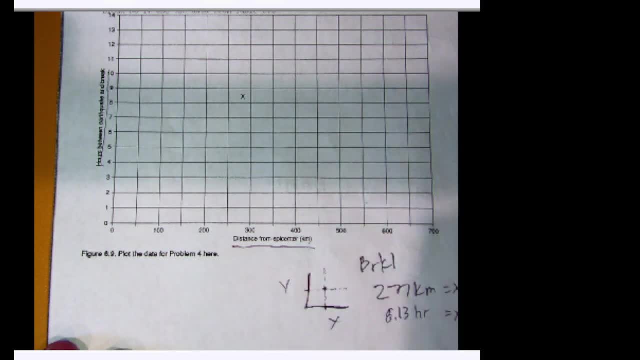 imaginary line across, and where they intersect is where you put your points, and so that was done here for point one, for the first break, right? so it's about 270 here. here's the X value, and then you look for the Y value and then you look. 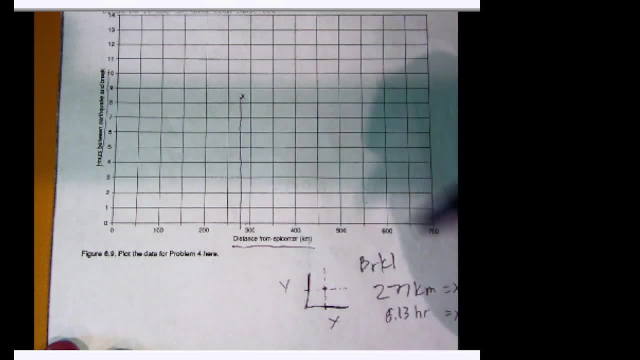 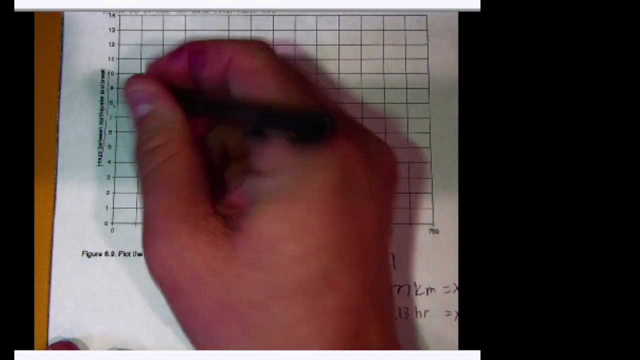 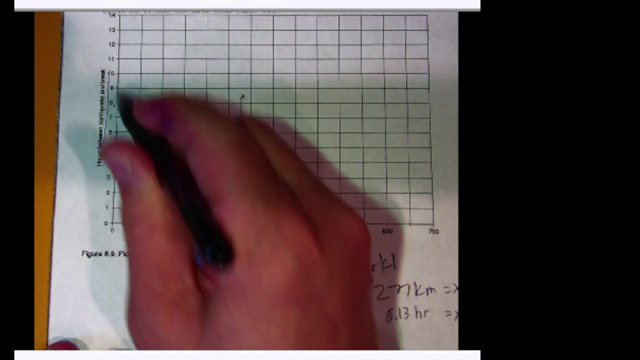 for it it's about 277 for the X value, and it's here's eight, and so it's a tiny bit. and here's nine, right. so across one cube is a value of one. so eight point one three is really close. these are just estimates and they kind of correspond to. 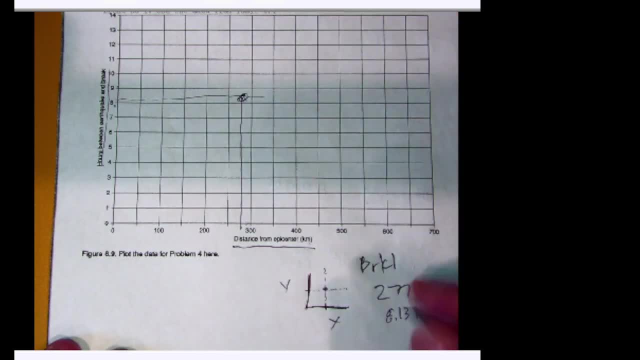 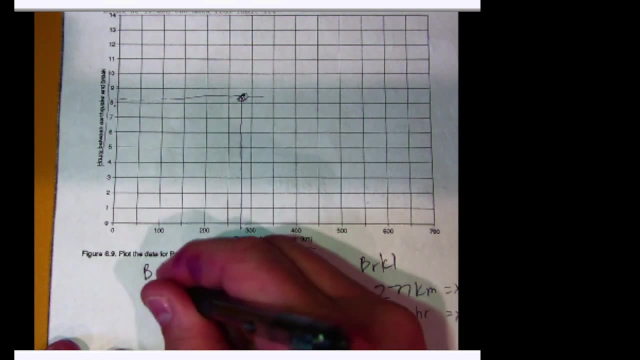 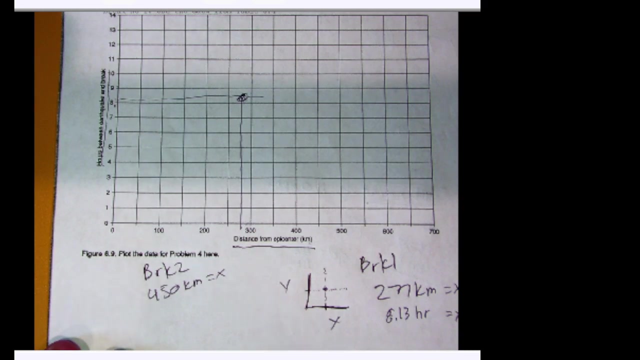 this point here, which is marked with an X, the next spot would be break two. okay, so break two broke at 450 kilometers distance. that's the X value, and it took nine-point-o2 hours for that to happen. that's the Y value. so 450. 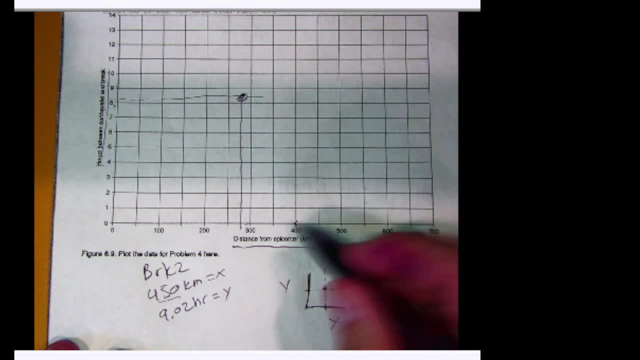 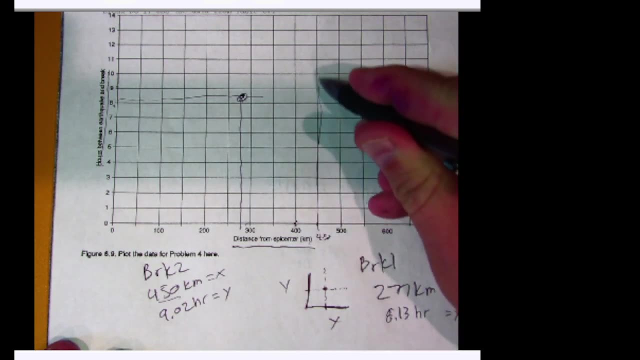 here's 400, here's- it's really hard to see, but you can see it on your copy- and here's 500, so this must be 450. so we're gonna go up this line somewhere, and over here is the line it was right here. here's 250, minutesوا garden. so an extra, that's about 750. 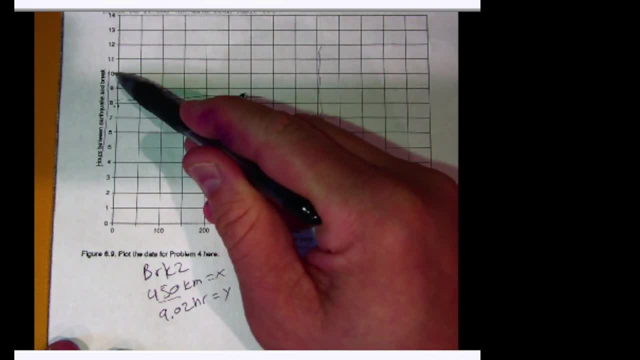 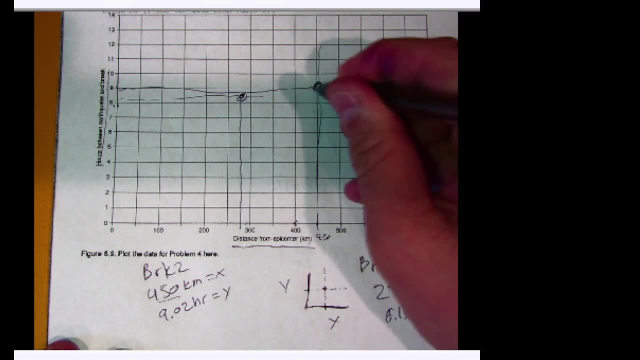 Here we have 8,, 9,, 10,. right, We're at 9.02 is what we want, so I'll just follow this line across. okay, And so break number two happens at this intersection, And then you can do that for all seven breaks. 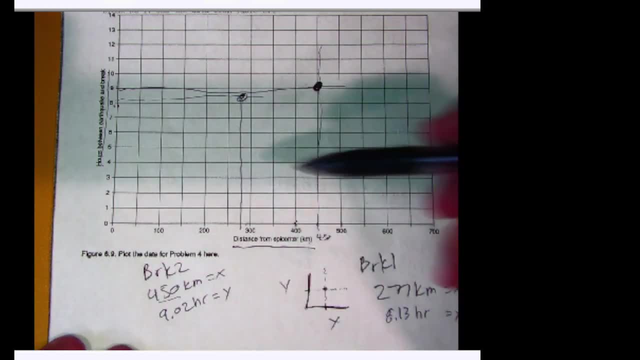 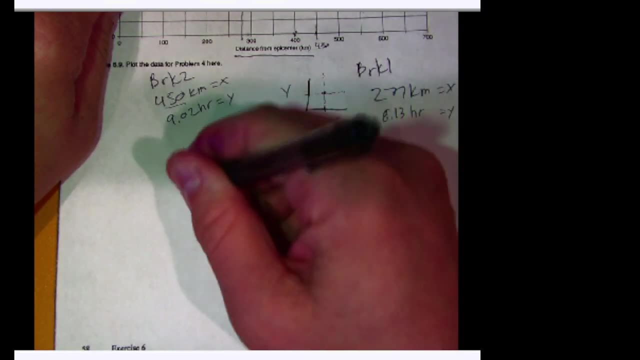 You're gonna have seven points here, right, And what they're gonna do is, visually, what they're showing you is distance and time, And I don't know what the chart's gonna look like, but pretend it's something like this: 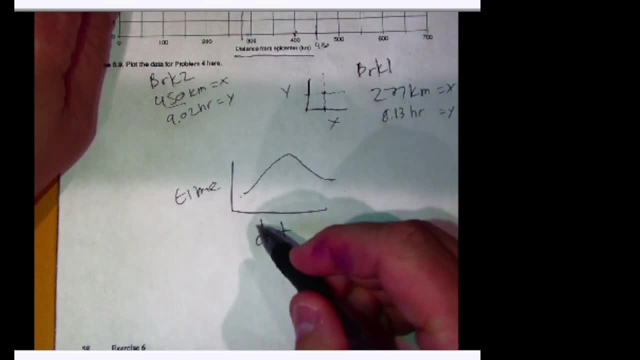 If you know that this is not Tim but time, If you know this is distance and time, you can tell that whatever was going on here, whether it was a car or whatever this object, was it sped up and then slowed down, right? 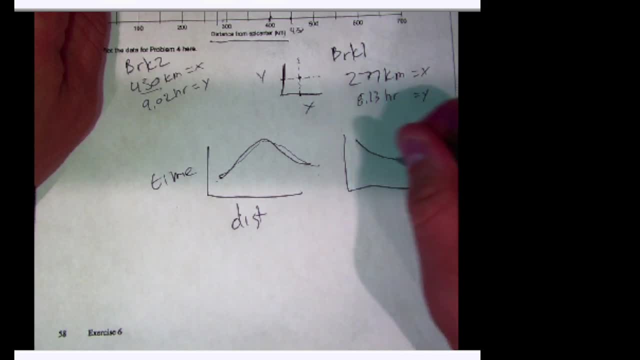 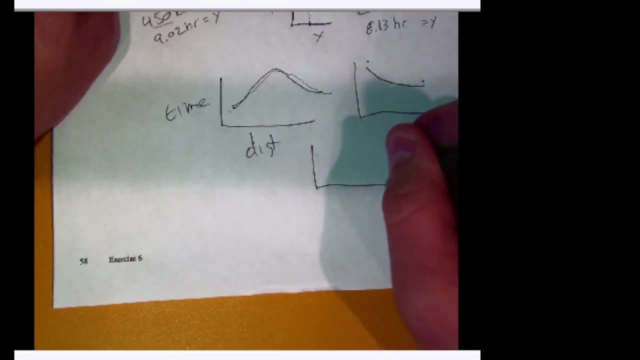 And so we might expect the chart to look something like this in a lot of instances, right where something has a high speed and it goes down to a slower speed, Or maybe it eventually what we expect for most things actually is that they'll have whatever their speed is. 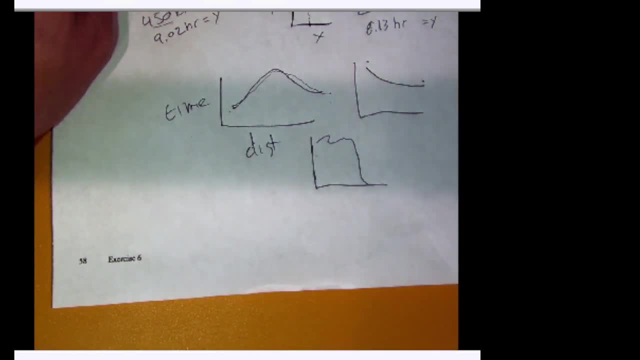 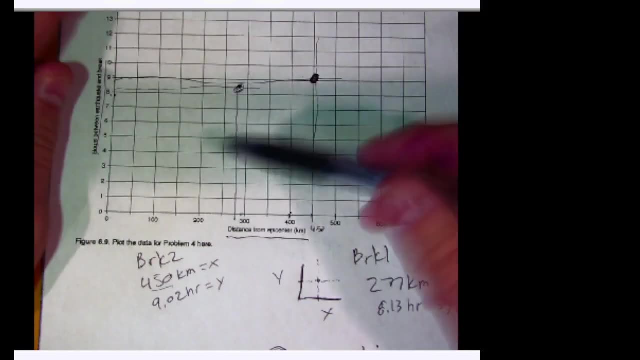 and they might go down to zero, right, Which means that they've come to a stop. So you can look. why do we do this right? Why do we bother going through this table and charting it like this? It will tell us about the changes in speed of that submarine avalanche. 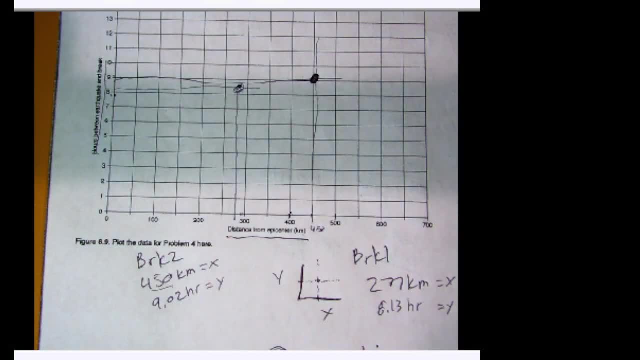 And so people didn't know about these things really at first, and it really started to convince people that they were powerful. there was a lot of energy involved, that they could move very quickly and that they could change the seafloor right. 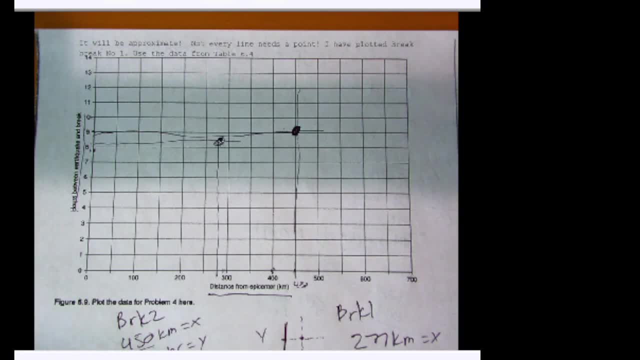 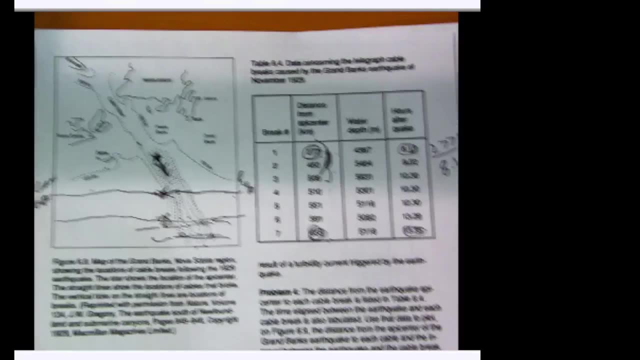 The seafloor. even These sediments don't just snap cables, they can scour out the bottom of those canyons and valleys and make them deeper. So these are all different And, like I said, this is kind of a famous example. 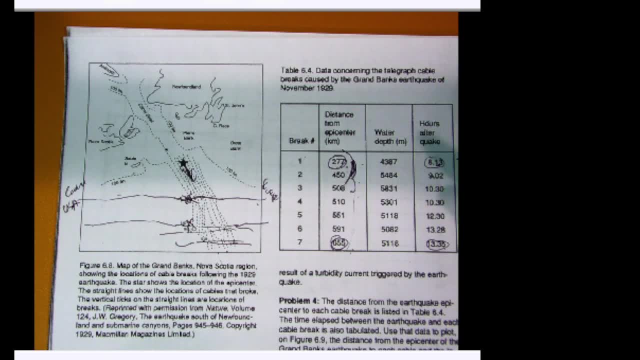 These breaks along the Grand Banks Canyon off of Nova Scotia. It's when people first started to realize that this was happening. So only 1929, right less you know about 100 years ago, which isn't that long ago. 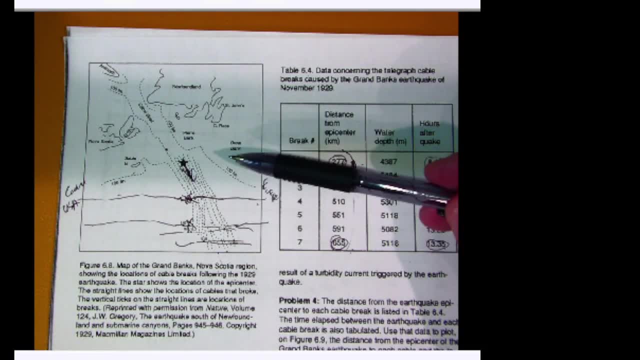 And so they, we were able to understand what's happening with these sediments on the seafloor. The seafloor is not some inactive, you know flat place where there's just you know mud on the bottom and that's it right. 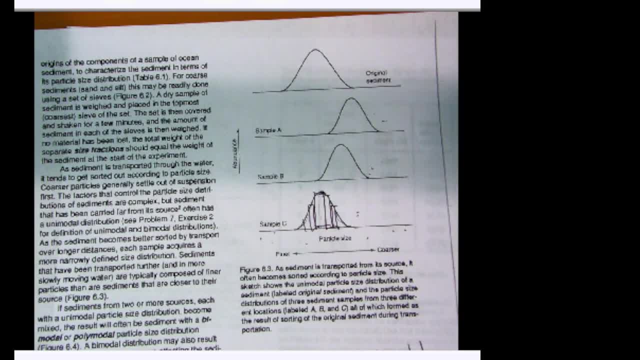 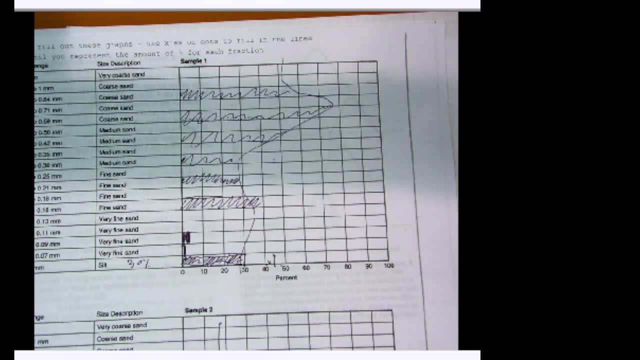 There's different kinds of sands. there's coarse materials, there's finer materials. Different locations have different distributions of those different sediment sizes. So some places have a lot of fine sand, some places have a lot of coarse stuff. Sometimes we find anomalously large boulders and cobbles there. 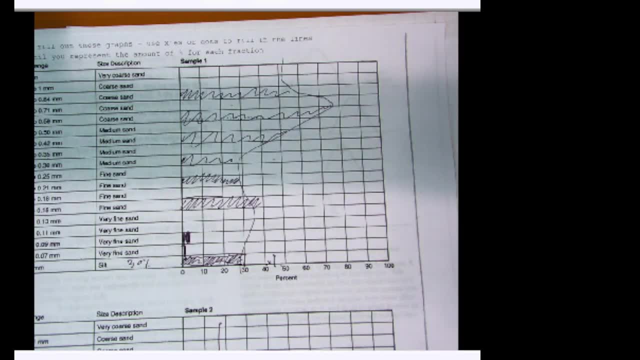 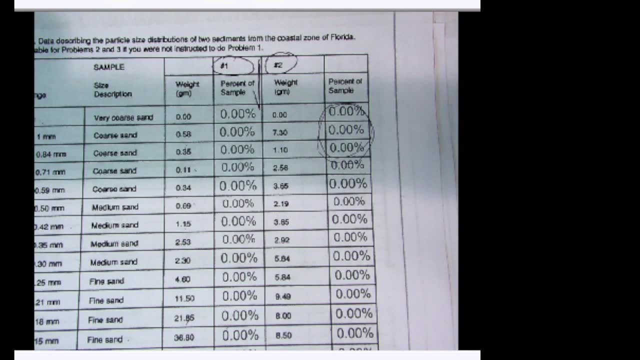 We have to try to explain them. They're, We think they're linked to, like the growth and retraction of ice sheets. We calculate that data in terms of these tables to share it with each other and try to understand what's happening. 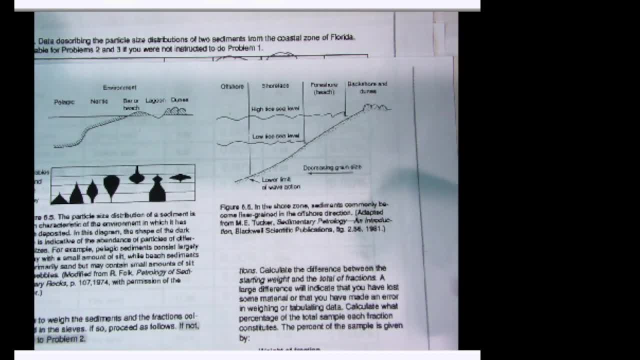 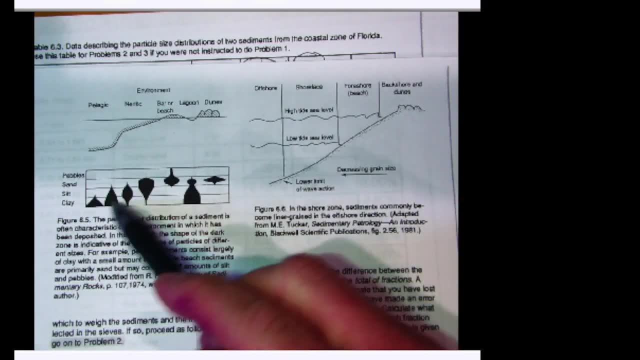 And then you know, in the introduction it talks more about the setting in which you apply these things right. So we have different beach profiles. You can tell very quickly from here now that you know this place has a lot of clay and very little of anything else, right? 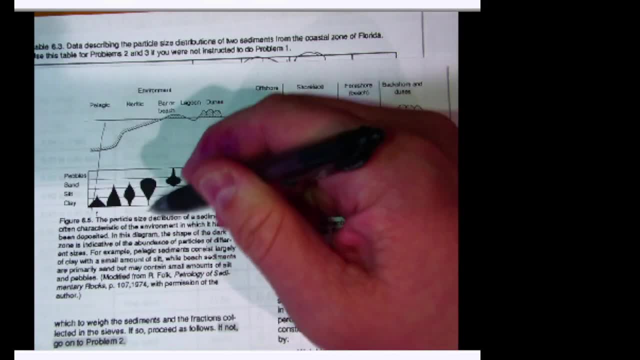 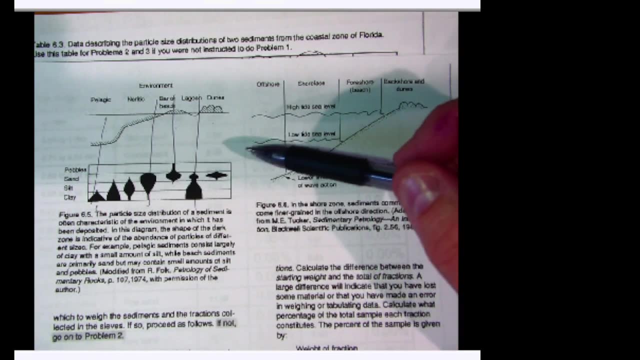 So it tells us about all these different And it corresponds to these different places along the beach, Right From where we are to where it gets very deep and there's lots of boats out there. So this is how we're able to understand what's happening with these different marine sediments. 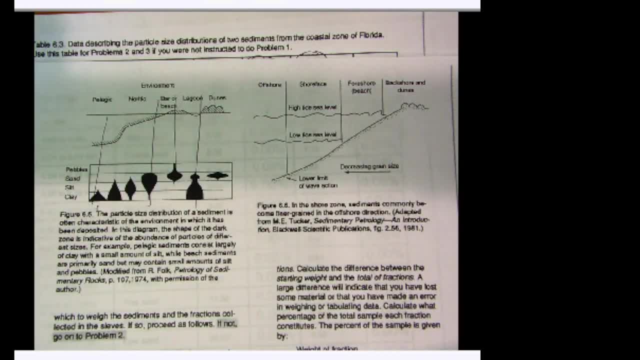 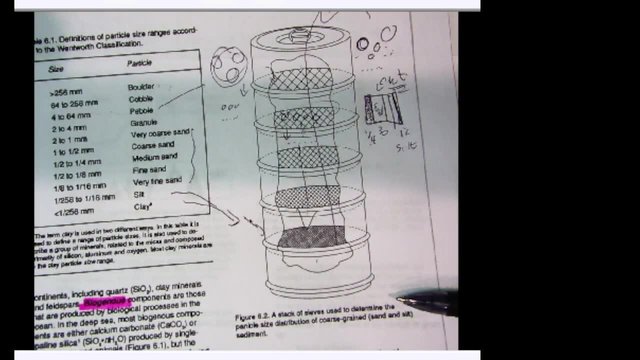 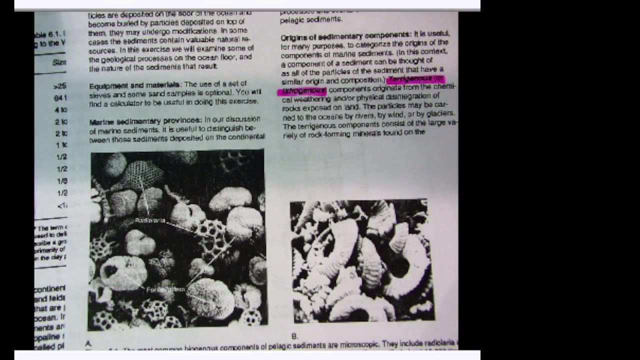 Okay, so you guys give that a try. I've extended the date for the upload. This all works because we have these nice little stacks of sieves. Try to answer that and give it and hand it in. Oh yeah, and these pictures here. what's going on here? these are some examples of the sediments. 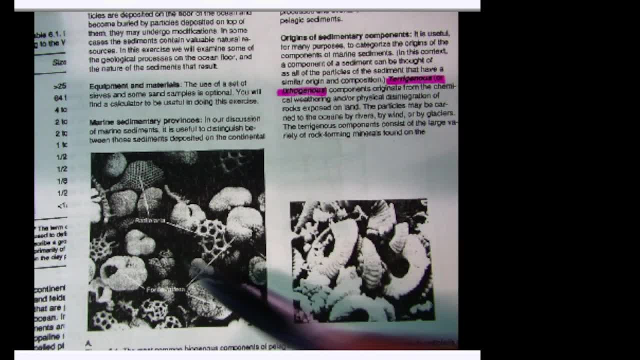 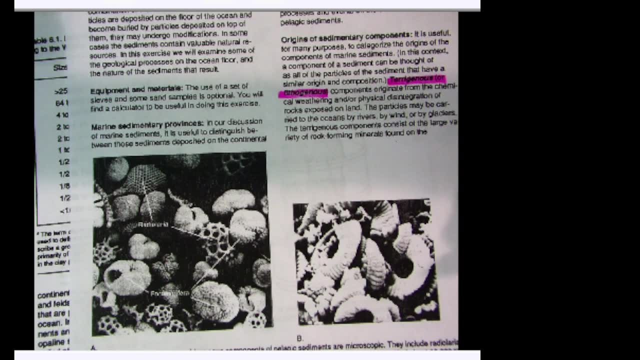 So they're not just, you know, spheres of certain sizes, right? These are like the shells and remains of different plankton and different marine organisms, So sometimes they make up the sediment entirely, right? So it's just, again, one way in which we try to understand these sediments which tell us about processes in the ocean. 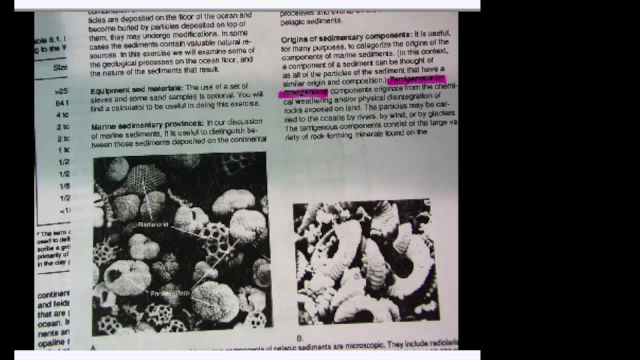 So give that a try, upload that, and then we'll see how that goes, Okay. 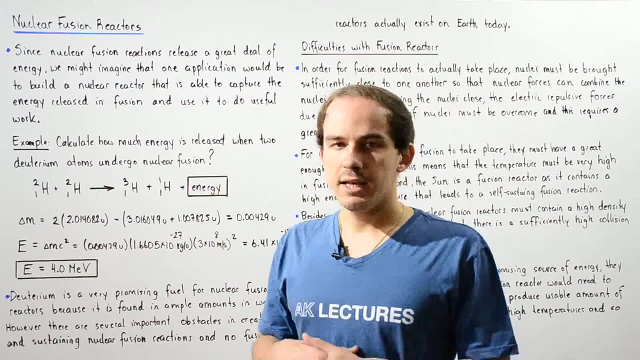 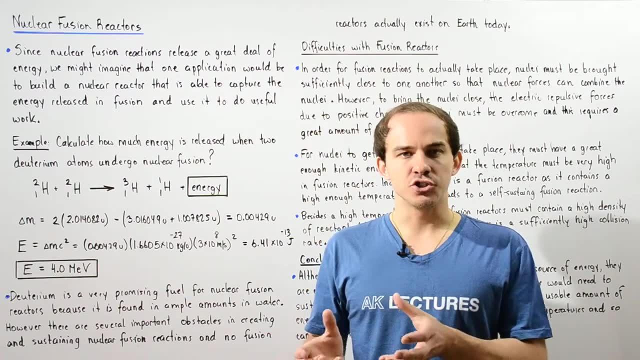 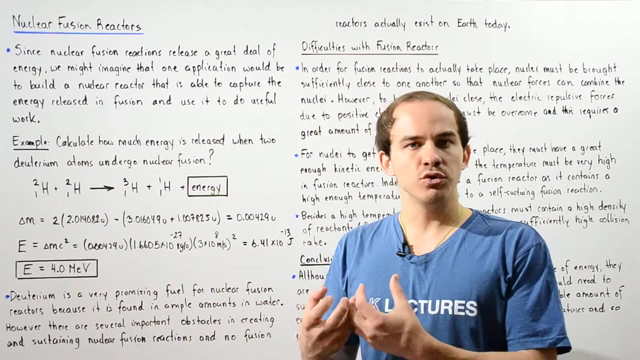 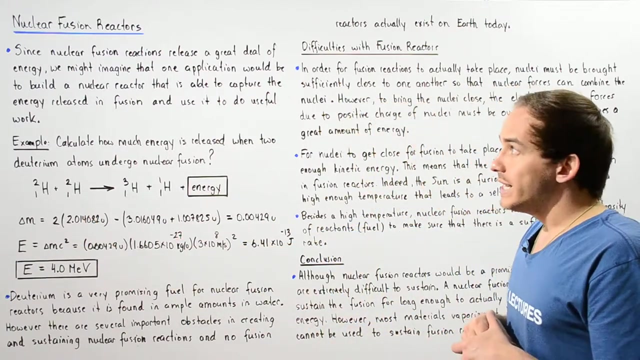 In our discussion on nuclear fusion reactions, we said that these types of reactions release a great amount of energy. So basically, we take two nuclei, combine the nuclei to form a more stable nuclei and that releases a certain amount of energy. Now, since nuclear fusion reactions 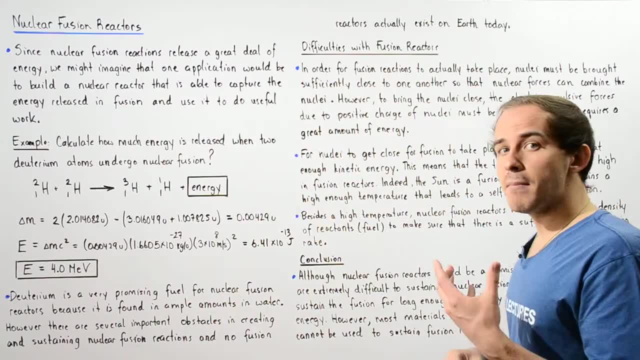 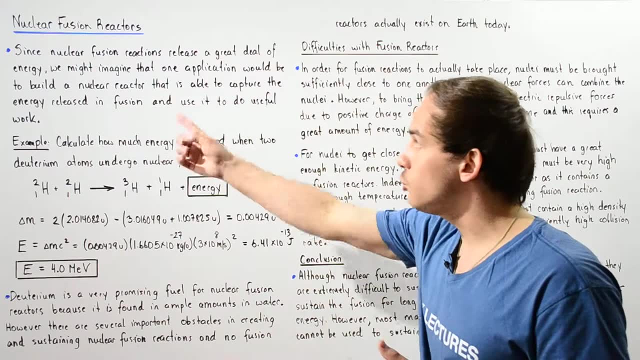 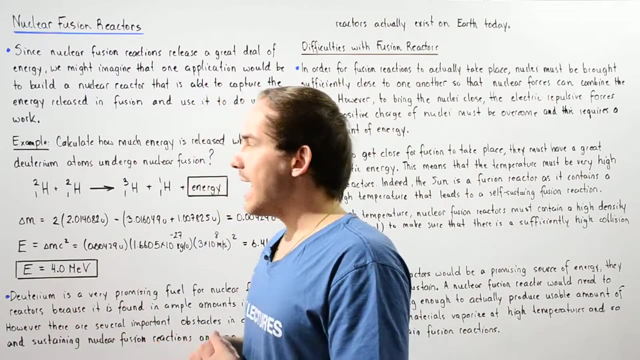 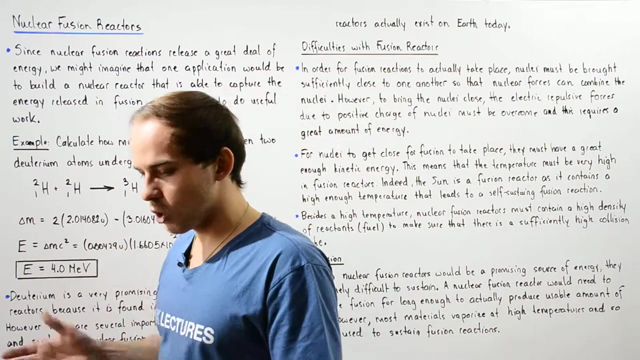 release a great amount of energy. we might imagine that one application of nuclear fusion reactions would be to build a nuclear reactor that is able to capture some of this energy that is released in any nuclear fusion reactions and we can somehow use this energy to do useful work.